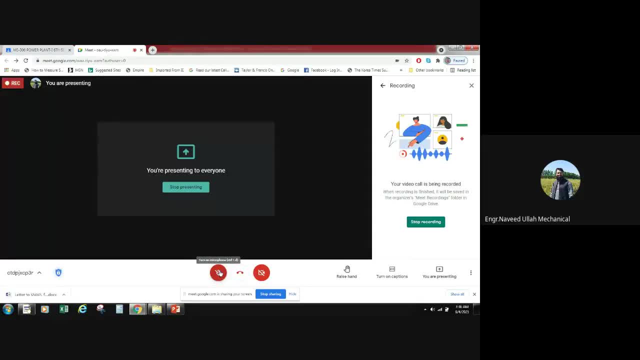 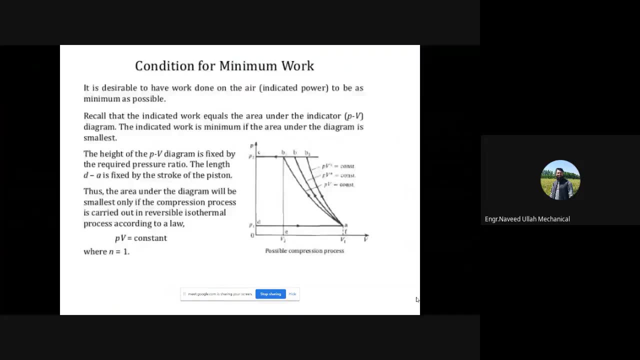 Okay, so today we will be discussing about the remaining portion, the that we left in the previous class. So if I just refresh what we have studied in our previous class, you know, we discussed about generally the working principle of positive displacement machine, okay, and particularly about the reciprocating air compressor, okay, and then we showed, you know, the diagram or the cycle upon which the reciprocating air compressor works, okay. And obviously we discussed about what is indicated work, R power, okay, and how to calculate that. So and also some examples. So that was actually because . 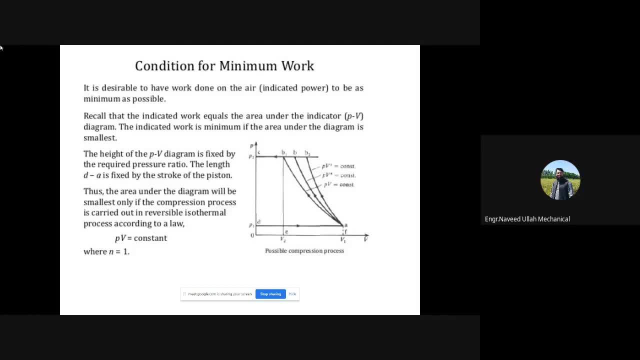 Okay. That was actually the one of the analysis objectives. So if you remember in the previous class, there was a slide where we talked about the analysis objectives, that what are the analysis objectives that you are analyzing the reciprocating air compressor. So we need to know about the pressure and temperature before compression process and then temperature and pressure. Okay. Okay. after the compression process and then we talked about how to calculate the indicated work our power and then after that we talked about the frd that is the free air delivery etc okay and obviously the important thing for any mechanical installation or machine that is the efficiency okay so mechanical efficiency okay then after that if you remember i told you that it's for is reciprocating here compressor is concerned we need to talk about three four things okay uh one of them is or it was basically that we discussed in the previous class uh is um uh reciprocating air compressor without clearance volume okay and um then we left with 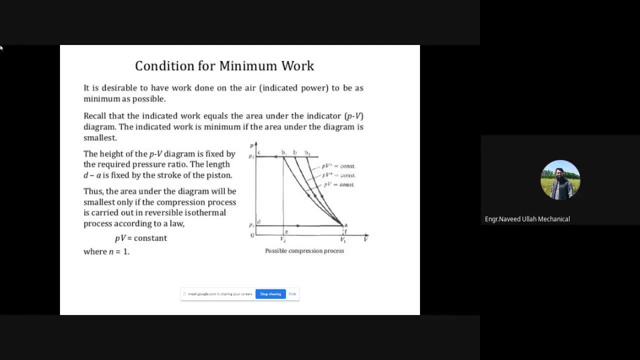 uh this relocating air compressor with clearance volume and i also told you that we will be 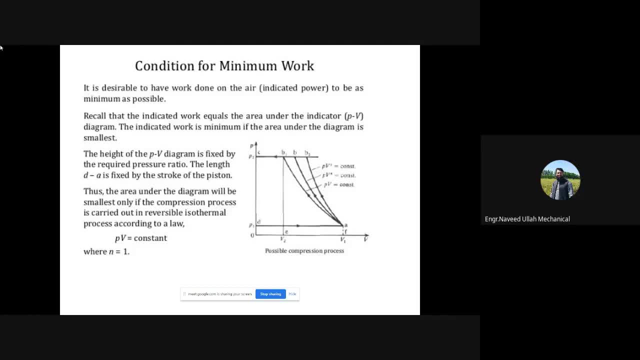 discussing about multi-stage compression okay so the first portion it was completed in previous class now after discussing some of the slides and some of the things we will discuss rest of the two bullets those were reciprocating uh air compressor with clearance volume and then 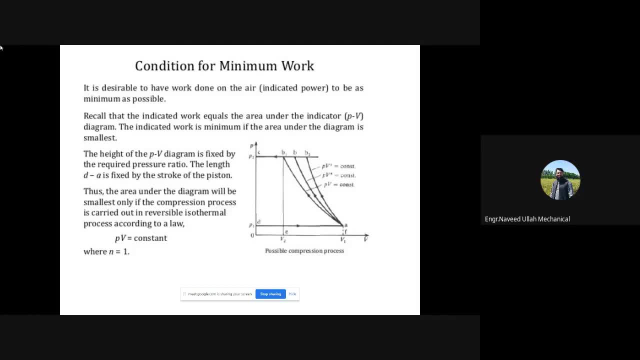 why we need multi-staging and what is a multi-stage compression okay so today's discussion will be about that thing right so you see here there is a topic that is condition for minimum work 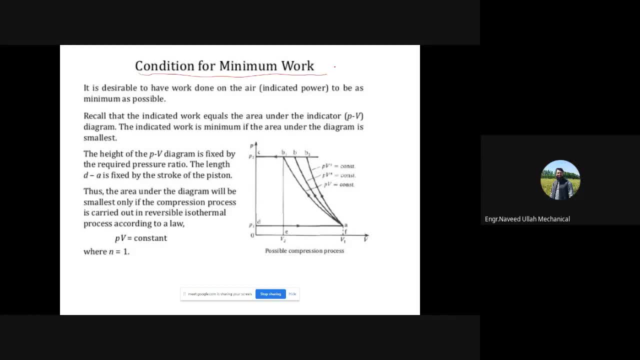 right the first thing you need to know that compressors are power consuming devices 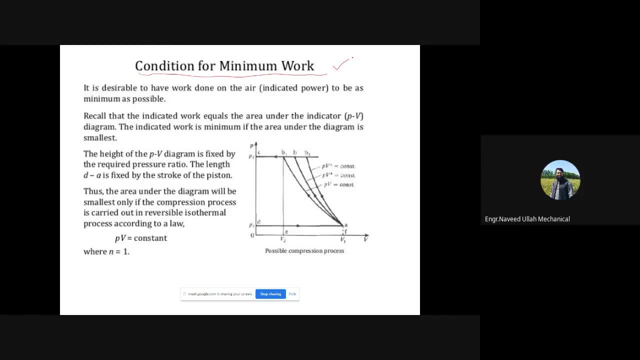 right as i told you and i am telling you so uh work consuming a power consuming device so being an engineer what need to what you need to do is 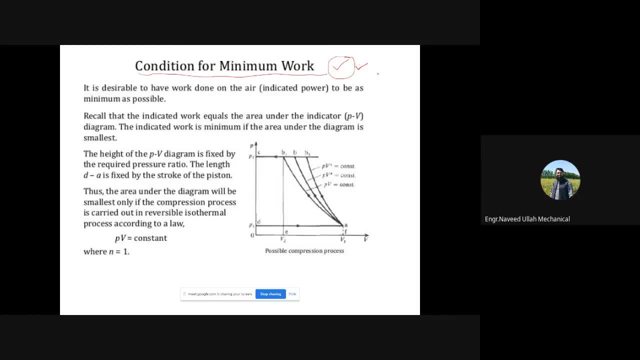 if there is an equipment that consumes power so we try to decrease that power consumption right and as far as the power producing devices are concerned somehow we do something with the machine that can increase uh you know the power output so in case of power producing devices 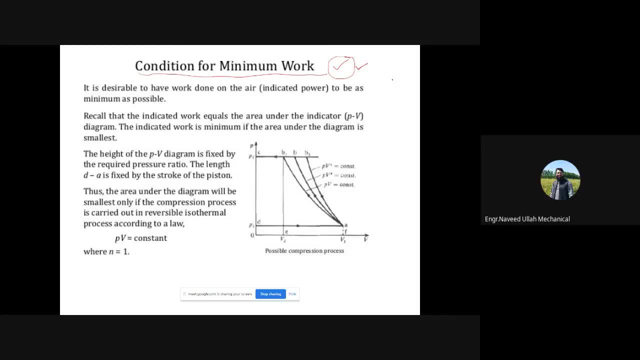 we want to maximize the output in case of power consuming devices we want to minimize 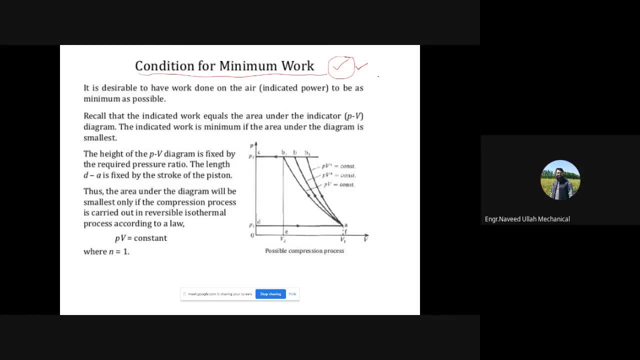 that power input so this is actually this idea is you know about that thing okay 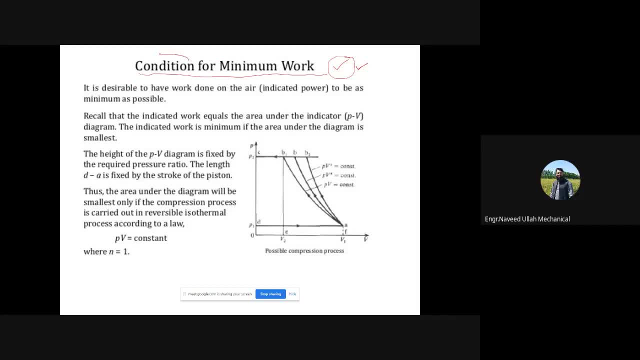 so condition of minimum mark what will be the condition okay that you can apply and the work consumed by the compressor will be minimum work consuming devices right so you can see it is desirable to have work done on that is always indicated per per you know per mass unit mass load rate 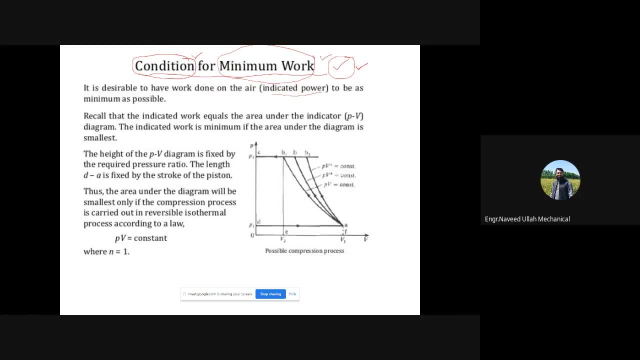 that will be indicated power to be as minimum as possible 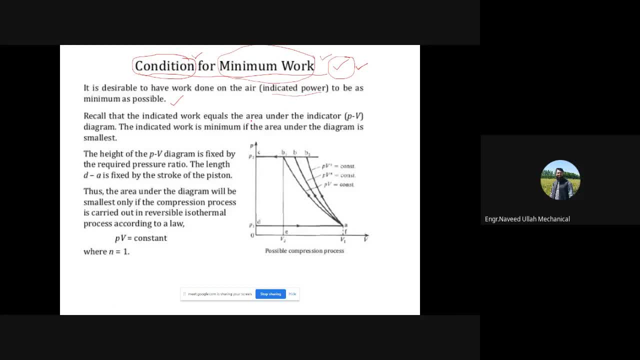 so they are saying that recall that the indicator quirk equals the area under exciter or pv diagram previously i'm learning the indicated work is minimum if the area that the indicator is unknown or the per watt of current or v di diagram- so this is the difference as you know the indicator work is minimum if the area the work resume if the area is minimum right so we can see under the diagram is smallest it is very simple right that the indicator diagram that is the PV diagram okay the area under this PV curve okay that is basically the work consumed are the indicated work okay so if this area is minimum consequently the work consumed by the compressor will also be minimum 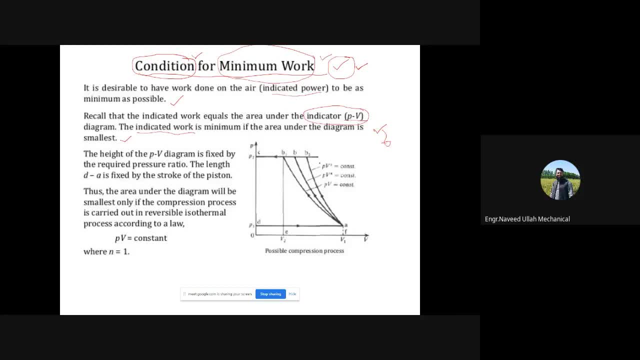 right so let us see that how we can minimize this work consumption so you 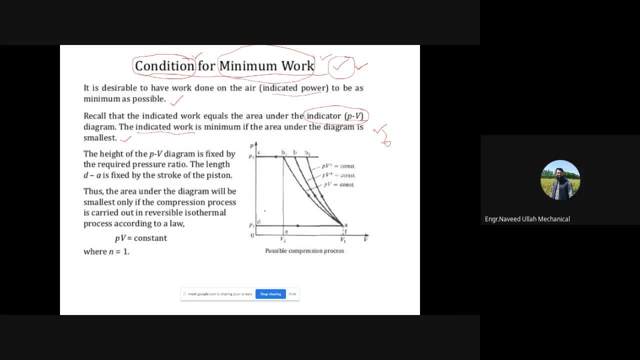 can see here there are three things okay you know very well that this is constant pressure induction process this is compression process the middle one polytrophic compression process 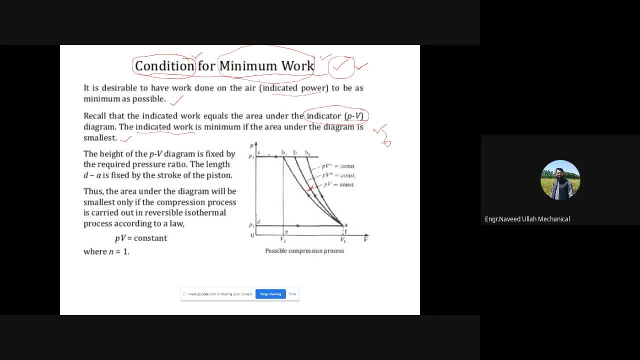 A to B and B to C is the constant pressure delivery process right now 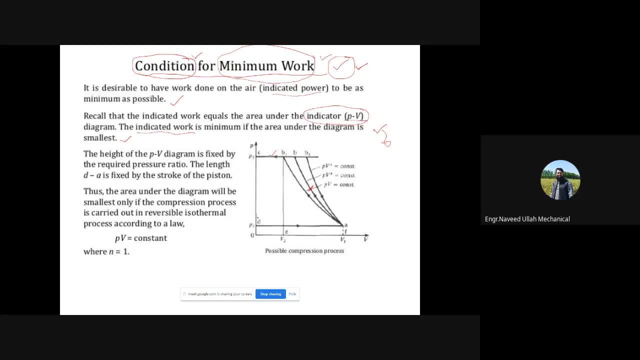 there are several ways to decrease this area under the curve one is that if for example you take this line to this position okay let's say for example similarly you can take this line from here to this position okay so you can see that you can decrease the area under the curve and consequently was consumed by the compressor right but these two things are actually not possible okay you can say they are not practical okay let us talk about P 2. if you are taking this line from here to here you are 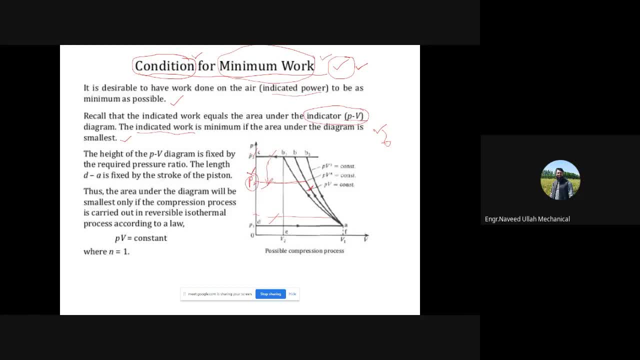 basically compromising on this delivered pressure which is not You know, which is not required We want that the pressure of the working fluid that is here in this case to be p2. That is this one 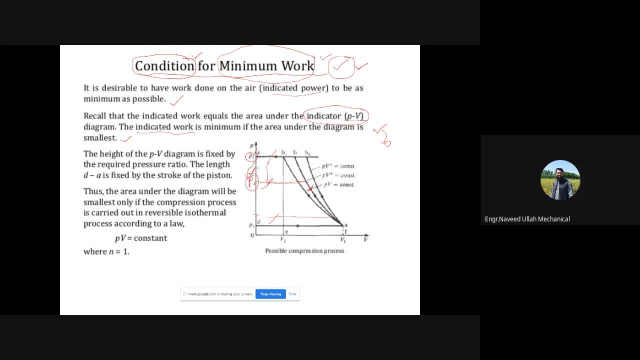 Okay, we don't want to come to compromise on that. It's one coming here sickly 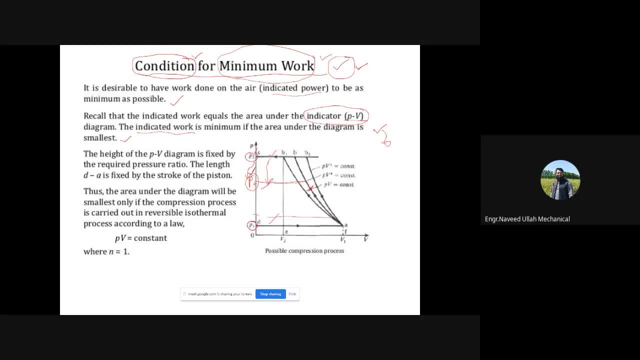 Right. Similarly, this is a pretty initial pressure before compression. So this means that equally these two 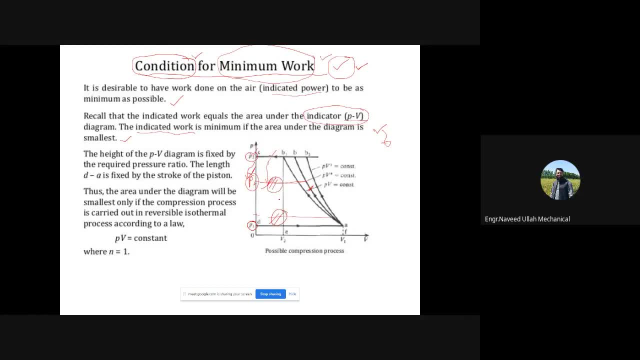 You know amendments are changes are alteration. They are not possible. Now the third one that is remaining here This is basically somehow you can do something with this compression process 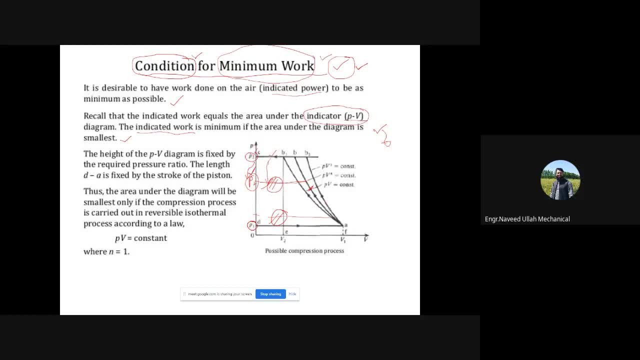 Okay, so you can see here this line a B Okay, this one this is polytropic compression we are pvn is equal to constant 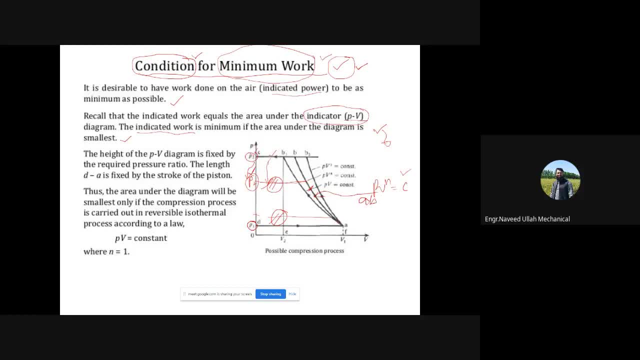 right this a b1 A b1 Okay This is a pvn You know, this is 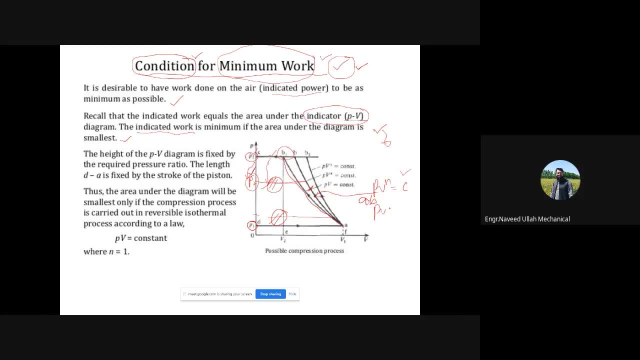 Isothermal process right that is pv is equal to constant That is this is isothermal process right 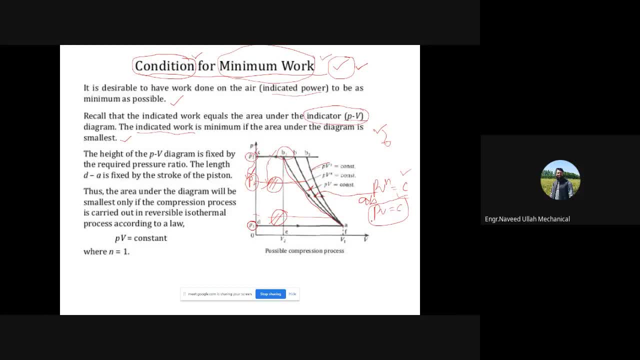 And similarly this one a to b2 this a b2 this is a pv gamma is equal to constant that is isentropic classes, so we have isentropic compression Isothermal compression and polytropic compression and you see that 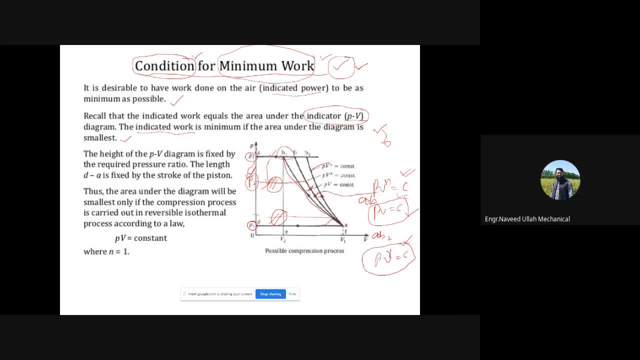 area under the curve for this isothermal process is the minimum one Right. This will be the minimum area This one is you know 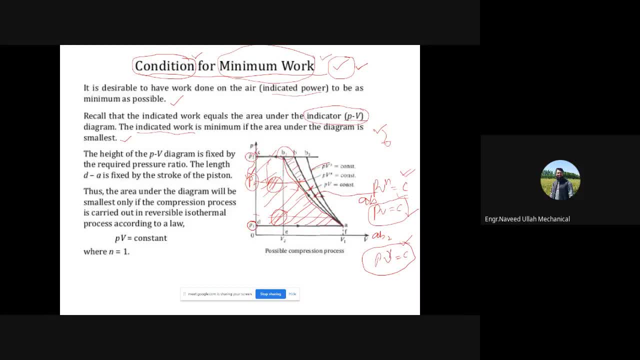 You can say that this is greater than isothermal process and for isentropic process This is even greater so 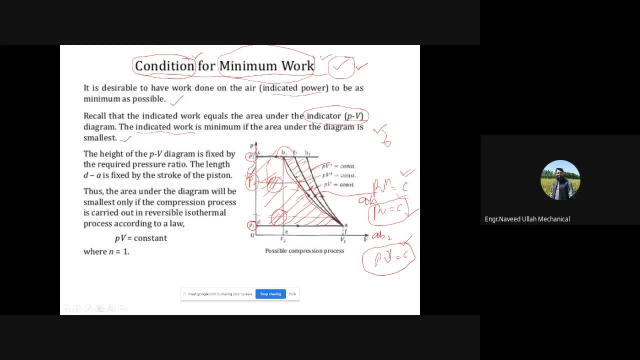 to summarize it if you want to minimize the work consumed by the compressor in 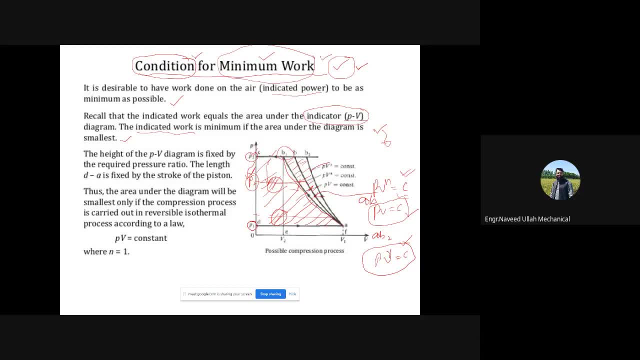 this reciprocating air compressor this Process of compression should be what should we has a thermal process? 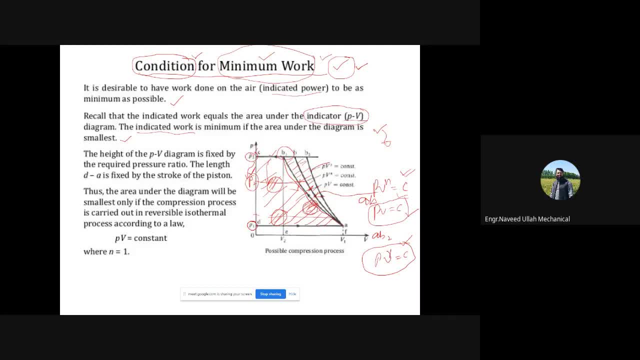 Okay We care process logo octopus. This will be I so thermal process. Okay ah 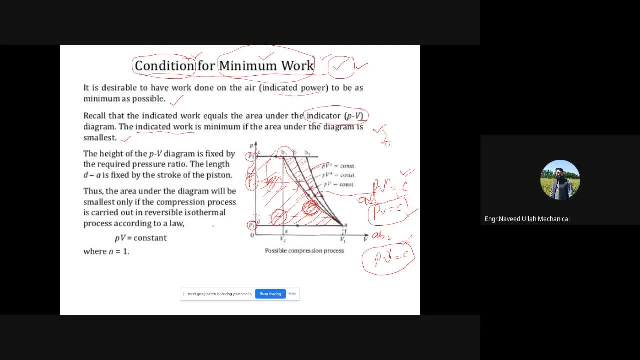 um so somehow if you can achieve this pv is equal to constant as a thermal process so up is area under the curve and consequently were consumed by the compressor right 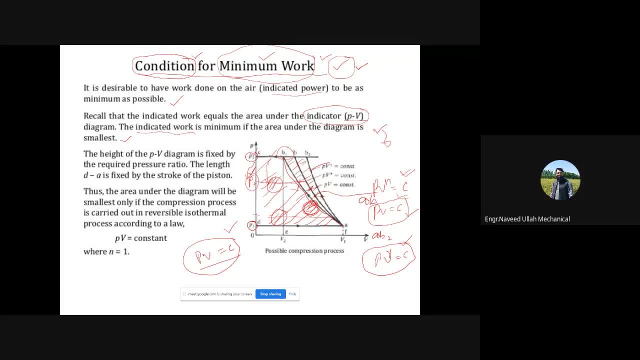 then we will discuss that um it is a bit difficult to achieve this process okay in a single cylinder so we can actually move to multi-stage compression but that is equally discussion in the later slides now this is actually the black and 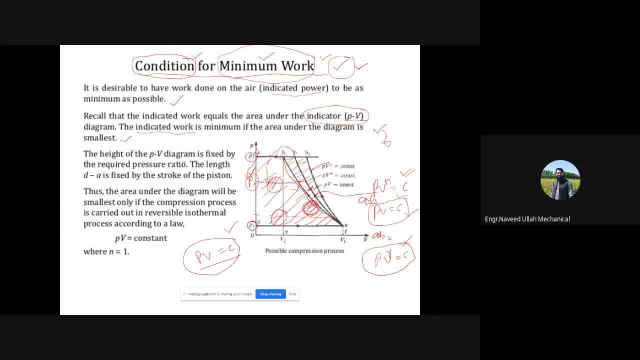 white what we have discussed already the height of the pv diagram is fixed 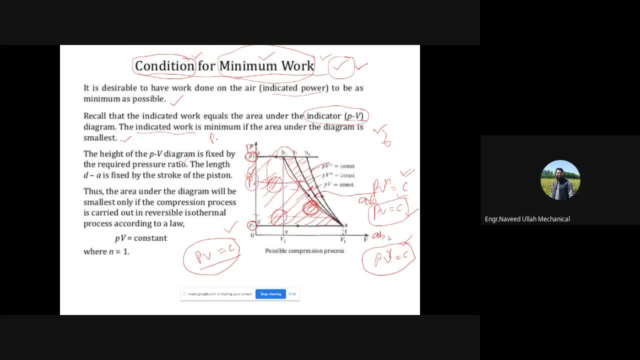 by the required pressure ratio pressure ratio that is p1 p2 by p1 if you change this p2 to 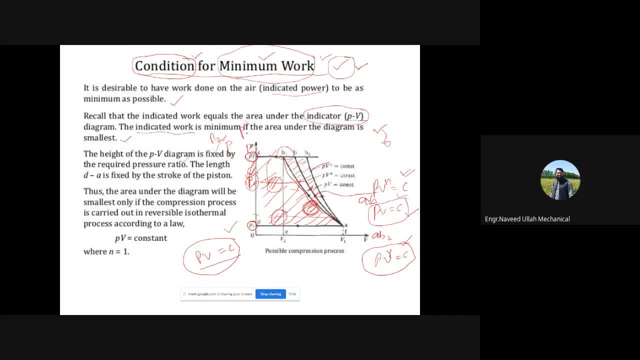 this let's say p2 bar p2 bar divided by p1 now this is not the required pressure ratio right so we are basically compromising 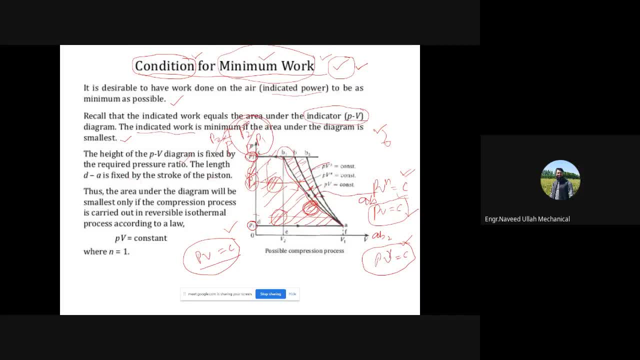 on this the length da is fixed by the stroke of the piston now this is the length d a d a 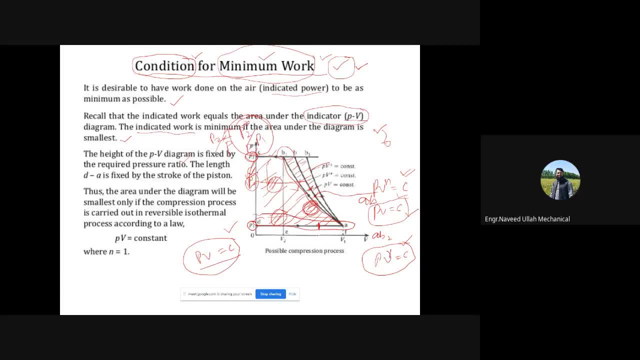 right this is the induction value you can also have this here so this is actually 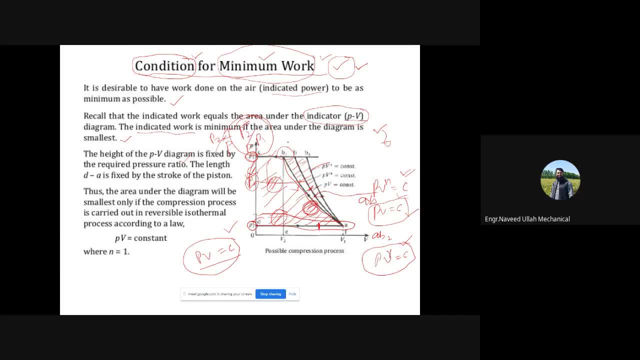 this is uh you know this is also fixed right because of this piston stroke 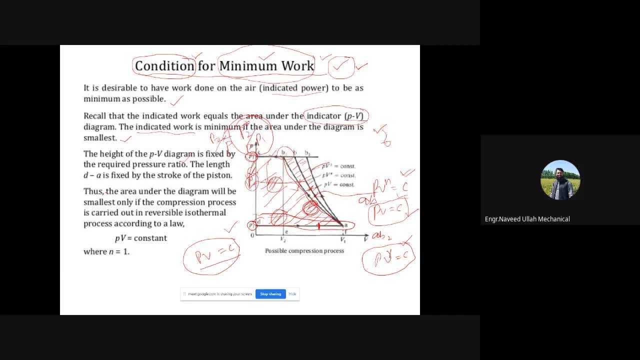 cylinder volume right so thus they are saying that the area under the diagram will be smallest only if the compression process is carried out in a reversible isothermal process according to the 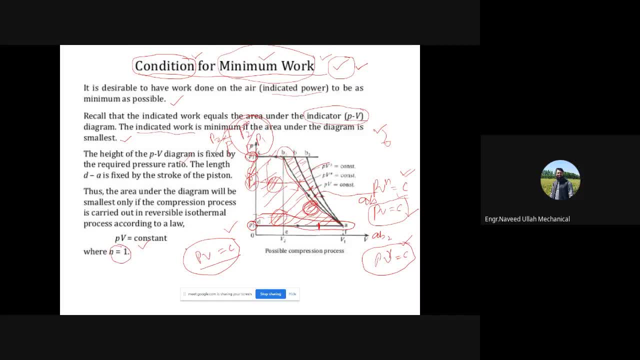 last in this one where the polytropic index is a one right in if you take this equal to one 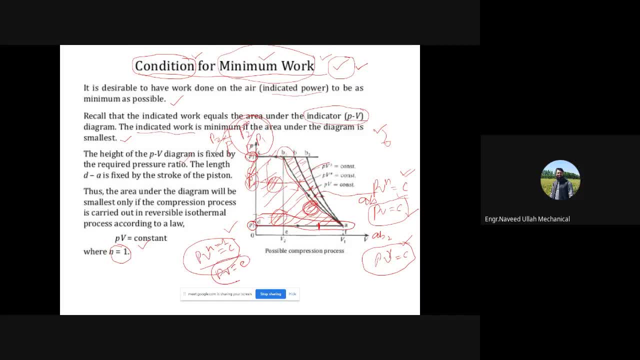 right so this will be pv is equal to constant okay so the summary of this slide is you can see in the indicator of the pv diagram if you somehow can achieve the isothermal compression process 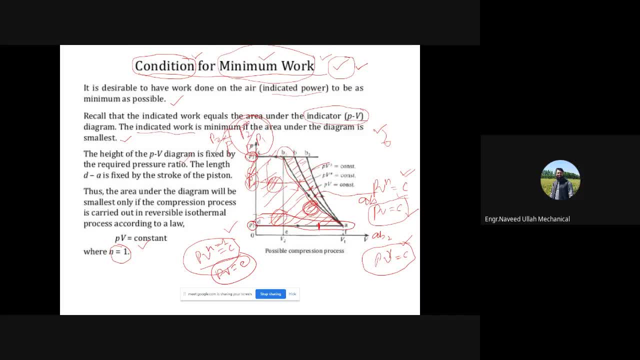 you can decrease the area under the curve and ultimately the work consumed the work consumed the power consumed by the compressor will be minimum so that is basically condition of 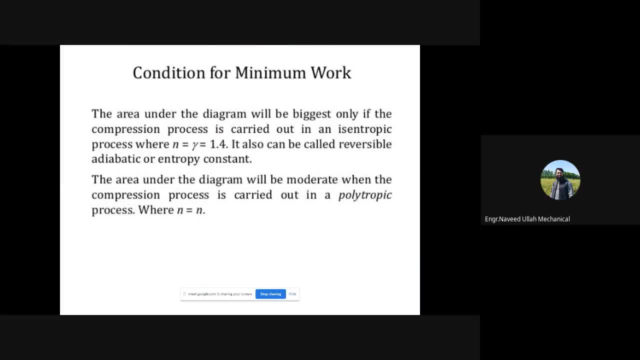 for minimum work right um that they are also explaining that the area 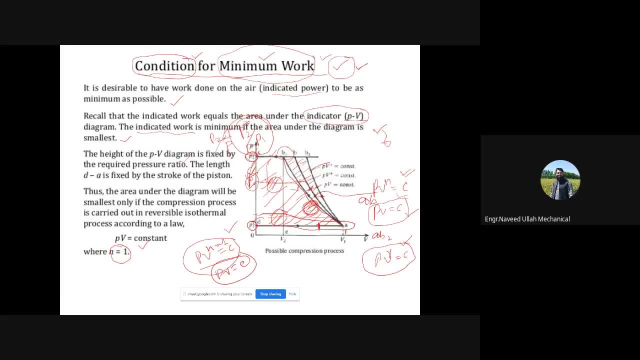 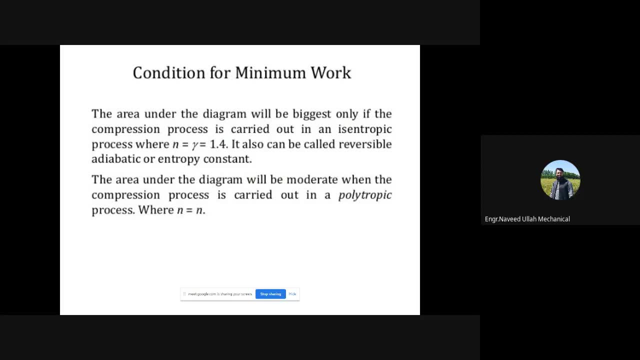 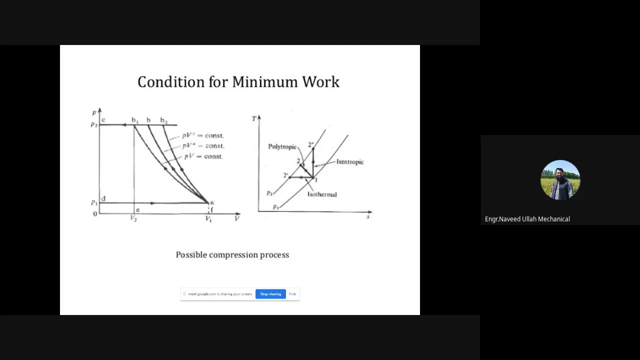 in the same diagram okay they are referring to this is this indicator diagram the area under the diagram will be biggest only if the compression process is carried out in an isentropic process where n is equal to 1.4 it is equal to 1 keel here isothermal minimum power work consumption it is equal to gamma is equal to 1.4 keel here apke paas jo work consumption hai ho zyada ho gaya it can also it also can be called reversible adiabatic or isentropic process the area under the diagram will be moderate when the compression process is carried out in the polytrophic process we are in is equal to and so the best one is the isothermal process right we can also look at this one okay this is a the pv diagram 200 is clear and this one is the TS diagram you can also look at this one right that this is equity in this this is isothermal process this one is a polytrophic process and this one is isentropic process okay and the work consumed will be less for the isothermal process okay and similarly yeah you can 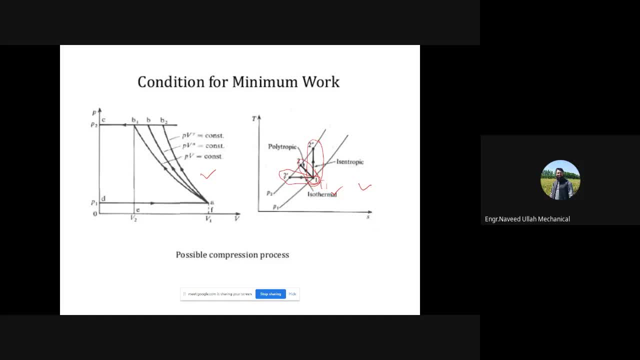 see that in isothermal process temperature t1 and temperature t2 paths 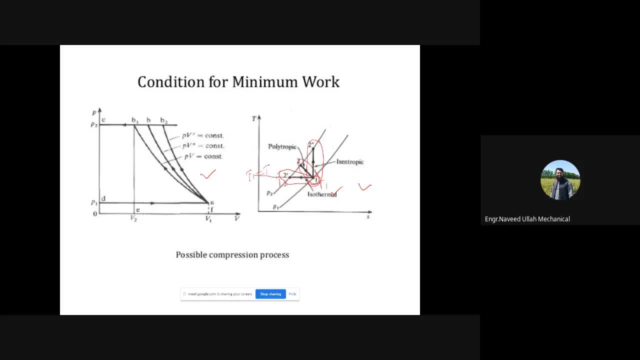 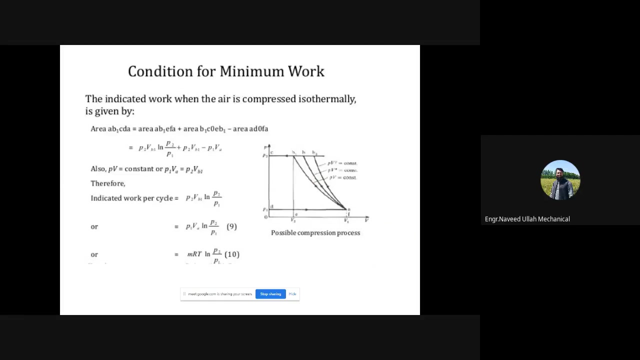 they are the same t2 bar they are the same so this means that it is having complete intercooling process right the pressure increases but the temperature remains the same pressure increase with the p1 say p2 right but the temperature remains the same okay and that is equally what we want right because if you remember i told you and i used to tell you that when in the compressor the pressure increases and undue temperature also rises that undue rise we are actually restraining over here okay and we are restricting it over here so obviously uh we we developed the formula for uh you know indicated uh work uh and similarly 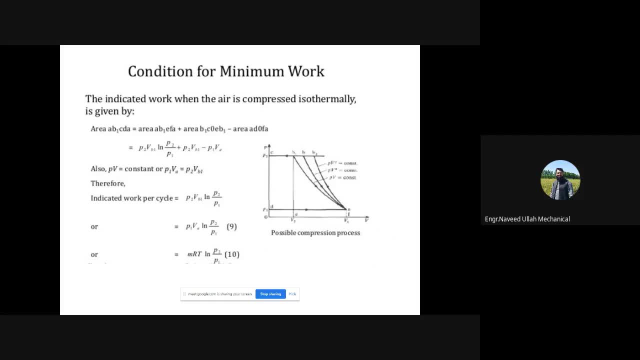 indicated power for puritropic process now if uh you you know use the condition of for minimum work means isothermal process 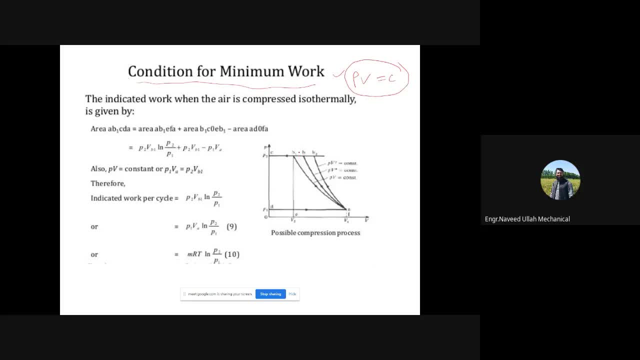 okay what will be the work consumed by the compressor so actually here it is discussed in the slide the indicated work within the ear is complete compressed isothermally is given by what you know area a b1 cda a 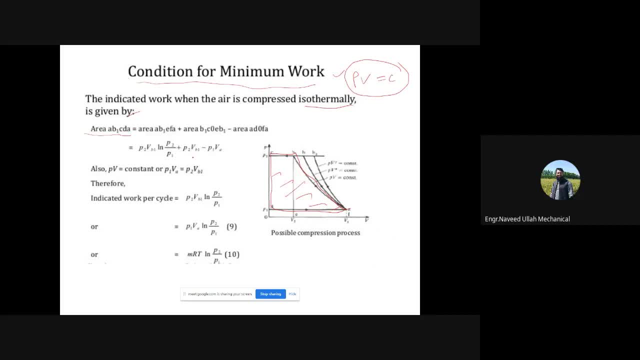 c d a this is actually that area under the curve right and uh these two are actually the same 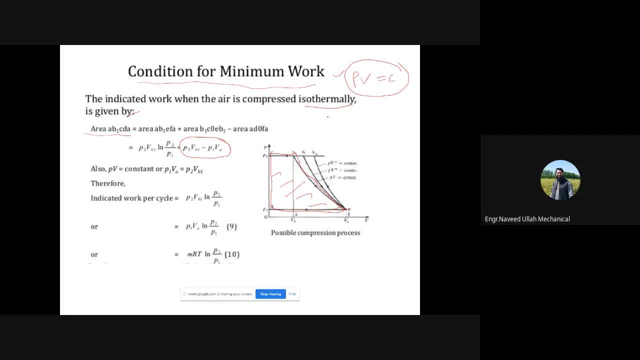 but uh maybe you know about this thing as i told you earlier that uh area under the curve for isentropic process polytropic process and isothermal process they are different right so for polytropic if you remember we discussed that that is n by n minus one i think that is a p two v two minus p one v one if i correctly remember previously i'm not discussed 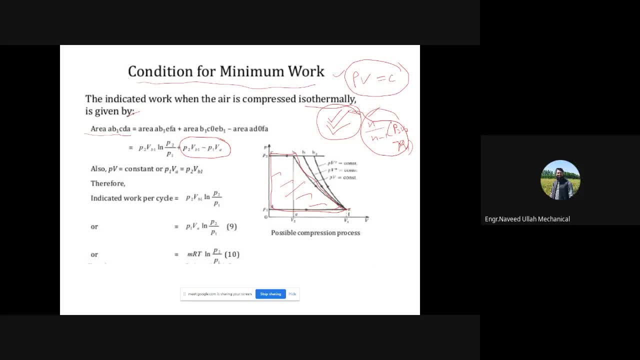 this is for what this is for polytropic process for uh you know um as a thermal process it is like this okay it is actually this one 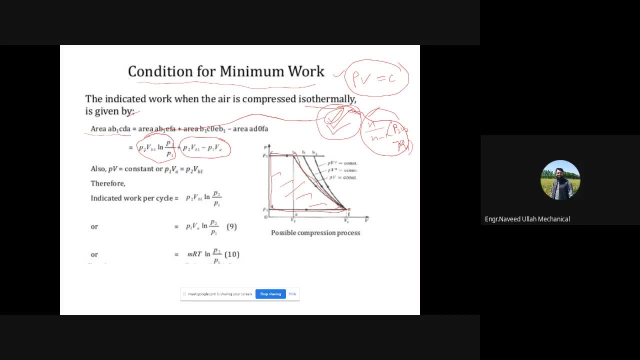 basically using integrals etc to derive this formula p2 vb1 log of p2 by p1 that is what that is your work in the isothermal process okay um right so you can say that you know this you can 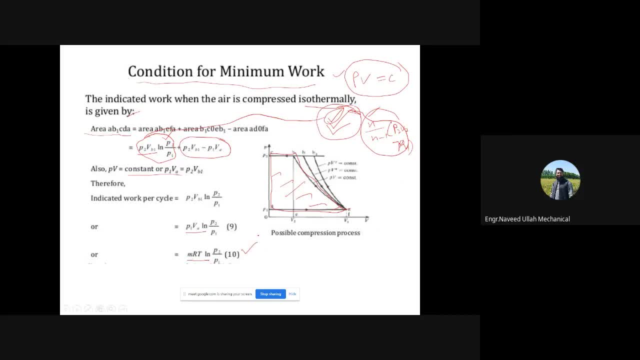 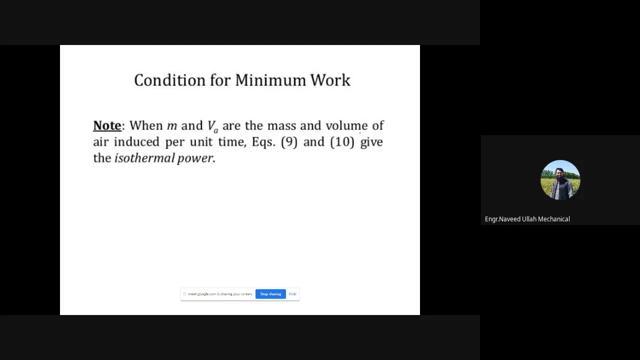 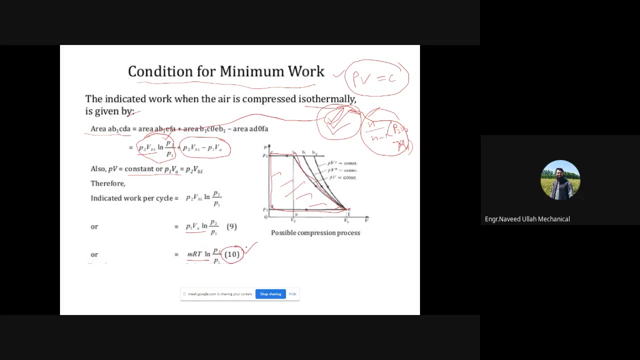 you know they are saying that when m and va are the mass and volume of air induced per unit time equation 9 and 10 give the isothermal power so this equation 10 right it gives you indicated work per cycle similarly if you take that equation in polytropic process so that also gives you indicated work per cycle and the work consumed by the compressor okay for this uh you know using this equation for the same pressure ratio will be less than for the one that we discussed earlier 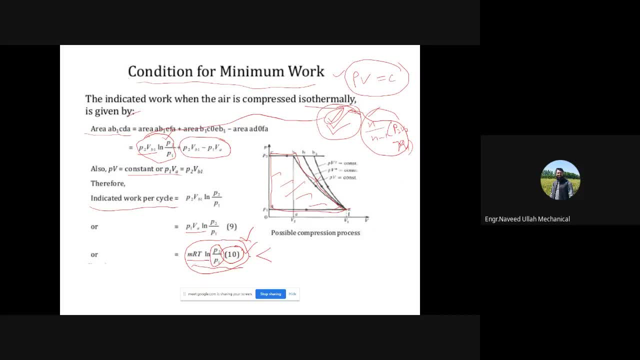 consumption example consumed by the compressor if the process is isothermal is 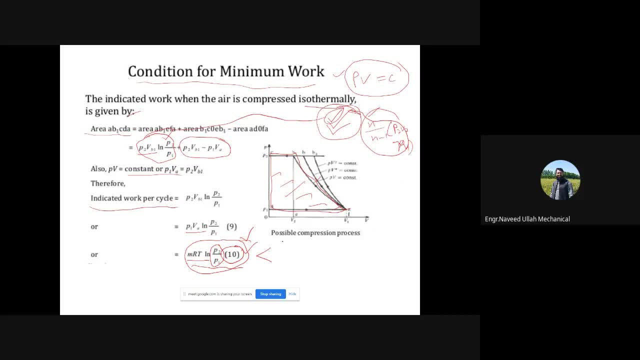 less than when the process is polytropic or isentropic so if the process is of thermal this is the relationship or this is the relevant formula to find out indicated work cycle and the one that we discussed earlier is for ice you know polytropic process right 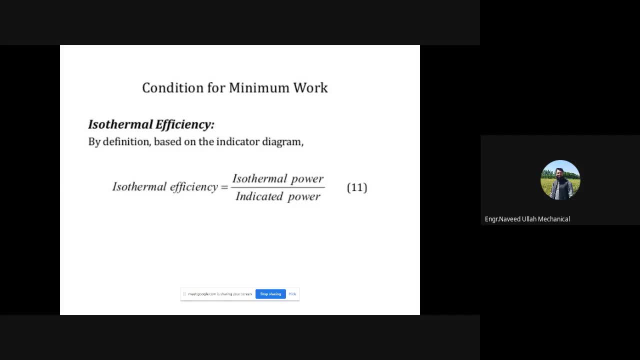 and in the same way we are basically repeating things okay previously we also have this as a thermal efficiency but 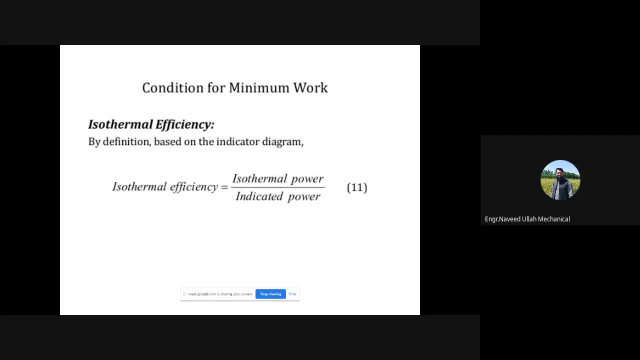 similarly mechanical efficiency but the process was polytropic now if you want to find out isothermal efficiency based on the indicated diagram that will be isothermal efficiency the work consumed are the power consumed by the compressor when the process is isothermal okay let's say it's not power consuming and the power consumed by the compressor is isothermal um 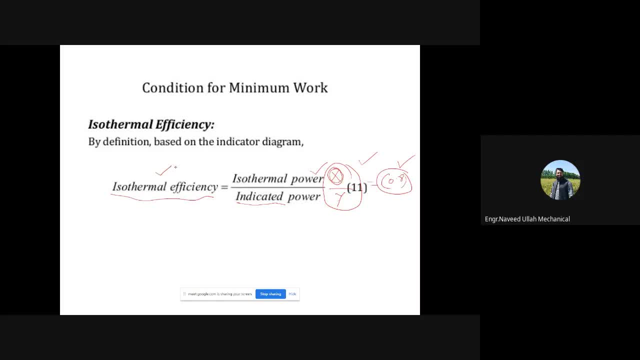 isothermal efficiency that is another discussion okay exactly and completely reversible isothermal process is very 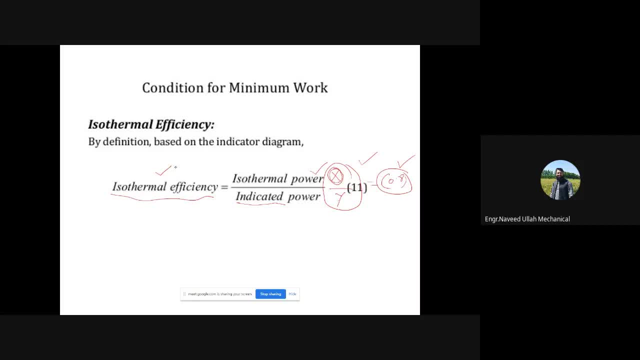 slow in nature and it is not practically possible so for that reason you need to have isothermal efficiency 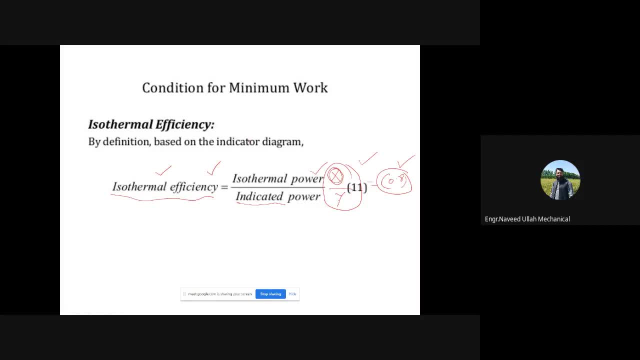 Efficiency comes when you deviate from ideal behaviour or from 100% efficiency 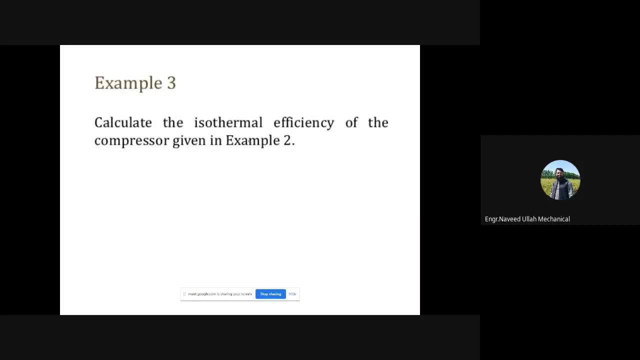 One example is Calculate the isothermal efficiency of compressor given in example 2 There was an example 2 in the previous lecture and over there we found out the work consumed 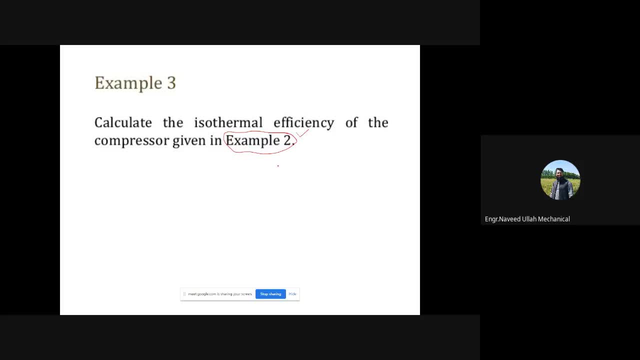 by the compressor and similarly we also have those efficiencies etc so they found out if the indicate sorry the mechanical efficiency okay so the work consumed by the compressor in polytrophic process is there right and you can find out the work consumed by the compressor when the process 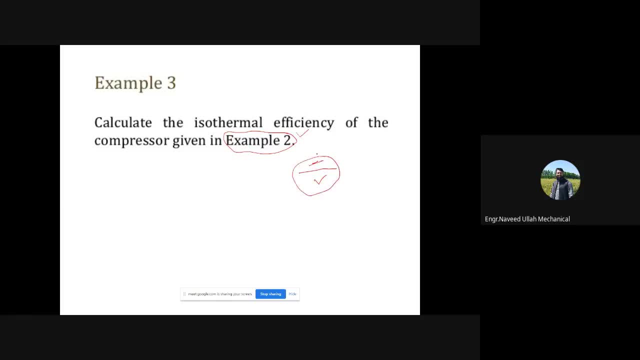 is isothermal and just divide this one that you calculated now by the one that we have in our previous you know example you can get the isothermal efficiency A salt for example I have put sugar 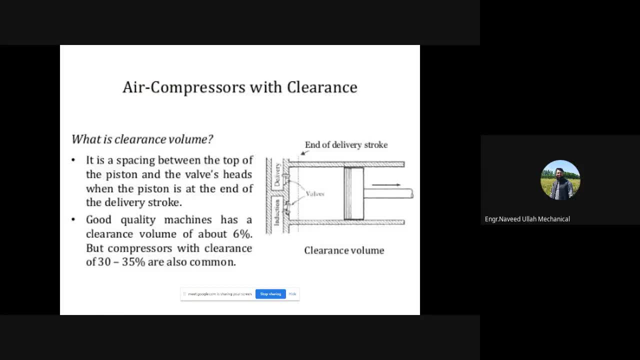 Right so the condition for many members if you know if you want to decrease the work consumed by the compressor that actually we want okay in order to increase the 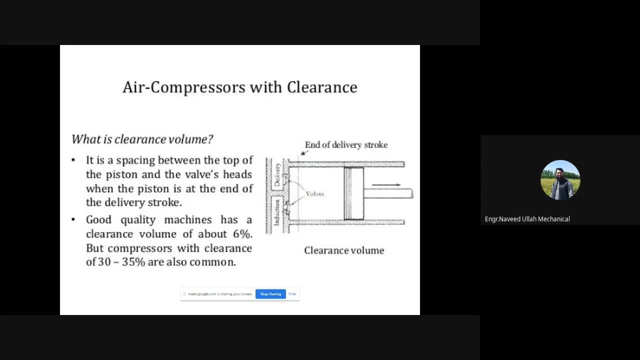 efficiency there are different possibilities but some of them are not practically possible 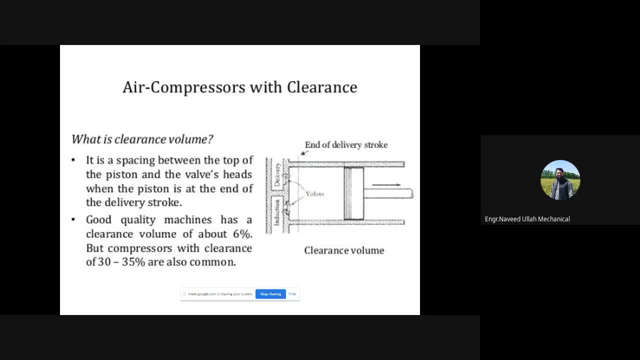 as far as the indicator diagram the p-v diagram is concerned we can do you know alteration over there we can decrease the length of a line you can take the line P2 down there but 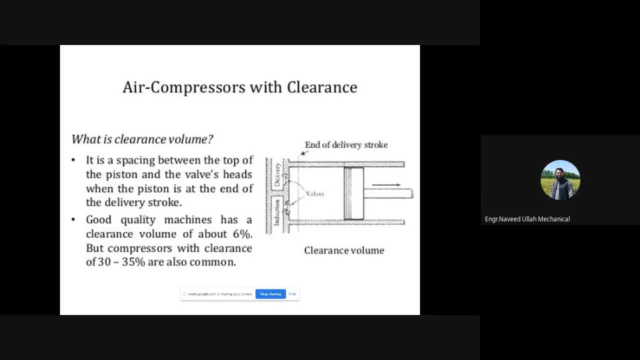 they are not practical right the one that is practical and it is most reactive is going 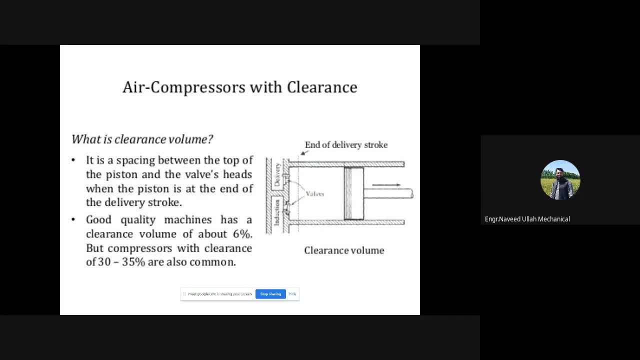 most be achievable is to change the process from polypropyl to isothermal and that's where you can get the you know the minimum water okay and that is 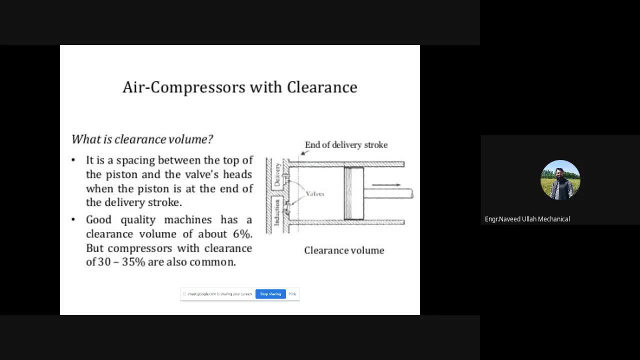 depicted and explained in an example three okay we are previously for the same data and from the same for the same pressure ratio the work consumer the compressor is calculated and then the isothermal power is calculated our work is calculated and then they found out they found out that this is opposed to 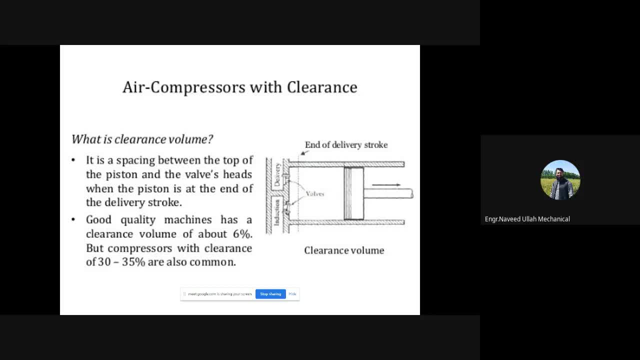 the one that we calculated earlier for will traffic process and we will be having some thermal efficiency that's it right then after that as I told you that we need to discuss the other bullet and that was what 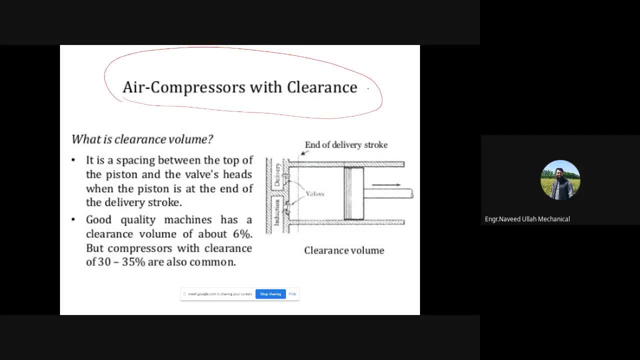 we did clearance volume and if you remember I told you that here compressor without clearance volume is not a practical case ticket Cunha we have 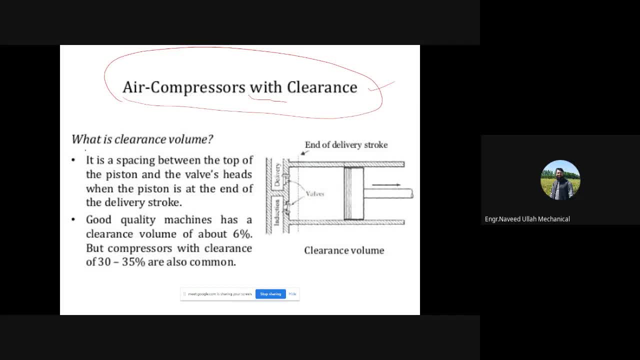 discussed right what is clearance volume are in other words I should say why clearance is needed okay so what we have discussed currently it is a spacing what 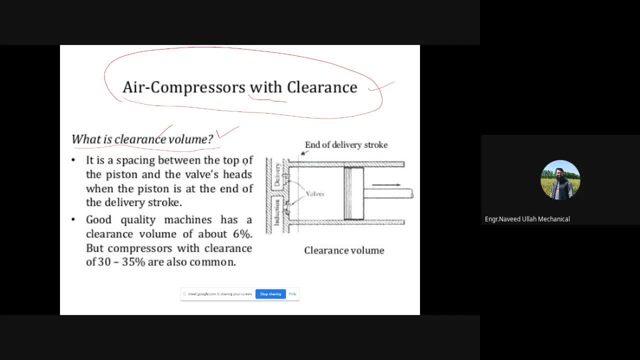 is clearance volume it is a spacing between the top of the piston top of the system 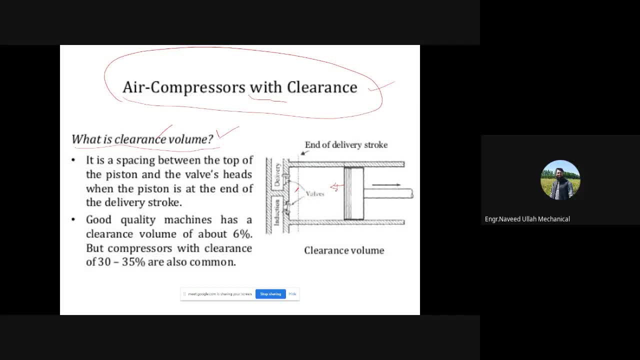 and the piston is moving in this direction yeah and it comes to this point what is this point he discuss and the wall header you walk ahead when the piston is at the end of delivery stroke right it is a for example let's say for example it comes here okay and 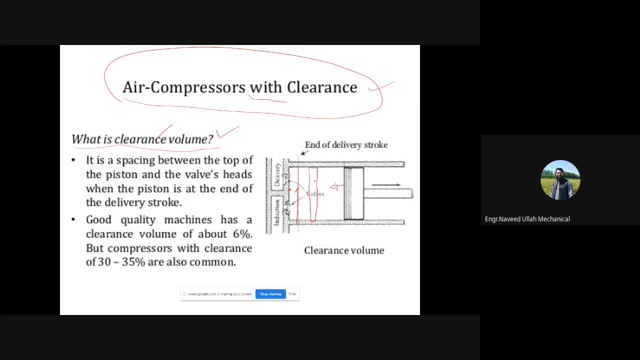 when it comes to this position it has developed the required pressure now the movement from here to here it will deliver that pressure okay it was exaggerated it is not like this it is we are having clearance volume very very small clearance volume okay about six percent but anyway i just exaggerated this so now it is uh now from here it is starting delivering or it starts delivering the you know uh the ear okay that required pressure and when it this 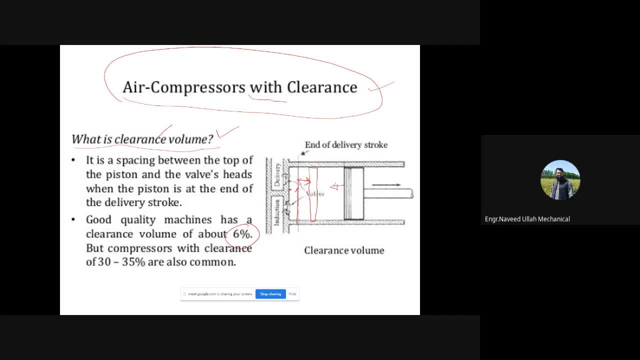 piston comes to this point okay this position it has delivered all the pressurized here okay except the one that is stripped in the clearance right so now at this position when the piston is what is at the end of the delivery stroke you remember right because this is induction compression and from here delivery starts this is delivery stroke so not at the start of the delivery but at the end of the delivery stroke so the distance between uh this is you know the space between the piston head and here the 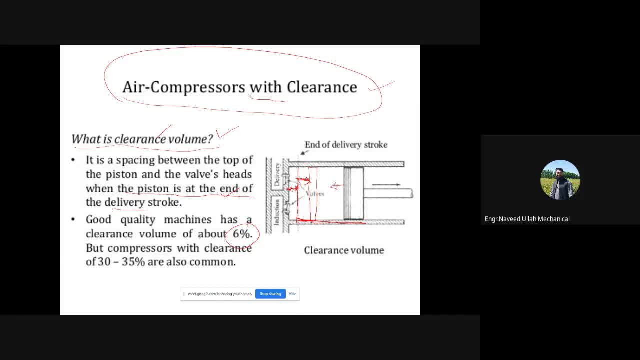 valve head okay at the top of the piston and the wall heads so this will be your clearance volume 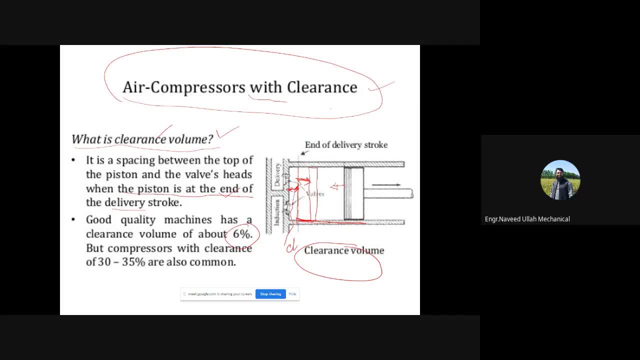 definition is simple the space between the piston the top of the piston and the cylinder you know this wall head this this space is basically your clearance volume but when 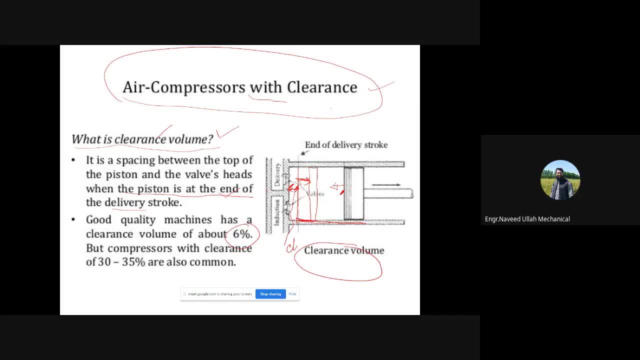 not all the way right after all the position when the piston is at the end of the delivery stroke or the end of the video is 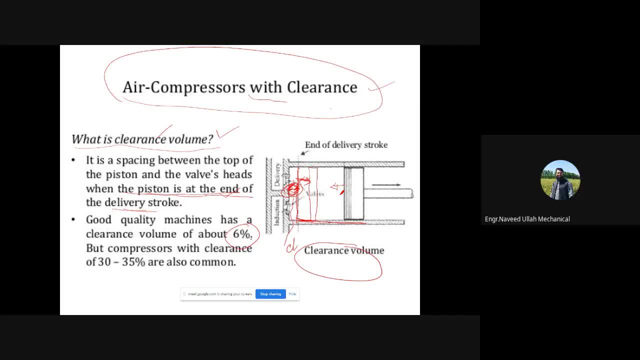 good quality machines has a clearance volume of about six percent six percent 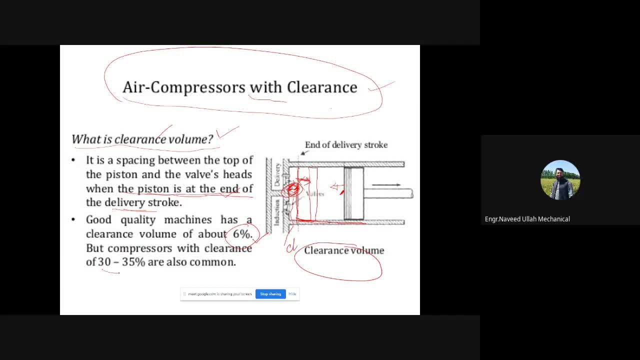 Chloe says here both have 60 voyez и 20 was testing ssc of 30 35 is not hard and faster it depends on the design proper why because the the moto for clearance from 30 has 30 to 35 but it is not hard and faster depends on the design why because the the motor for the clearance value is 24 crowd is not a community against veg answer to every video hopeless and i had asked me about them asap that why they use to update 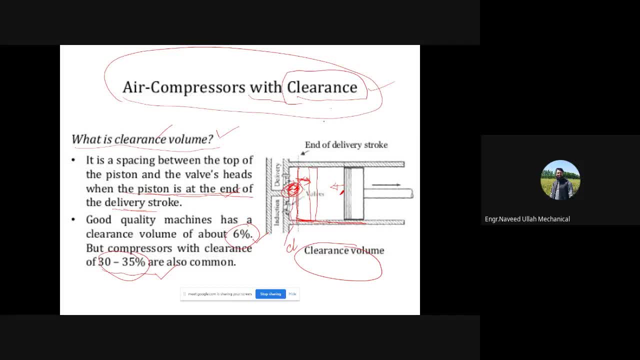 For clearance volume is a pretty different. Okay, here is give you a Zulu. Yeah, remember We will see 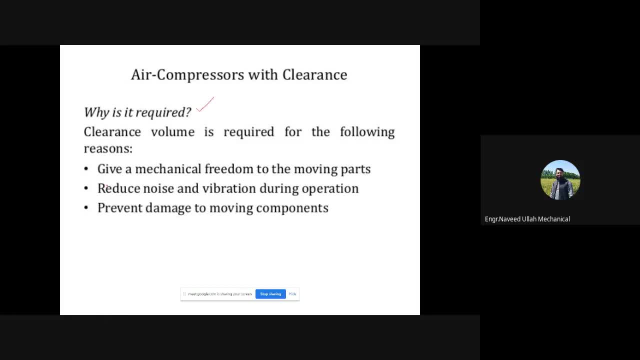 Why this is this clearance is required. So there are actually three things. Okay one Cleanest volume is required for the following reason. One is give a mechanical freedom to the moving parts. Look 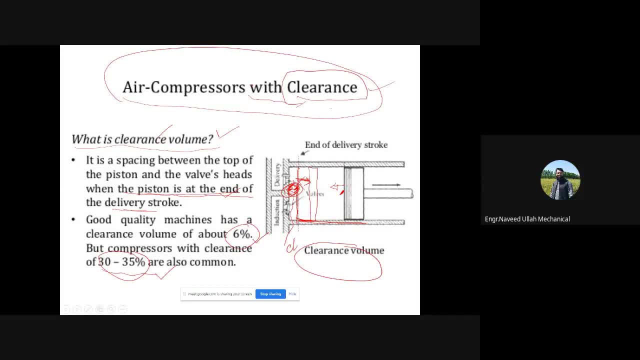 Yeah, pick it up easily. I mean, I could but I thought this is actually without please volume is not a practical case And I told you 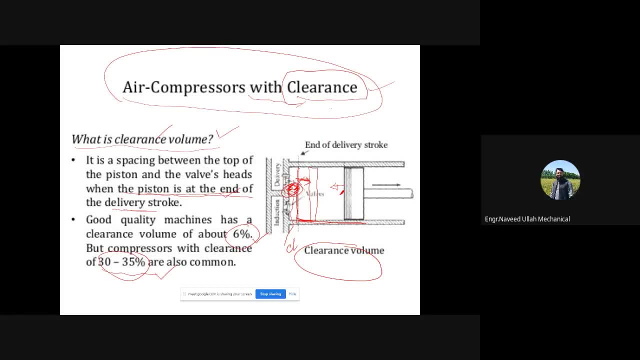 If you see here, this is a clean wall up there And particularly this one is the one down there. Okay, so if there is no clearance how this wall will open 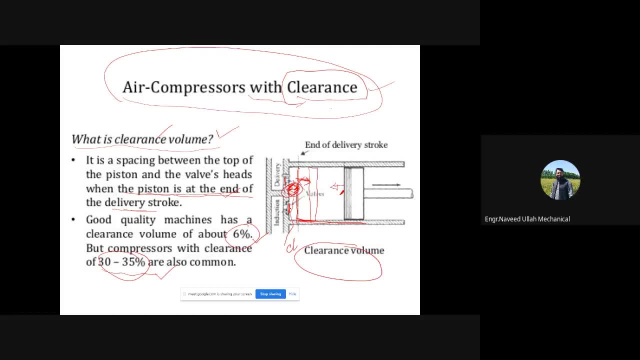 You are Casey open hoga. So I'm getting a mechanical freedom to this moving part You are movable in us. This wall is movable and the motion of this one is only possible when it is having some space over here so one is that we 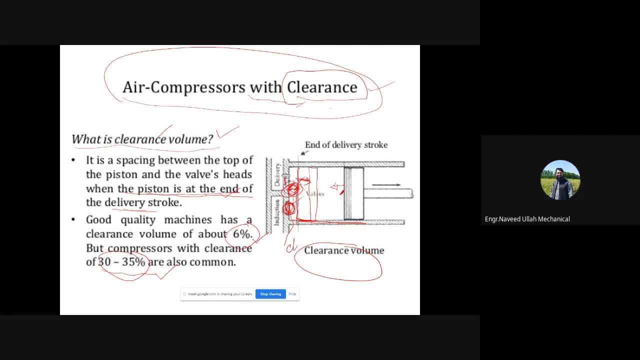 Don't want to constrain the motion of this walls But we give a mechanical freedom to this, you know moving part 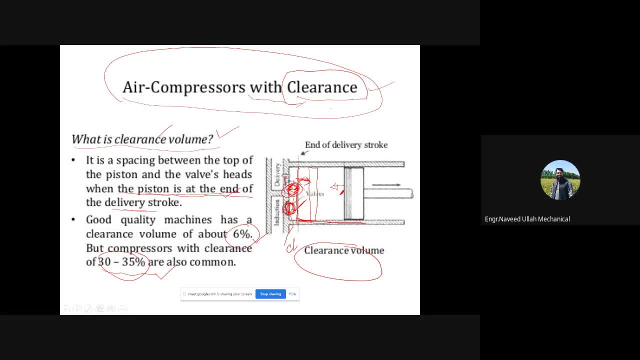 We need to have some clearance to take to your data, right? Do you see what I have reduce? You know nice and vibration during operation 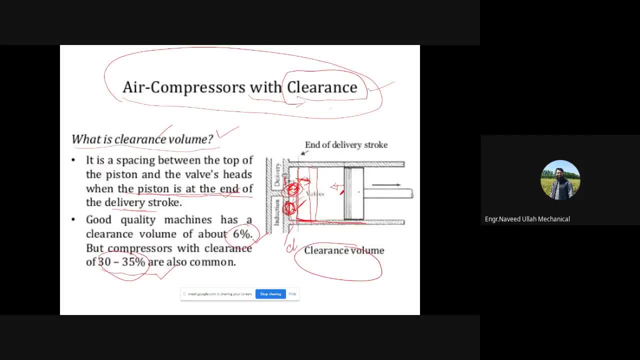 It is very you know obvious that if for example the piston is moving from here and it comes to this position and again It is coming here. So it will actually all the way be in 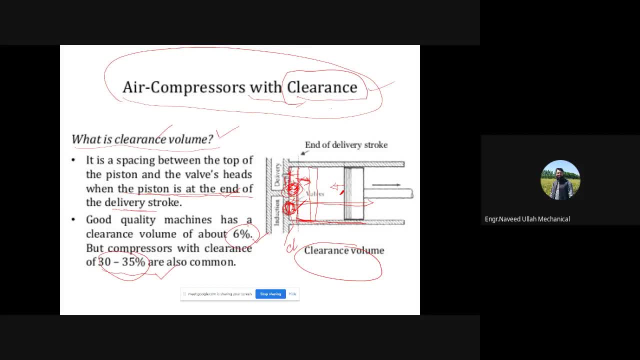 Contact with this wall this this head Okay, we are the way it needs to carry gonna tucker tucker tucker keep this case. How do I get a guy here in contact over? 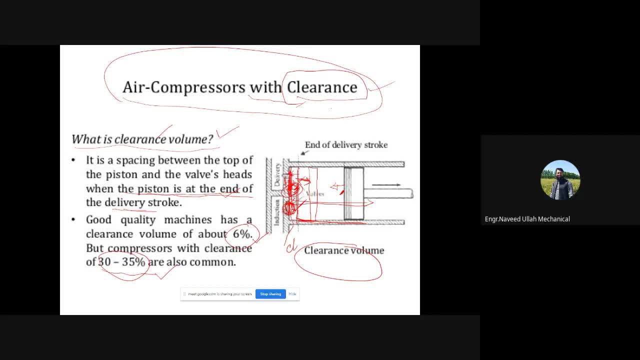 So it can produce where interior it can produce, you know vibration, etc Right and ultimately it can even wear the wall and the head. Okay, so easily 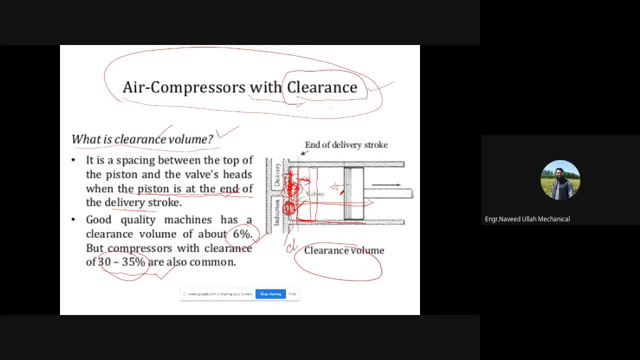 I don't have to take it to avoid this contact of the piston and this cylinder head Okay, this wall head. We Want to have are we need to have this clearance volume those usually and the third one is prevent damage to moving parts 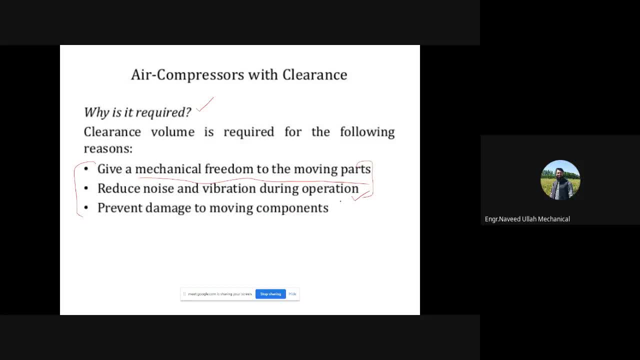 Very simple. This is actually related to even the first two that it is constantly in contact. It can damage the part 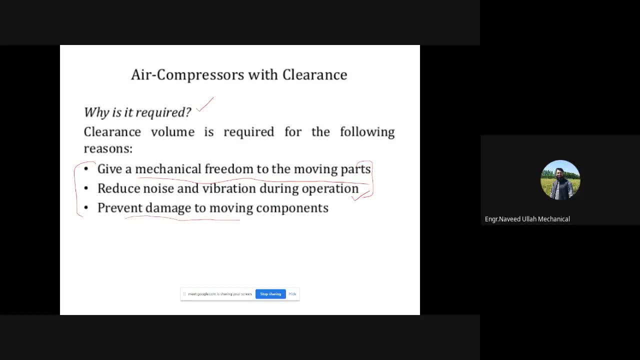 Okay, because there is a you know, there will be bearing stresses. Okay on the way. So for that reason if you want to you know Have these parts, you know 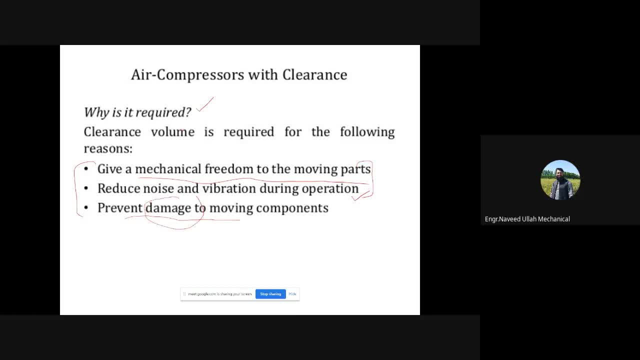 It's free. So you need to have this clearance over here. Okay, so this is basically the requirement for to clear is key But students have his therapy now from now onwards 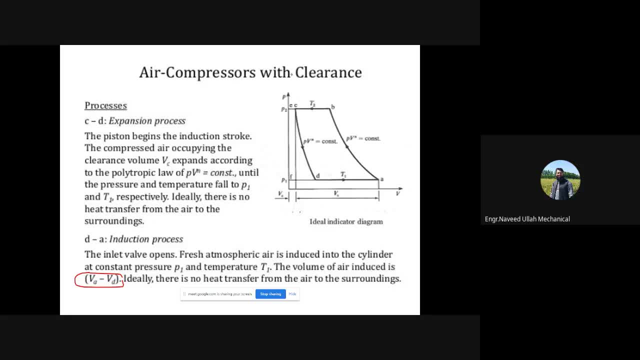 Remember that we have developed developed relationships and we discussed about different things for the previous case and that case was clear, you know 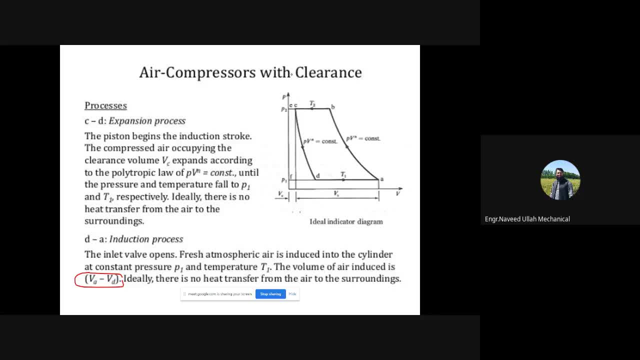 getting ear compressor with out clearance volume ticket with clearance volume carrying in a Will not be going into? 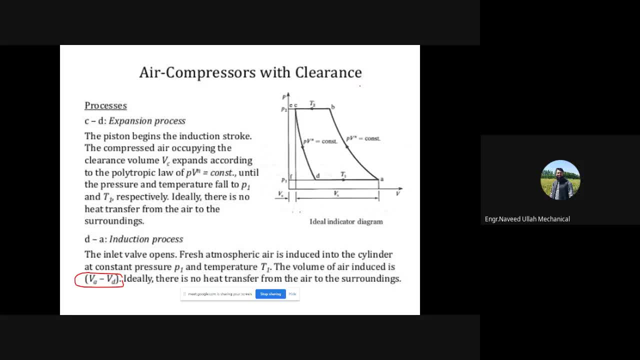 Too much detail, but we will be just changing in, you know, altering those relationships. Okay, so you can see here Almost this is the same diagram ticket, but a little bit different how it is different because of this clearance volume So you can see here one is that there is 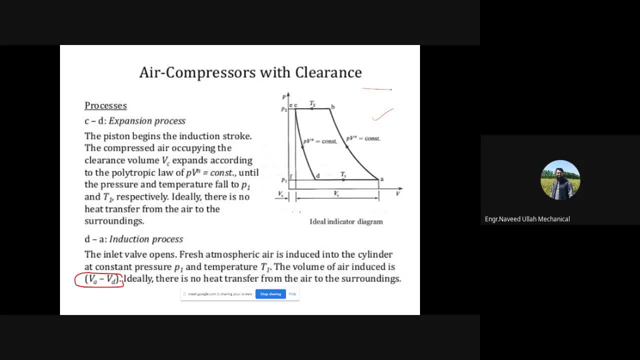 Over there. We were having induction Compression and delivery strokes, right? So three strokes for this now here will be having four strokes induction 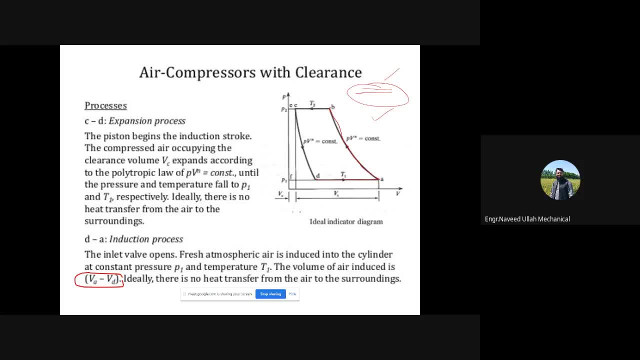 Compression the same way Delivery And then expansion 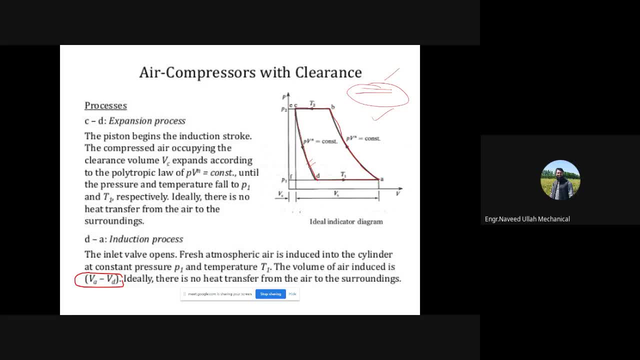 Yeah, hey Expansion expansion control. Yeah, this is extra 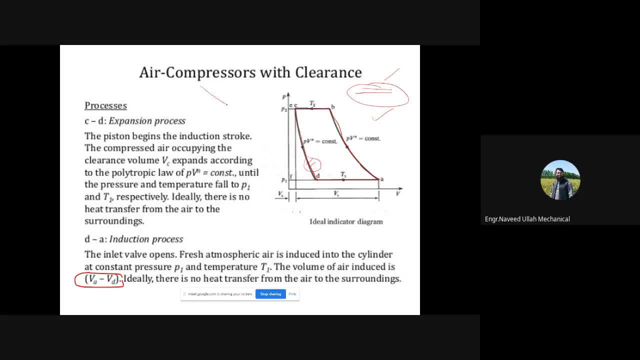 Expansion, you know very well High pressure say to blow pressure get about a henna. Oh, so I'm getting an expansion pressure drop 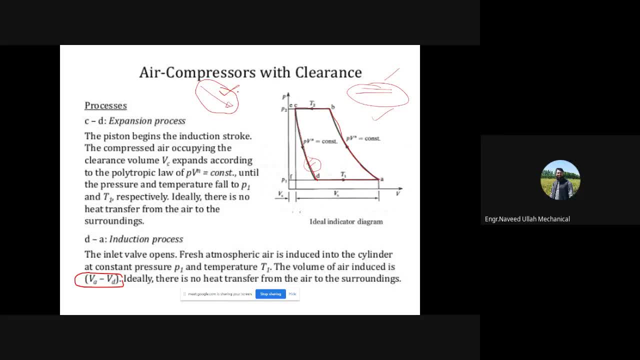 That is known as expansion process to give you this many a is may hey 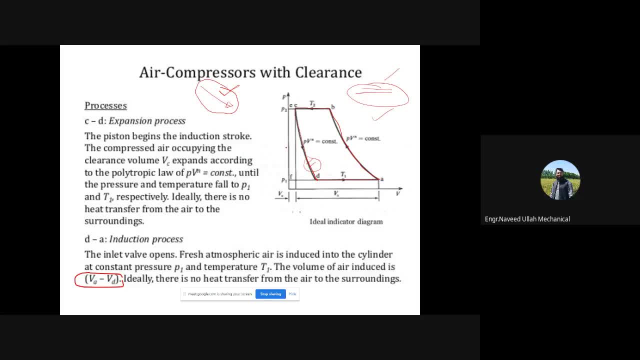 Or do you get the request ahead? So yeah, I'm yeah, but we're gonna just go discuss. This is the same look 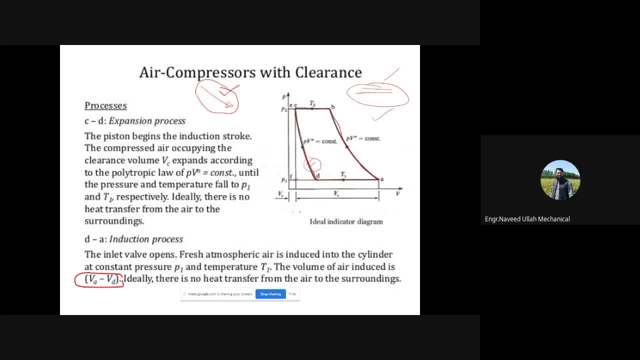 Here, you know initially it starts induction from here Okay, then you know this is a compression process B to C is the 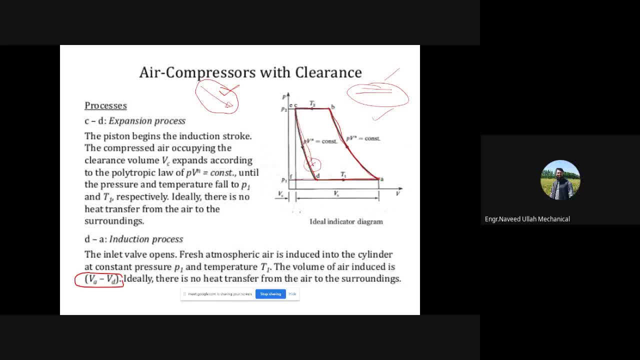 Expansion, sorry the delivery process and C to D is expansion process and again, you know, this is Induction compression delivery and expansion process. Okay now expansion process you have that is this compression and expansion They are polytropic in the first place. Okay, so yeah, what you need to do is if you want to find out the work consumed By the compressor to work consume media or under this curve 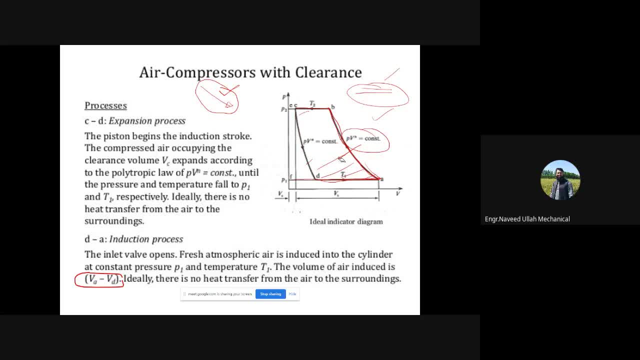 Okay, this will be a clear the work consumed by the compressor now you see here why this Bucky cheese, do I go? 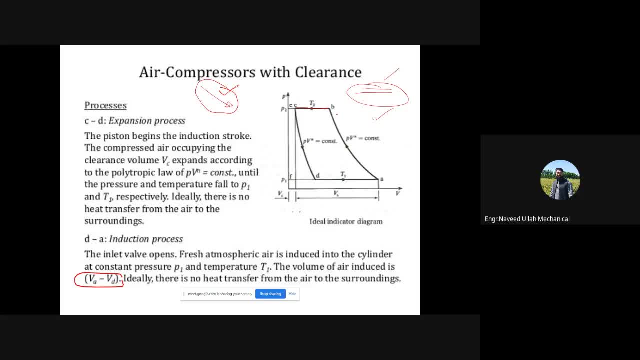 a compression case you Deliberate as you the a kiss pressure Cooper starter, but this new thing is about some expansion how this expansion takes place 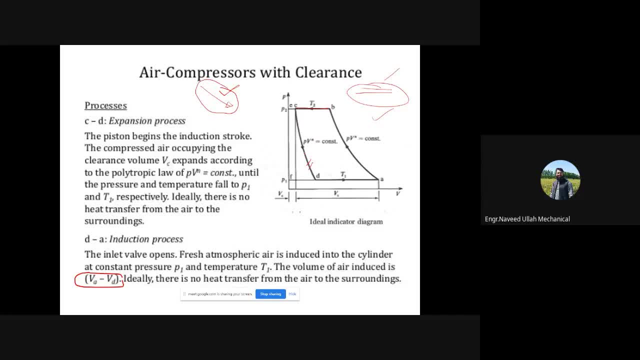 It is very simple, you know What happens is? 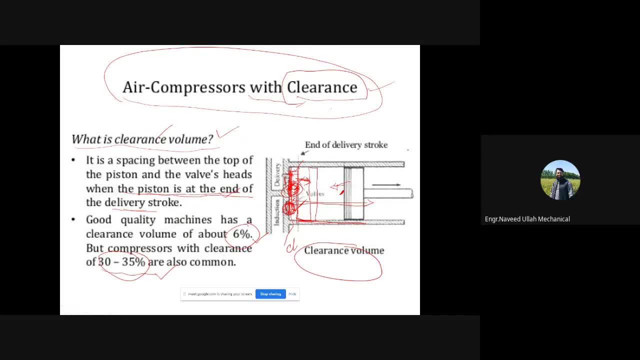 If you come here, right, let me rub this a little bit Okay, when the pissed when the you know piston is the delivery other compresses at The end of the delivery stroke. Okay, this one is at the end of the delivery stroke. Okay now it is start moving from here in the 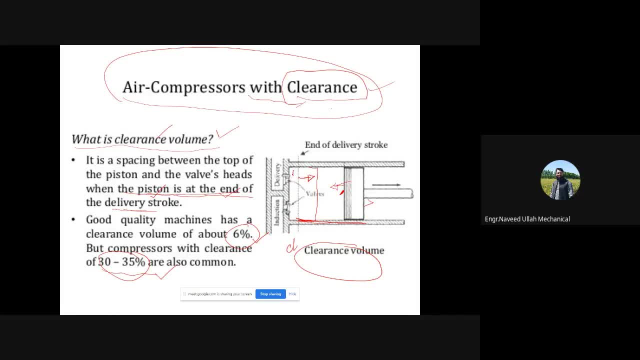 Rightward direction up. Yeah. Okay. Here we are having compressed air in the clearance volume Right compressed air in the clearance volume the moment it starts From this position in the rightward direction 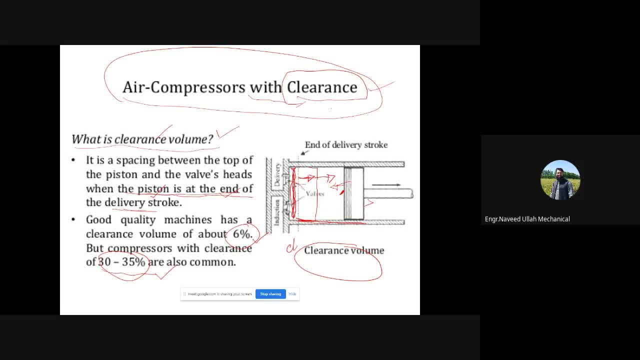 this pressure drops TK a pressure come over now why because volume is increasing volume increase yoga pressure will drop right 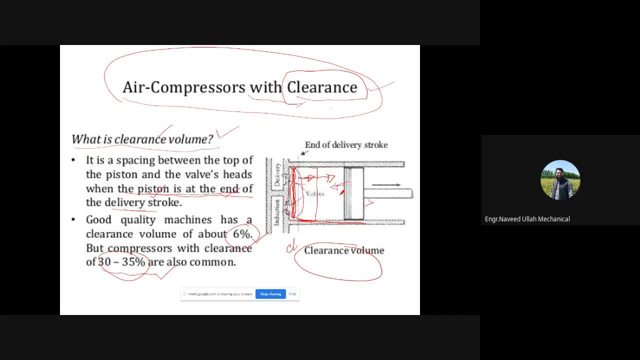 This pressure drop is basically your expansion process, which was not the case in the previous, you know 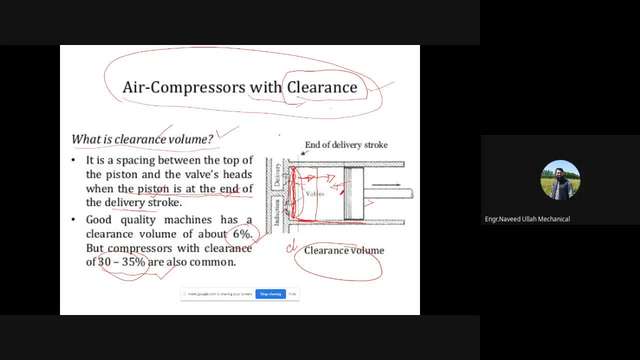 Scenario just me clearance volume Nita. Okay, I really do have induction Then we have compression and then delivery. That's it in the previous case, but in this case 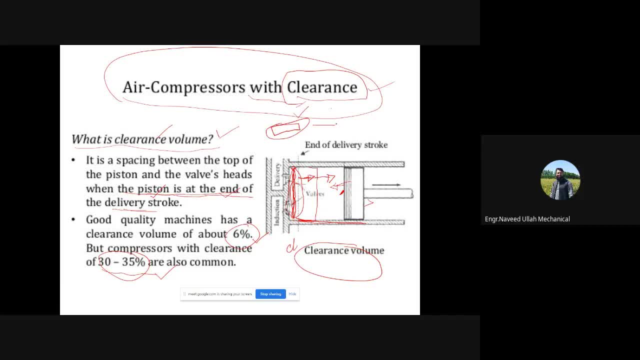 The moment the piston starts moving from the rightward direction. Sorry leftward direction To this right world What happens is that that compressed air? 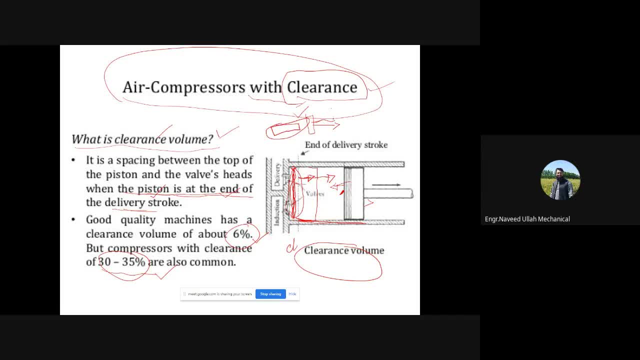 Is you know the pressure of that compressed air is it decreased? Why because the volume is now increased so the pressure will increase even if you have PV energy equal to constant PV game is equal to constant our PV is equal to constant in all the cases volume increases the pressure will decrease that decrease in 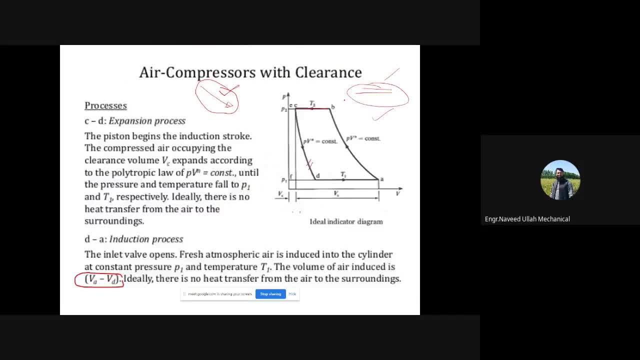 pressure is basically attributed as a expansion process It's because I'm a guy 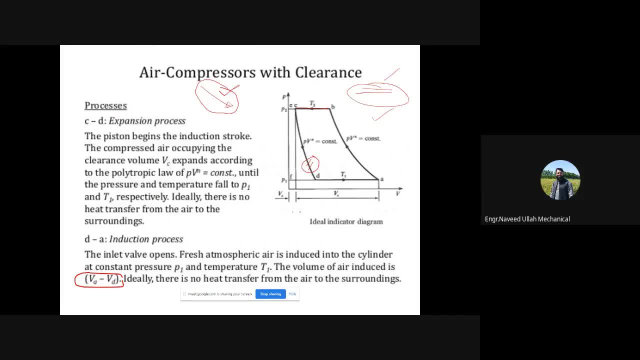 Expansion process is she's the same. Hey, let's go. I'm gonna ask you today. See today 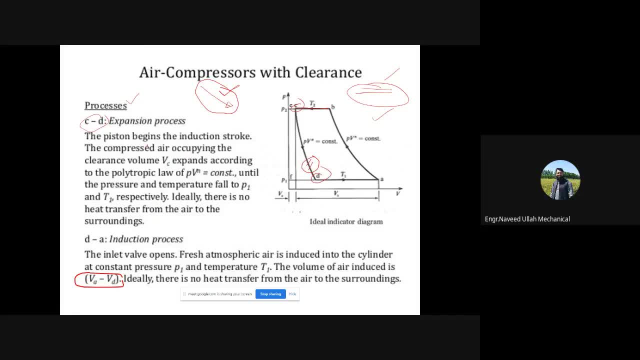 This is C and this is your D. That is what extension process the piston begins the induction stroke To get this is key and you per induction stroke start to start all time 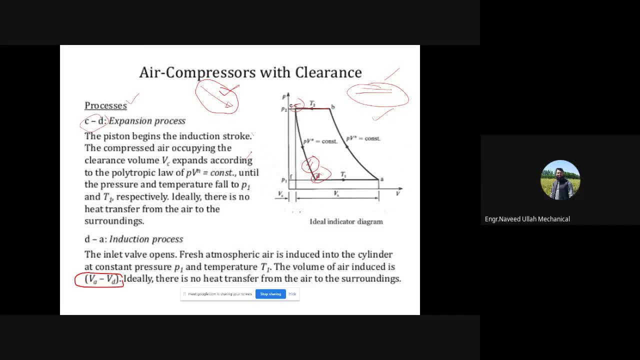 The compressed air occupying the clearance volume is the expense here to the political topic law TV energy will be a political expansion H until the pressure and temperature fall 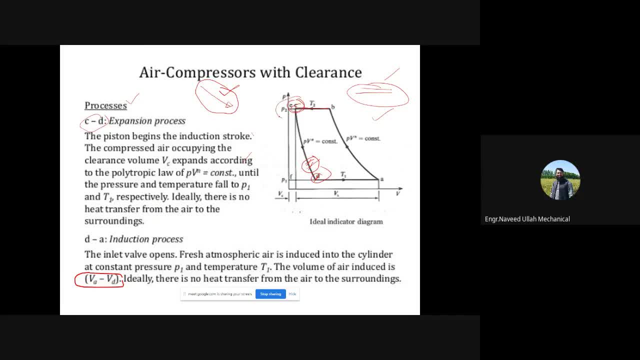 to P1 and T1 TK a pressure to have P2 T2 it and The expansion takes place the pressure drops right to P1 and T1 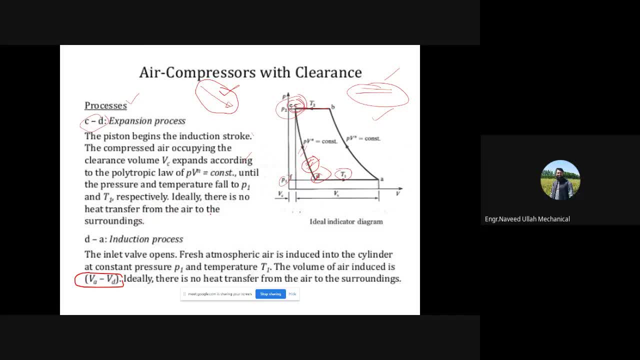 Right respectively. Ideally, there is no heat transfer from the air to the surrounding Induction process can 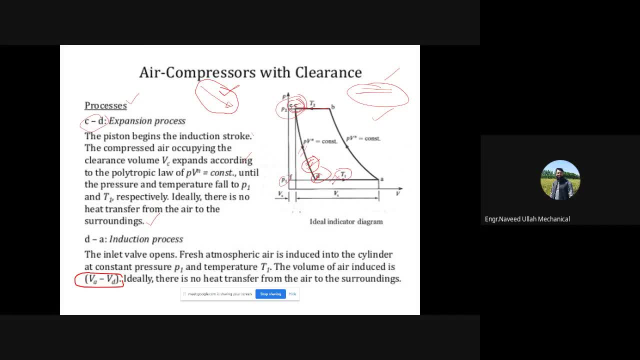 Induction process where he had to get again is my induction volume come over there 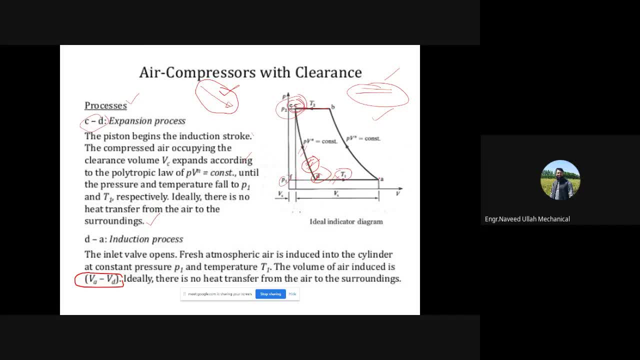 Gotcha, you can see previously we were having this much induction volume, right? So you can see here that? This is if this is let's say for example the total volume of the cylinder Let's say that is VT for example 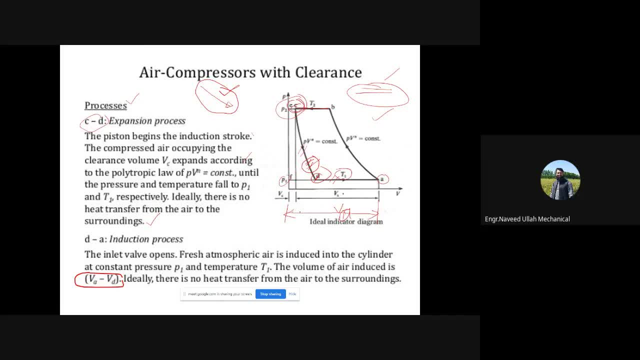 Yeah, we have this okay, so they because this is your VA so 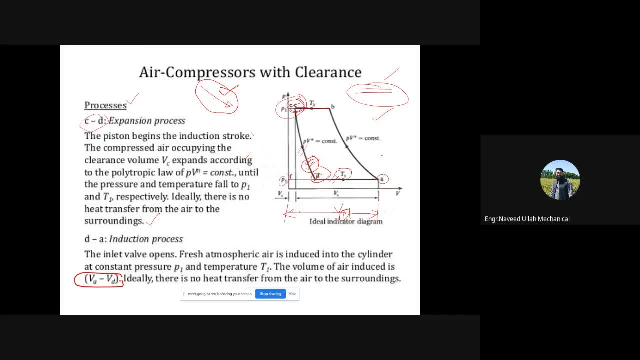 The volume that is swept to get swept up Is the sweeping new time sweeping? Is people this is actually stripped? right by this piston So yeah, I don't know yet. Yeah, I don't script 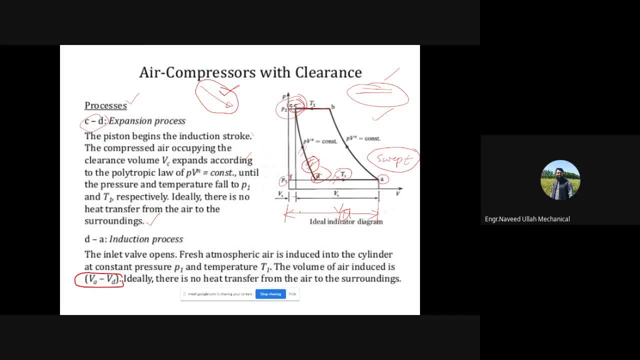 You cut the ITK fire the gun time is kill our you and your volume get the bucket at the end of that is work clearance volume So this is your sub volume and this work clearance volume. So we see is 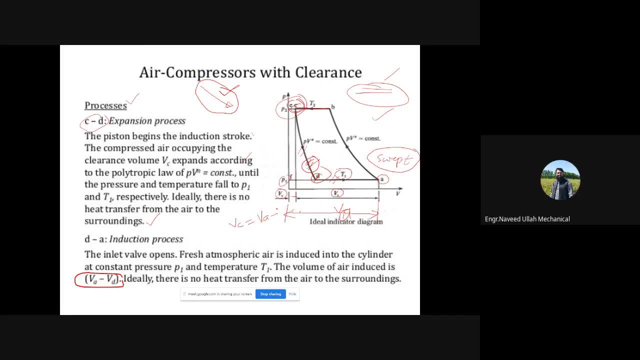 equal to the total volume we a minus swept volume TK are you can say that the total volume is equal to clearance volume plus a step value? 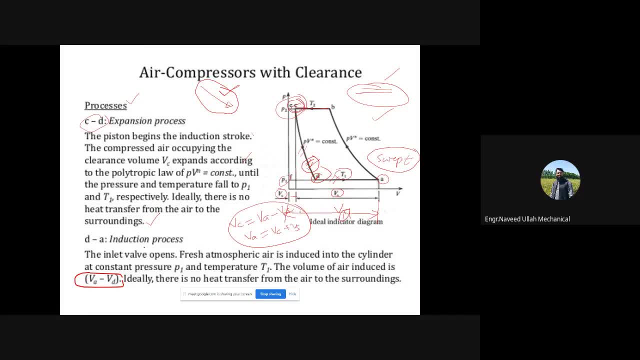 Take a year you and I'm the except a induction process previously I'm a repassion reduction kata induction was VA 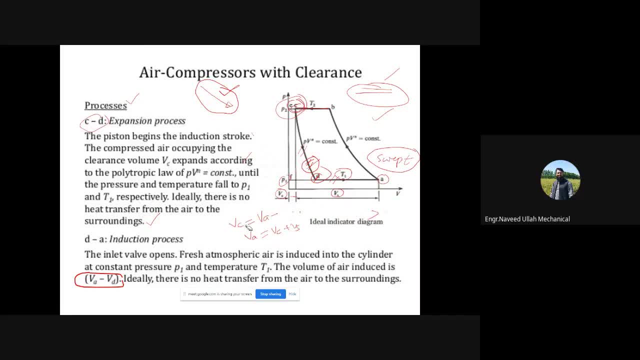 Okay Chitna yes, our value. You have any induced volume the abyss case may get a induction will be what induction is your this is your VA and 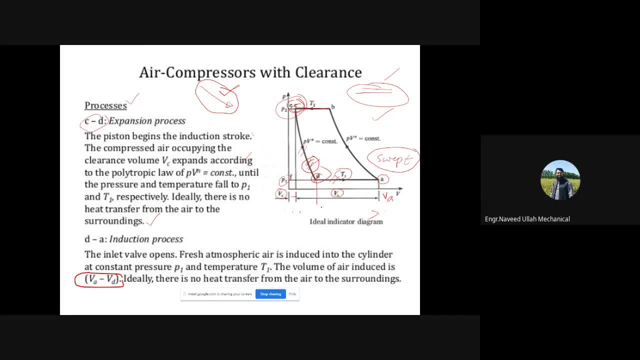 This is where is your VD this one? We need 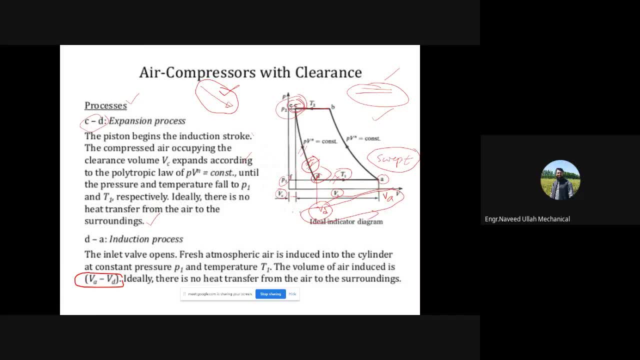 Because will be a minus VD is your induced volume now TK we a 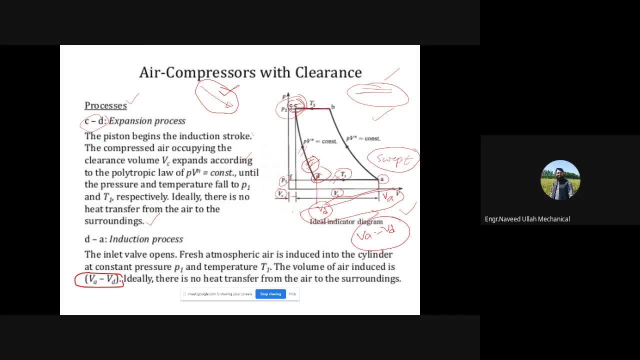 Minus VD this is your hand is the value of induced. Okay, so yeah, they clean the inlet wall opens fresh 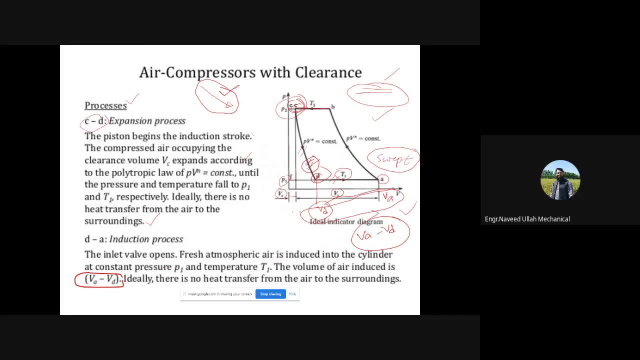 Here is induced into the cylinder at constant pressure p1 isobaric and temperature t1 So it not enough the volume of air induced is VA minus VD in this case 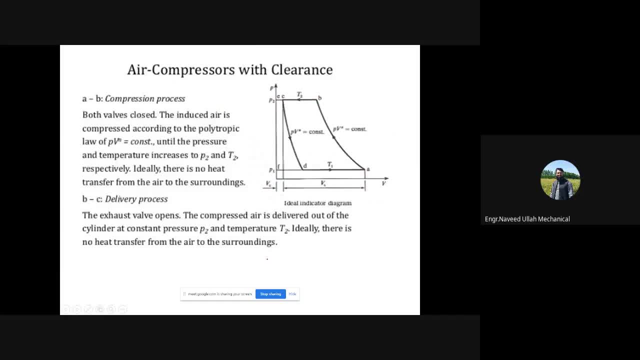 Ideally, there is no heat transfer from the surrounding your case. No time on a pass, right? Ideally there is but you know 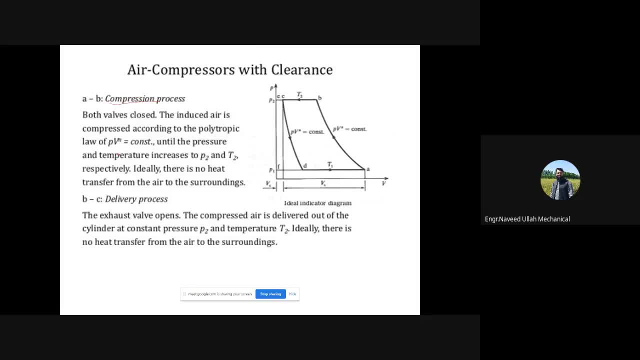 a little bit compression process will be up to pass a PVA is equal to constantly compression power delivery stroke. We will hear the pressure increases from 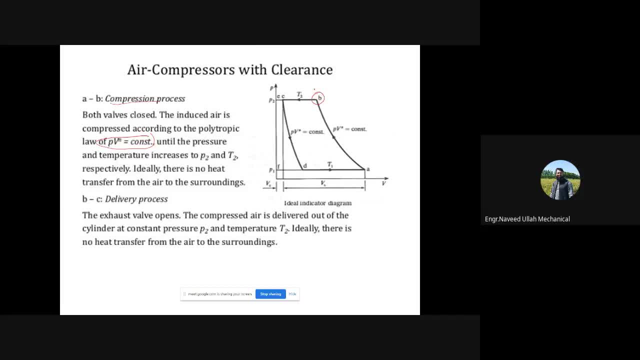 p1 to p2 Okay, and the wall will open and it will deliver that volume to you. You have to be better volume. We see yes, it's basically what? Previously I've to pass Joanna. This was a VB 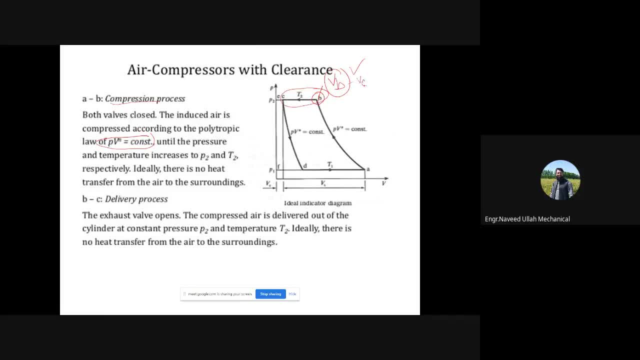 This is the delivered volume. Now. I was going to be my SPC will be the deliver value, right? What I'll just put it up for the next thing right now 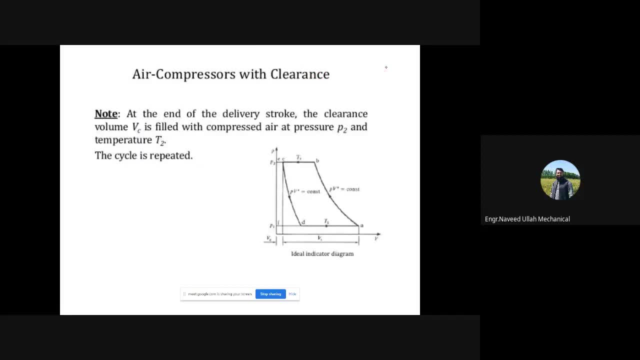 It's for discuss care care here compressor with clearance So they are saying that at the end of the delivery stroke Clearance volume we see is filled with compressed air at pressure p2 and temperature t2. The cycle is repeated, right? So 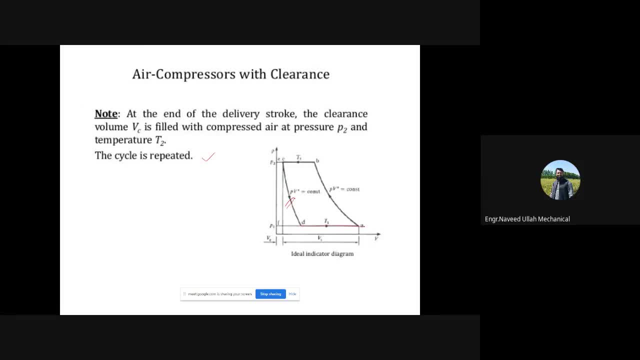 expansion takes place and then induction takes place and the induction volume will be your VA minus VD 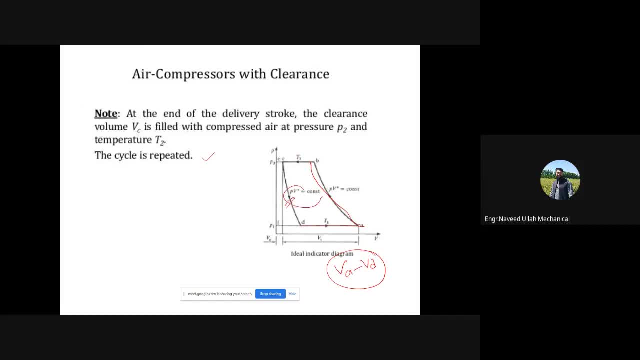 Then compression takes place for the topic compression This is also for the topic expansion through topic compression induction and it will be the delivery and it repeat itself if it's okay, I Am a Gap, if you remember how many we bought the DK, I'm a repulsed. Yeah 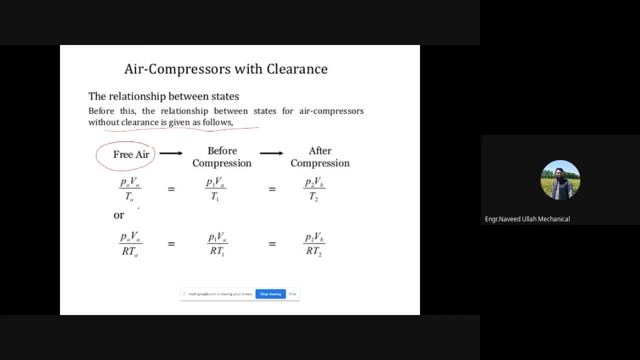 Do you previous this free here? Hey, we not we not by t naught TK. Yeah 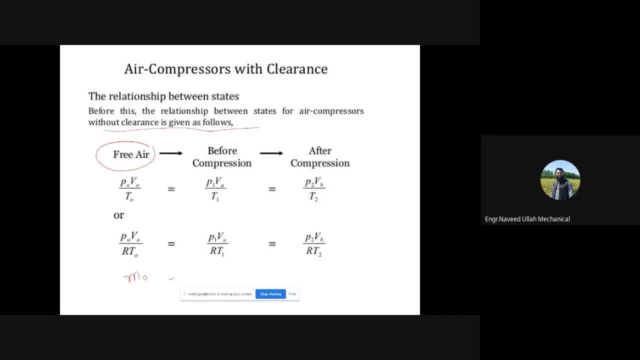 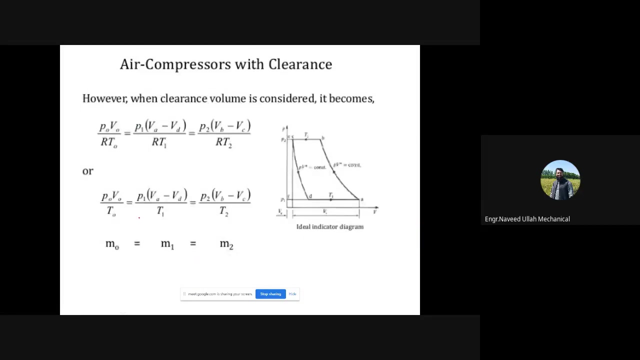 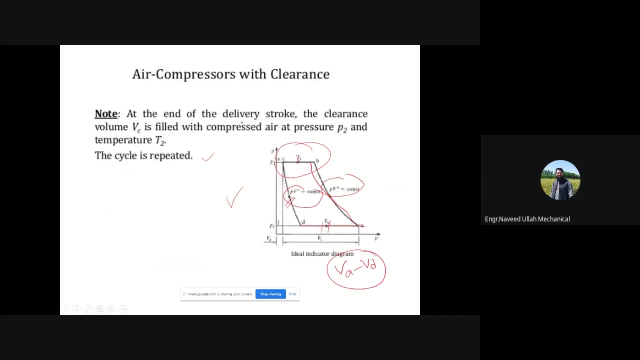 This is basically we want to show that this is M naught This is your m1 muscular rate is a constant. So how to to have these mass flow rate is constant because pb is equal to m r t so m is equal to pb over rt right pb is equal to rt okay so here you can see that p naught p naught will be rt naught p1 this is the previous case remember without clearance p1 va rt1 p2 vb rt2 this this was for you know without clearance with clear is the same thing but you know free here the same one right but here same thing this is p1 by rt1 but what is the induced volume va minus vd this is p2 by rt2 the same what is the delivered volume that is your vb minus vc previously this whole volume was delivered volume this one from here to here this is vb vb is the delivered volume now we have actually a clearance volume over here 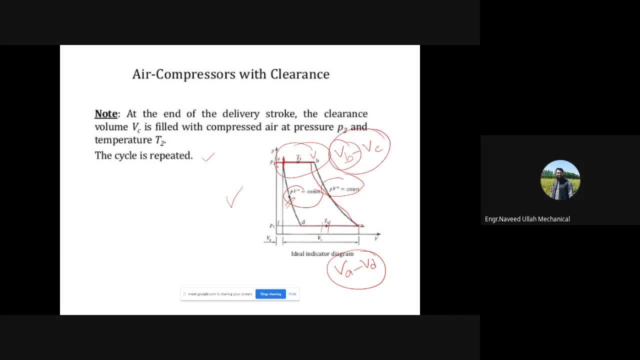 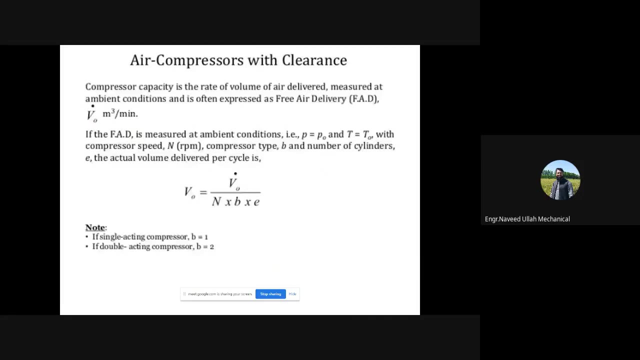 so vb minus volume at c okay this is your you know delivered volume okay so this change comes to you anyways um then they are talking about the compressor capacity 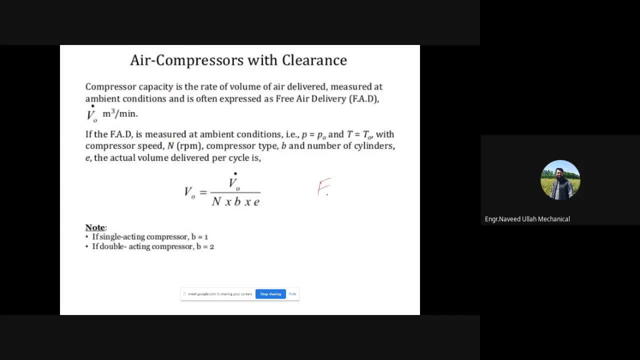 about the compression capacity of the wind 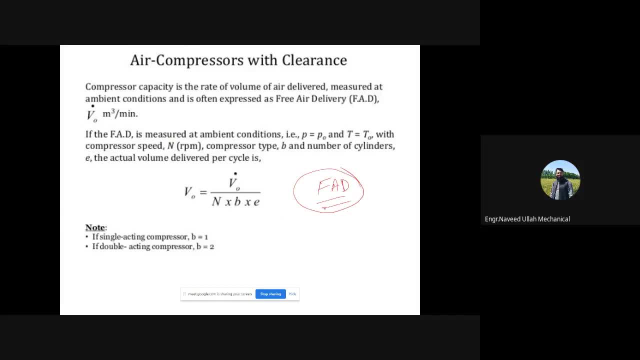 so obviously if this happens it is hundred times more efficient than you should not consume so you will not��ʿ~~ 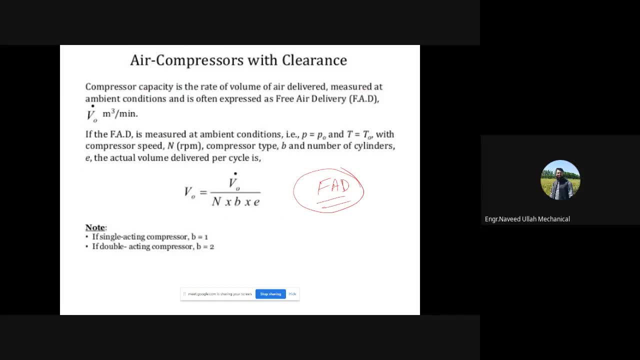 p rate but it is measured at ambient conditions okay and is often expressed as free air delivery so basically this is volumetric flow rate but if you see here there is a not here okay it is measured at free air condition if you remember 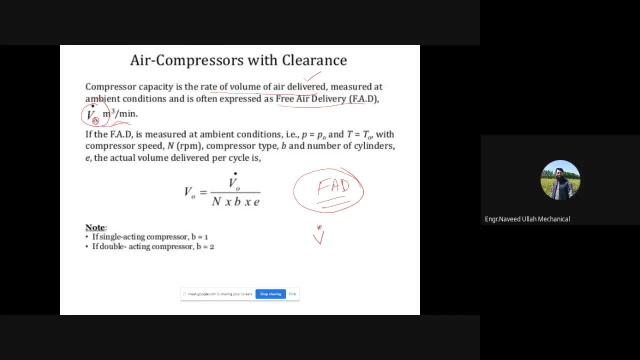 this is the delivered volume uh sorry dot and you are measuring ticket 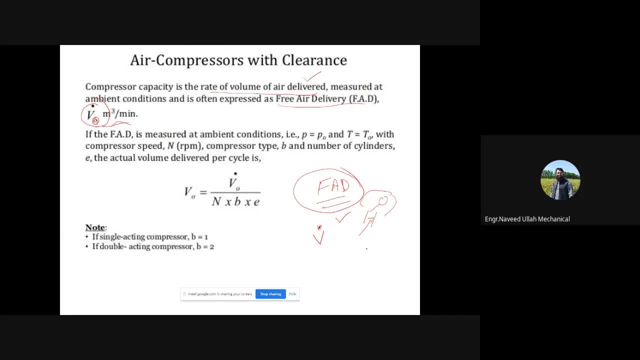 are measuring this in vacuum that will be different a bit different okay but it will be a bit different right because you are measuring it in the vacuum similarly if you are measuring it 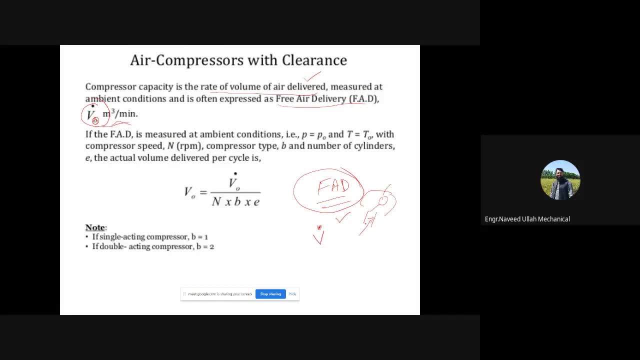 against higher pressure it will be different but if you are measuring this volume okay the volume delivered by the compressor it ambient temperature and pressure if ad so this is actually volumetric flow rate in cubic meter per minute but measured at a ambient condition ambient temperature and pressure 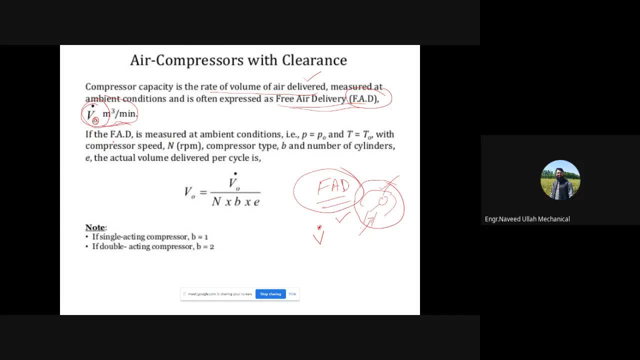 and it depends on you know different things so if the fad is measured at ambient condition t is equal to p not free ambient pressure and temperature with compressor speed it depends on compressor speed it depends on the piston type sorry compressor type it is it is single acting double acting and also it depends on the number of cylinders okay to increasing 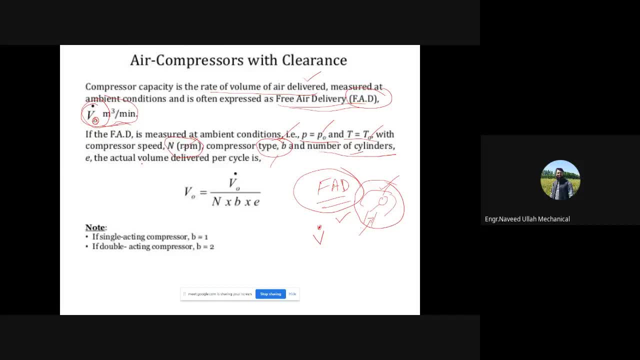 if you encounter these things and you want to calculate the actual volume delivered per cycle that will be the fad divided by rpm compressor speed multiplied by e multiplied multiplied by b that is the compression speed. 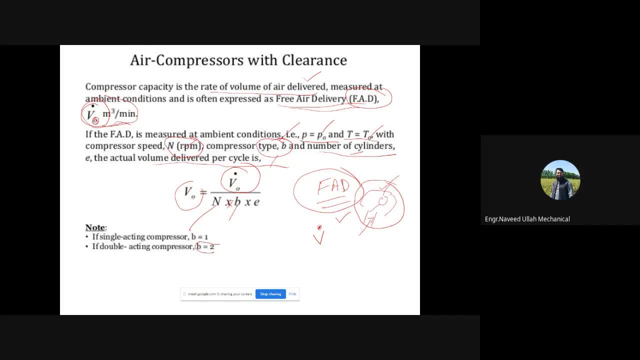 compressor type single acting here so in place of b you can put two sorry double acting other single acting here you can put one in place of b and similarly this e is for uh number of cylinders so this you know you if you know about you know this uh if ad if you know about the rpm you know about this uh type of air compressor and you know about the number of cylinders you can calculate actually how much air will be delivered okay which is then analysis of the cycle 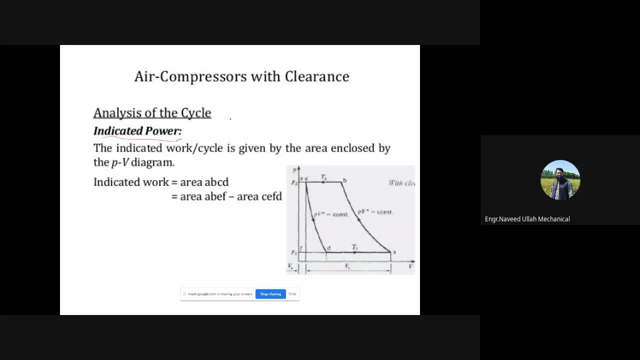 in the same way in the same fashion you need to find out the indicated power okay for the case with clearance volume 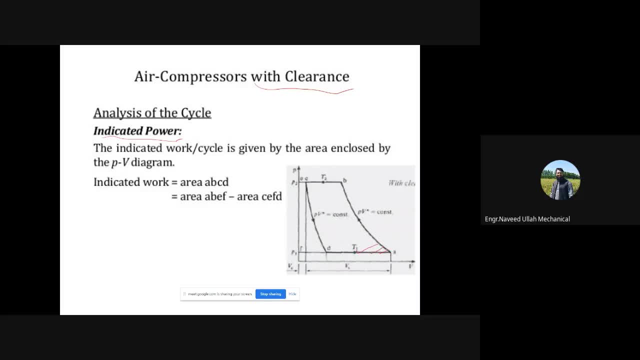 there is even no need to explain this you need to find out the area under the curve for this pv diagram that's it because previously different 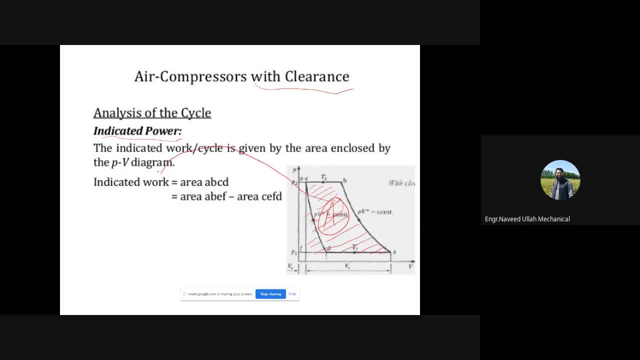 you need to find out this area this area under the curve is your what indicated work area a b c d a b c and d how to calculate this area a b e f a b e e h 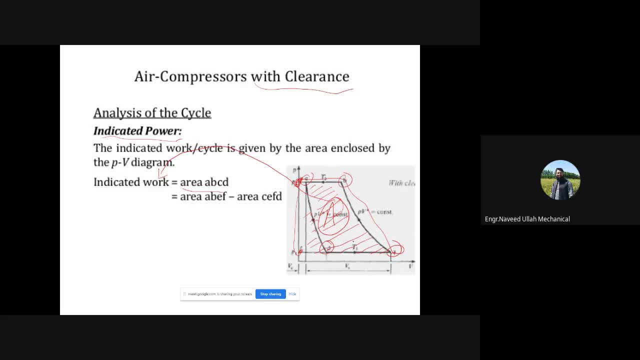 this is a period of analyses in this area has to be found out from a к c fixation look again ann you see this here area this one area here so if this area. 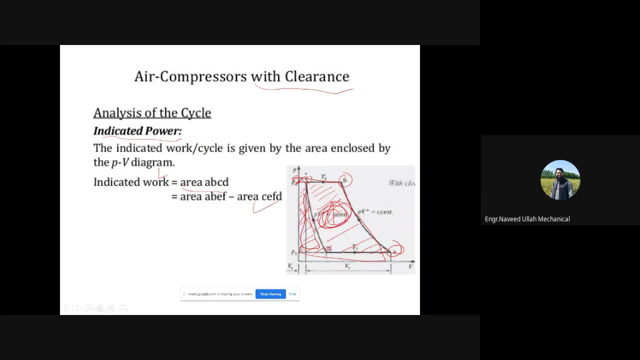 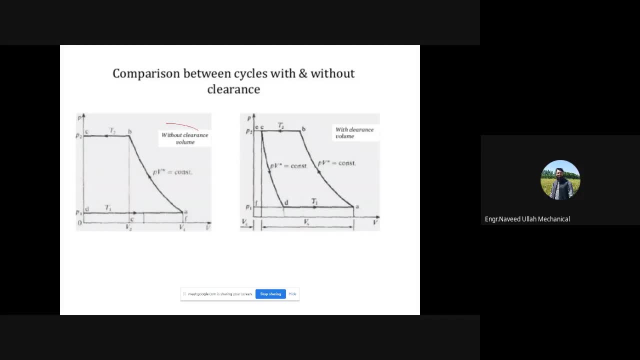 sa you can see induction volume this is the polytropic compression and this is polytropic compression this was the delivered volume and this one is now the delivered volume is this one 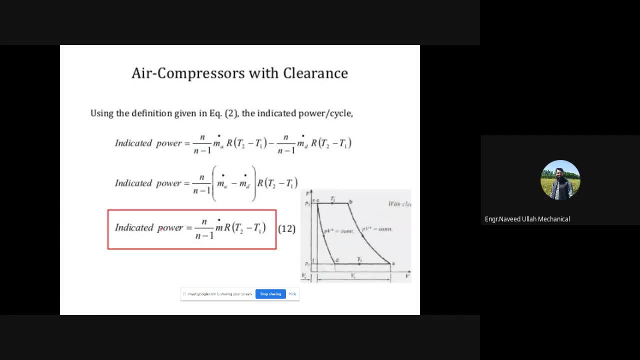 okay uh you know very well but just i'm uh let me tell you that indicated power will be equal to from that diagram n by n minus one m dot r t two minus t one relationship where you can find out the indicated power okay actually m is basically your mass flow rate at a and mass flow rate at t 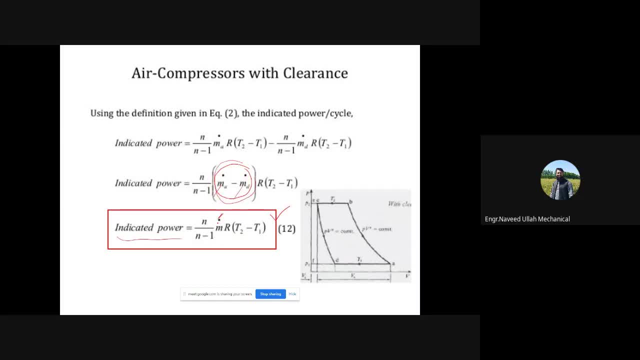 i should write it like this because but here i should write it m dot bar where m dot bar is basically what in this one 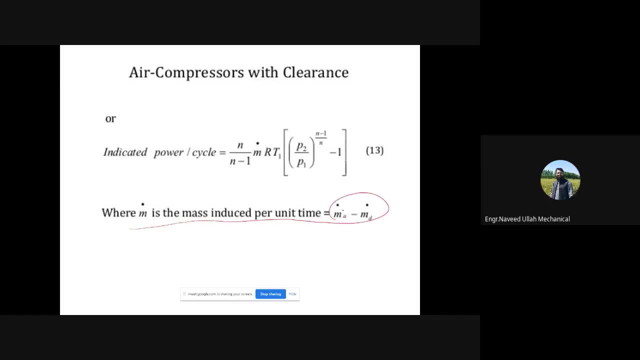 m dot bar is basically the induced mass so unit time or this is actually if you want to find out how to make it you can also get that diet and you get the幹嘛 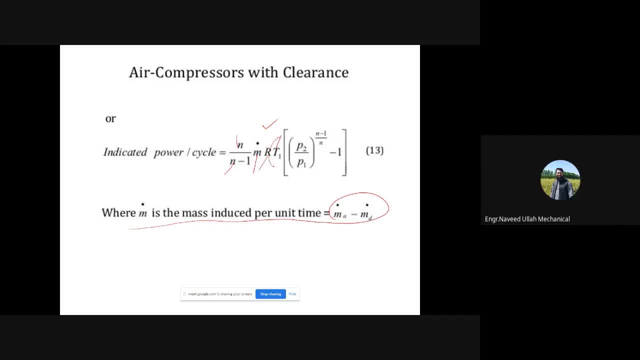 mass flow rate that you have induced r is constant t1 is the initial temperature you need to know about this and you need to find you you need to know about the pressure ratio this is basically the requirement how much pressure did you require how much n dam we need so if you know about all these things just know that we need the decision ratio a lot of times so if you know about all these things you know a lot. 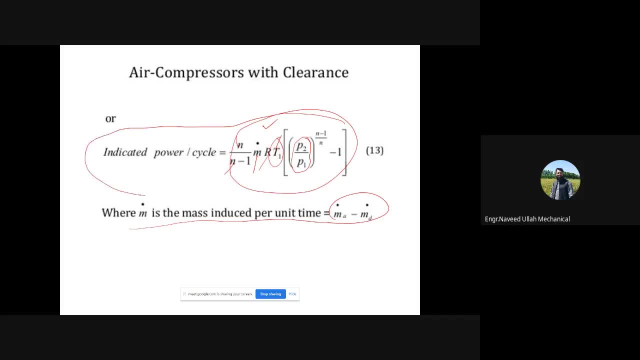 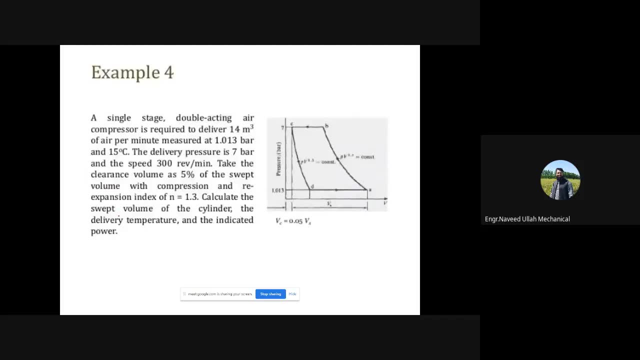 these things you can find out that how much indicated power per cycle will be consumed right and from here you can even select the motor for this right okay three years people do an example for him a single stage of double acting single stage here okay double listing here your compressor is required to deliver this much volume okay for a minute to measure later this actually a decade now this is a very sick because it is measured Edward it's not very pressure okay ambient head for this keeper we have given head the deliver delivery pressure is seven please come at the week is seven by one point zero one three this is actually your pressure ratio p2 by p1 and the speed is 300 rpm and take the greatest volume is five percent of the swept volume at a to swim volume did not keep us in a house car 0.5 up language you have capacity as a clearance volume on the other of the sweep volume with compression and decompression index a polytrophic index about car right in is 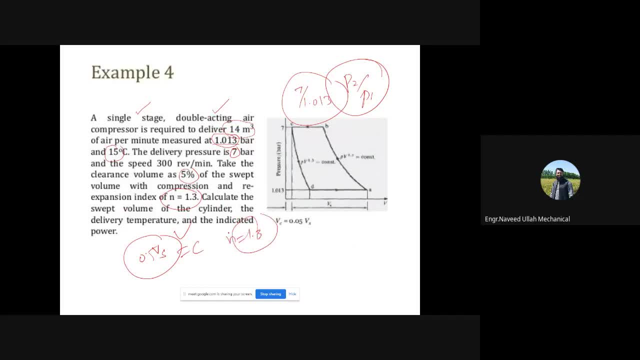 equal to one point three right calculate the strip while you play up mr. Paul you find out Karna hey take care of the cylinder and the delivery temperature T to operate find out Karna has and the indicated power and may do you have to pass it okay this is indicated power yeah 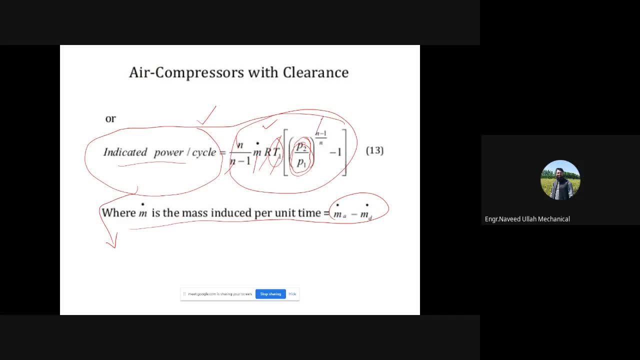 so t1 of the pass hey p2 by p1 of the pass a in up a pass hey and maybe good she is to have t1 and 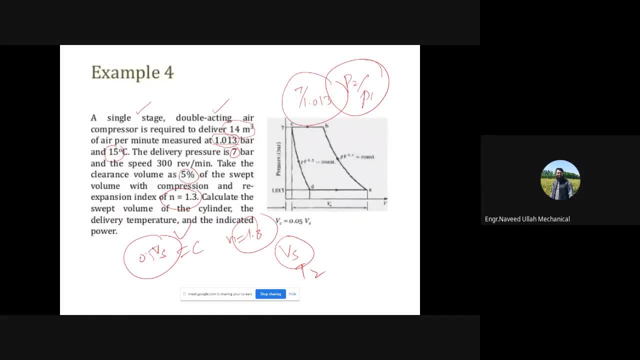 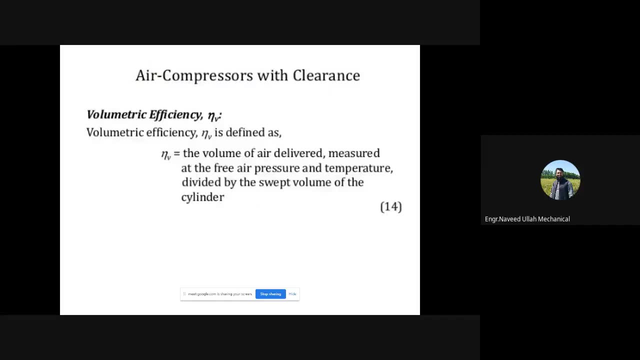 find out to a point of her name yeah for future nature this is for example based on the simple relevant formulas 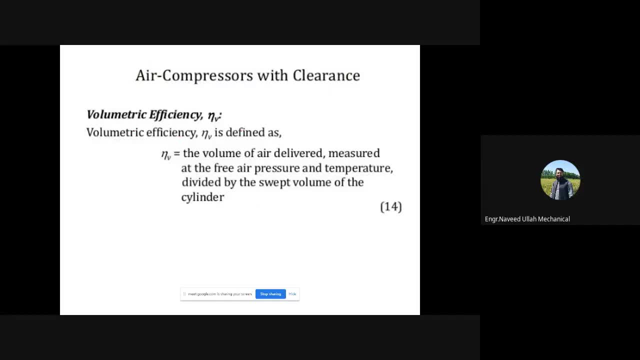 volumetric efficiency is defined as the volume of air delivered kids now I do deliver cut the head measure is the free air pressure and temperature divided by the stress volume of the cylinder it's not only a deliver 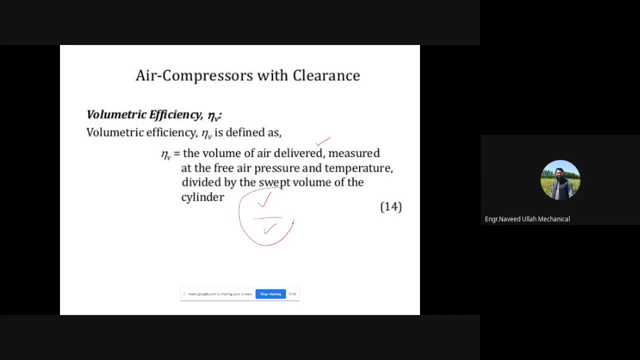 cut the hair or get not really a sweep cut the hair in a leakage is to basically what you make the efficiency leakage in counter cut the TK it miss kidna sweep your volume go okay how much while volume is stripped how much volume is stripped and how much it is delivered okay so in this major ratio head that is 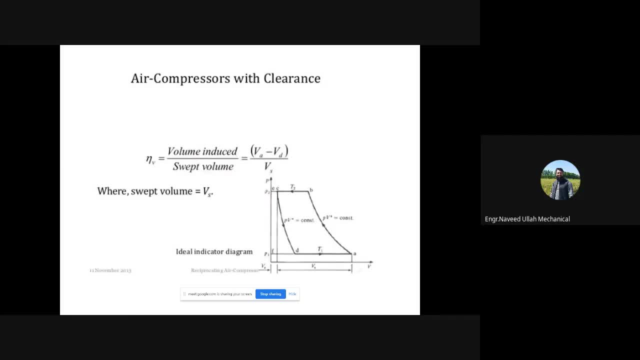 known as volumetric efficiency basically leakages go back to easy to kiss and keep our money I don't listen to Rico say I'm so curious okay take the 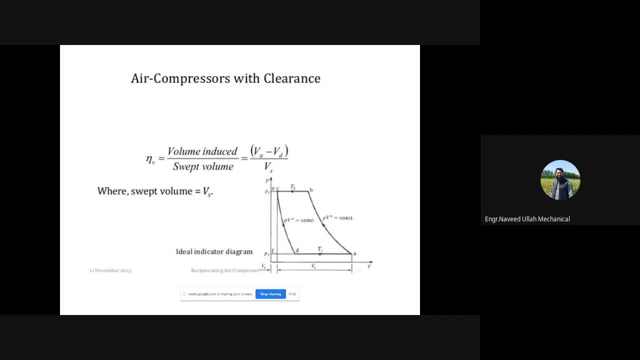 whole head volume delivered by a stir volume or do so I don't have volume induced based upon you give me up yesterday okay so volume induced you can 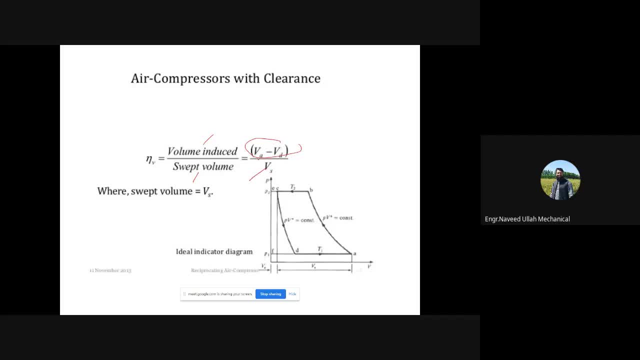 heavy a minus B D divided by strip volume right I tell you we strip volume 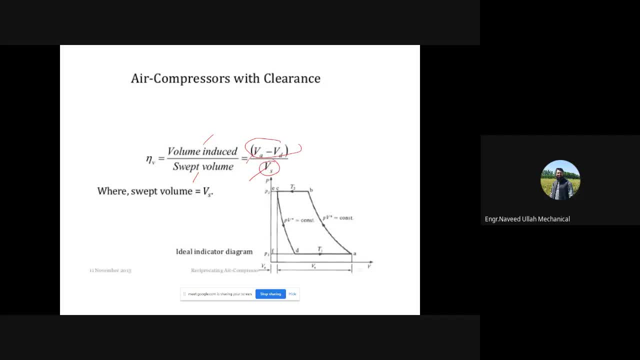 co or deliver volume go to Hannah sorry this 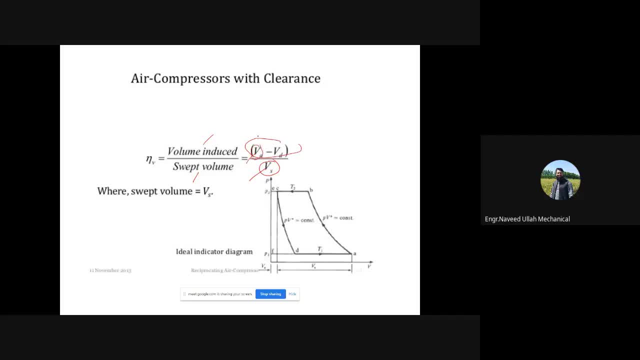 what should I say this total volume go to Hannah hum find her cussing are risking to have woman affection go pataki by total volume of the cylinder it nahi two manager Hannah with clearance it need a key head to slip volume you know a Mariposa calculate concept a point six percent of the total volume yeah as you 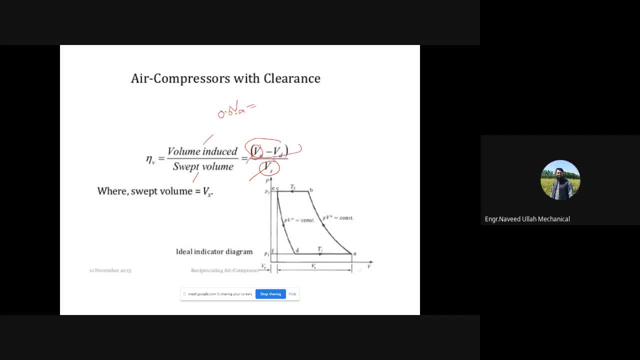 do a makes clear this volume our USA I JGK it's a were six percent clearance but this will be your clearance volume now you will total volume minus plus 5% clearance 3.5% so this will be your clearance volume now you will total value minus 6% clearance 3.5% this will be your clearance value now you will total volume minus 6% clearance 3.5% now you total value minus 6% clearance 3.5% 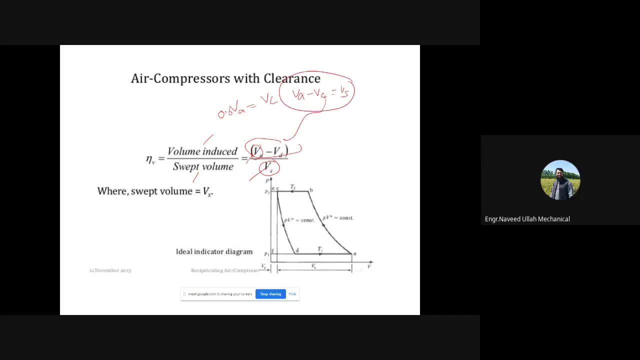 your clearance volume will be your step volume so you can calculate your step volume similarly this is the total volume of the cylinder okay 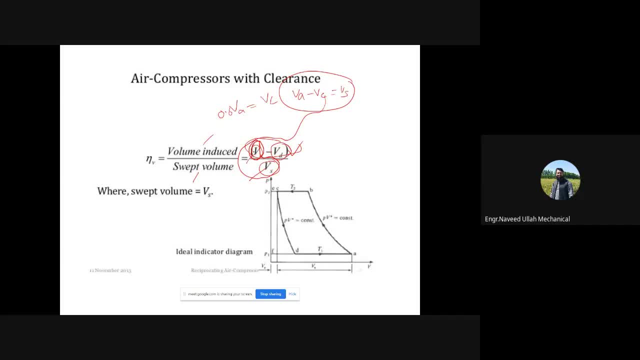 so you can use readily this formula to find out the volumetric efficiency the volume the value of the volume here 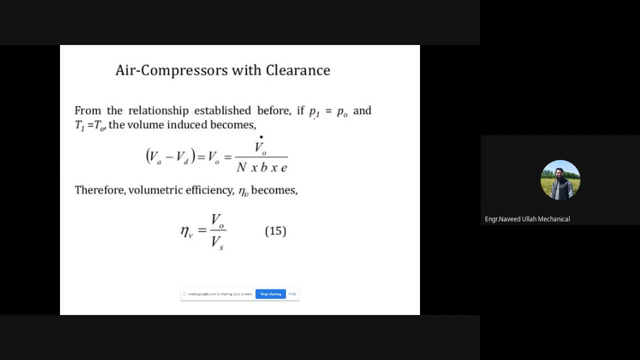 anyway from the relationship established before if i got a pass p1 or peanut the compression process is the same and the pressure is also the same so the volume induced will be this this is the volume induced okay and that will be equal to this 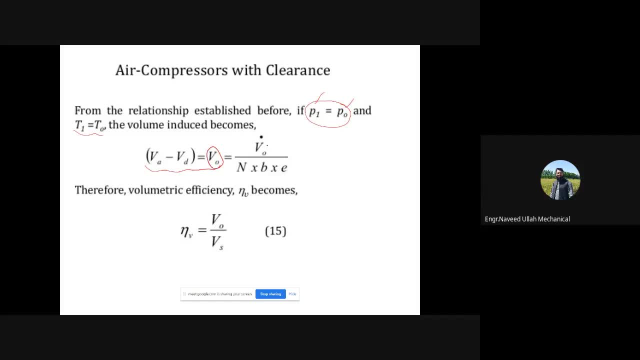 v naught okay or actually we not or actually we not when our past cc's it is influenced by these three things okay therefore 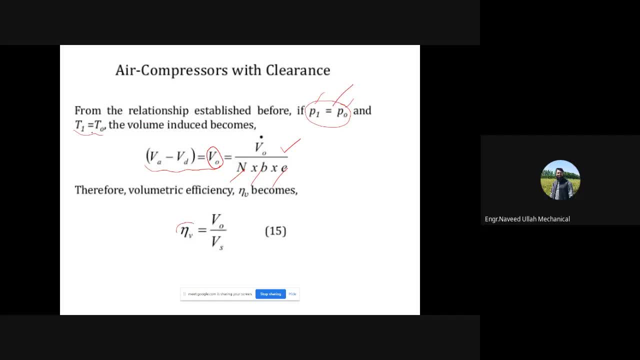 for this assumption where p1 is equal to p naught and t1 is equal to t naught 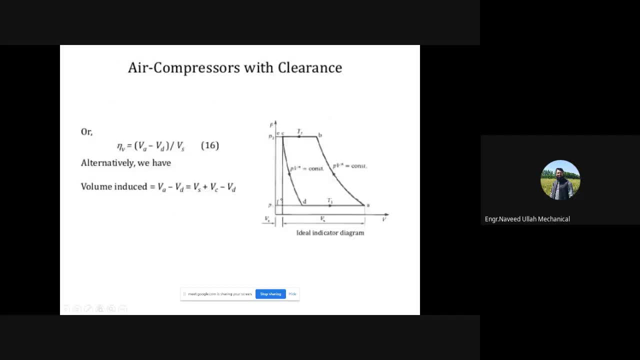 this is one of the relationships okay similarly another relationship is you can see that volumetric efficiency is equal to this v a minus vd induced volume by store volume and induced volume you can see that this is v a and got to all the 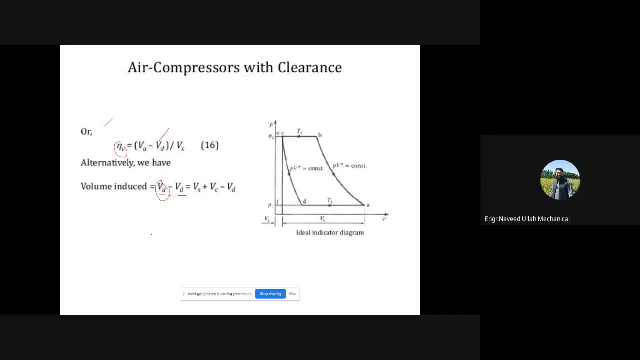 versus so minus vd what is your v a let meúa 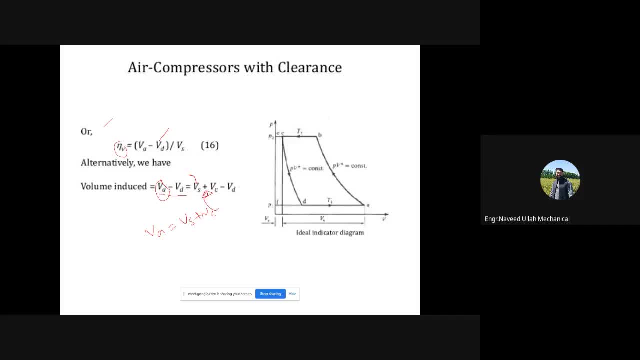 yeah that is actually the edition of suffering plus a clearance volume plus clearance volume so volume is with you okay and then uh further if you remember previously you can relate volume ratio to pressure ratio for polytrophic process okay if you remember previous so vd by vc is equal to p2 by p1 1 over n vd is equal to this thing now you see that we know about polytrophic index we know about our required pressure ratio we know about the clearance volume so all these things at right side they are actually known quantity this means that you can find out the value of vd okay so uh it is difficult to find out this v a and v s is simple but to find out vd is difficult so for that reason we have actually converted 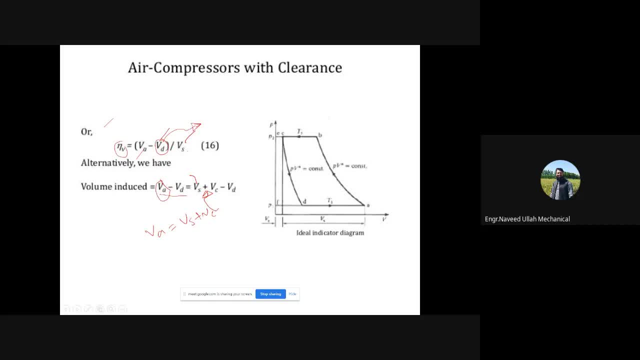 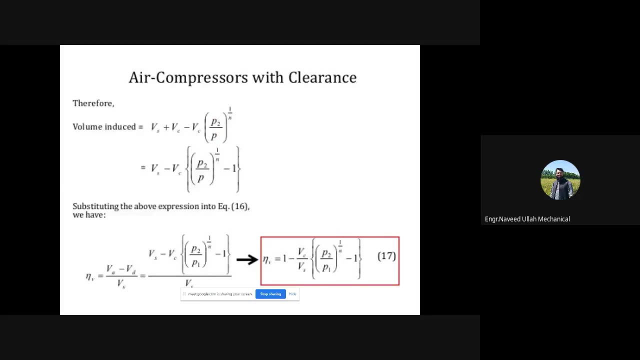 uh we have actually alternate you know what should i say and directly find out the value of this vd using this relationship you can find out the value of vd and then you know putting it over there ultimately 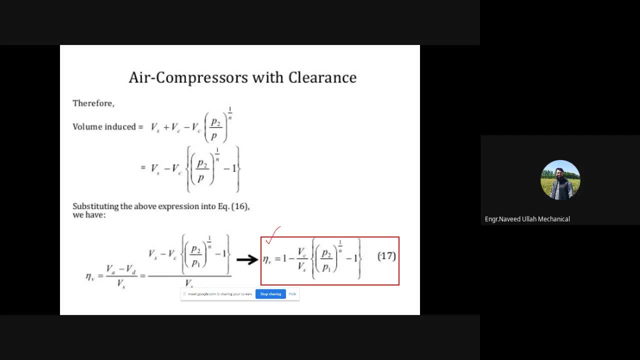 you will see that the volumetric efficiency another formula okay that is one minus vc by v s both are either measured measurable are calculated easily and this is pressure levels only and these are not charged in the form of G vivos and so you can find out value of volumetric efficiency right there is an example five and that is 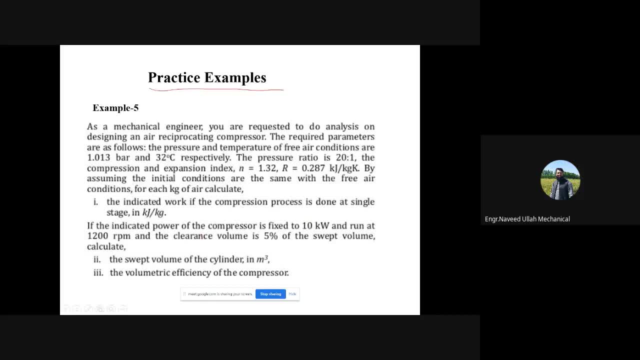 actually your practice example of the uh solved example 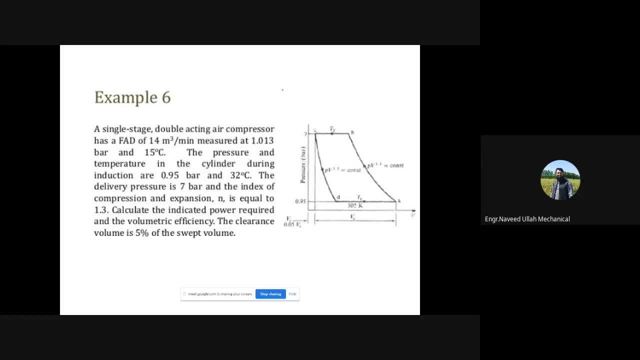 right okay example six is also there you can have the data from there and you can find out 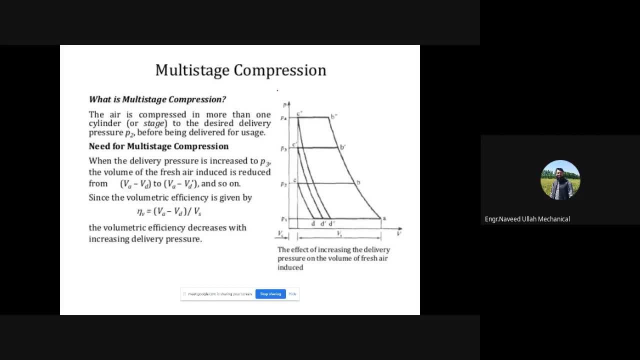 okay now discussing um the ear compressor it's cutting ear compressor with clearance volume we can also we are now in a position to discuss the multi-stage compression so let me explain this uh with the pb diagram you see here why we need multi-stage compression 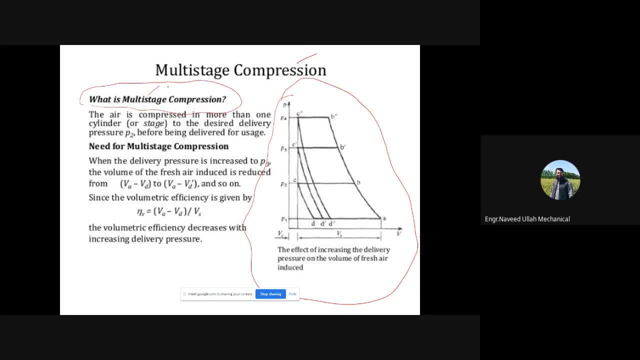 multi means more than one right so you see here that if you are using a single cylinder okay it will cost you let's say x and if you are using three cylinders it will cost you y and obviously y will be greater than x so you are actually spending money on extra cylinders that's it okay uh you are using equity for having three stage uh ear compression you are using you know various um and more than one cylinders okay and more than one stages so it will cost you okay how you can justify this cost or how this process of multi-staging is cost effective again 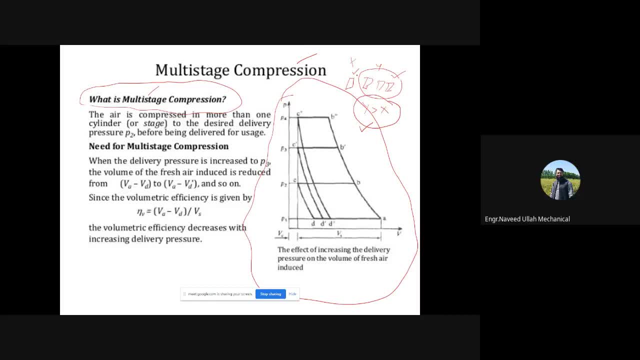 is you know let's say this pressure ratio is x bar now if you want to achieve this pressure ratio using a single cylinder a single you 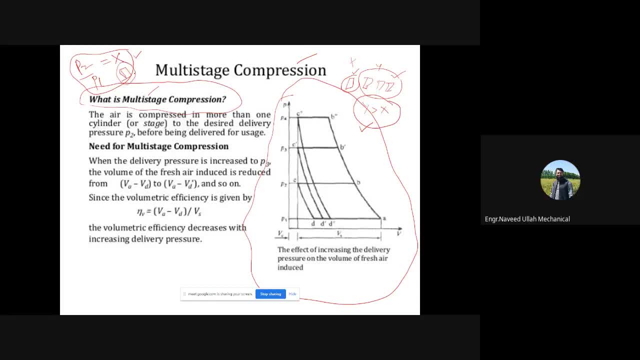 know stage is advocating ear compressor what will be the limit is p2 by p1 so then with that said 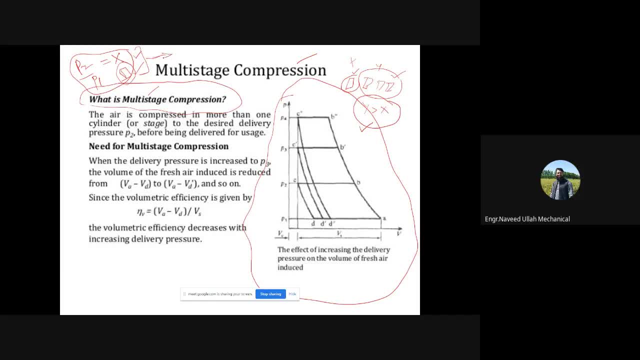 Meditations and drawbacks Okay that you are flipping from using the single stage to two three or four stage reciprocating air compressor But somebody 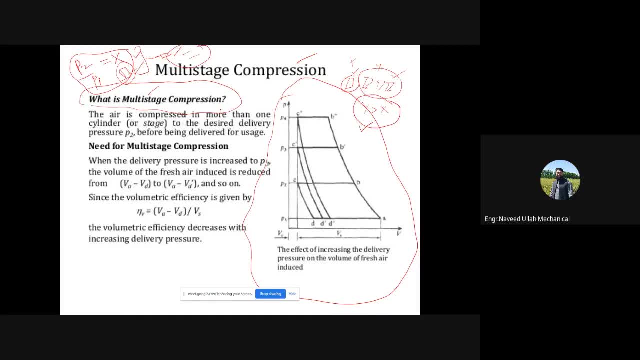 To this key reason honey change. Oh, yeah, I'll be up They clean subsequently back to kiya. Hey if you see here 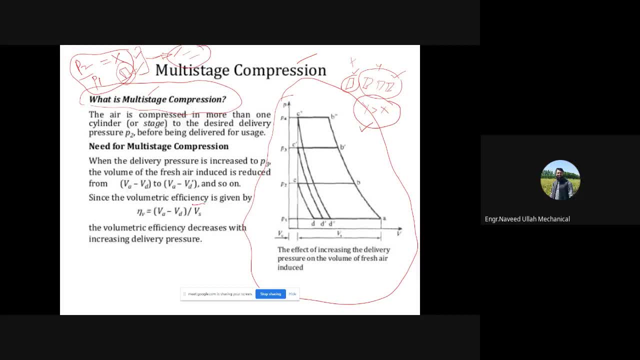 Yeah, I'm just pointing out the important things I 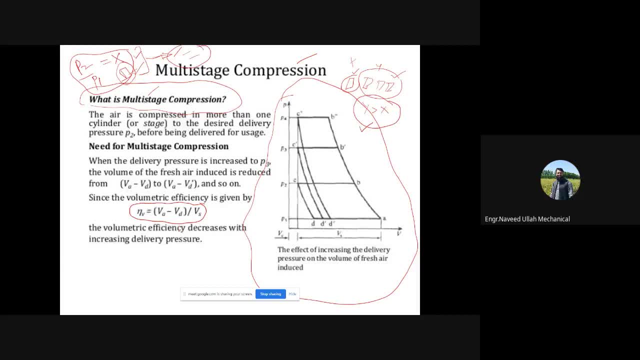 like it if you want to increase the pressure ratio up Great 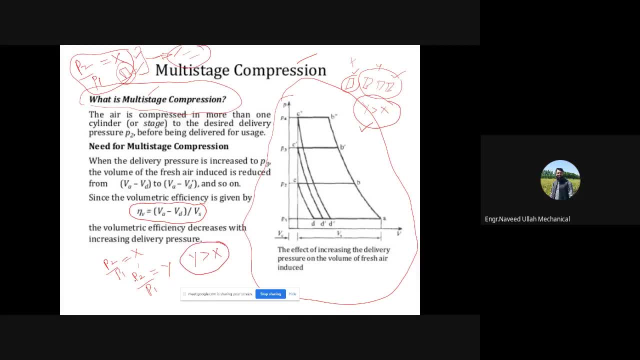 See case then I Want even more pressure , then this? one 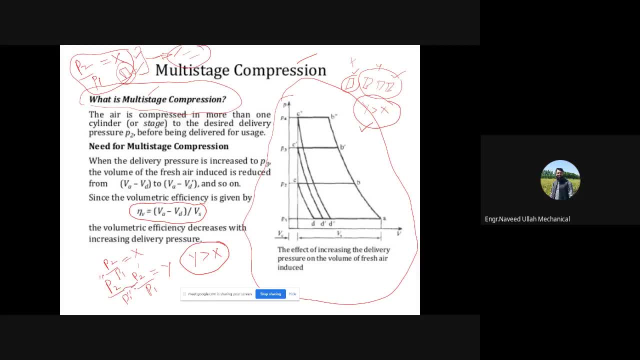 let's say p2 double bar by p1 double bar r prime this is your z and this z is greater than y is greater than x okay so you want more and more pressure ratio and if you are using the single stage compressor what will be the limitation in tropic and hazards okay and then you will flip that actually you know compares you to flip or to use the multi-stage cylinders 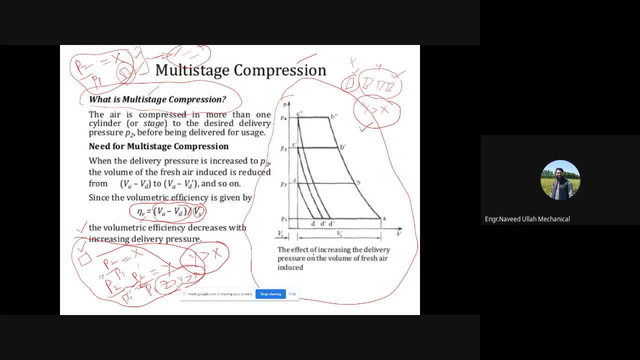 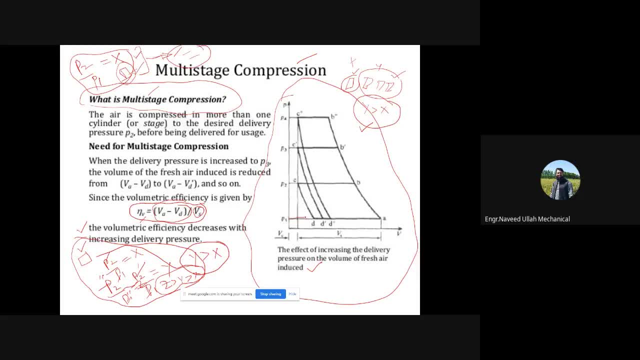 so if you see here in this first case this is basically where you see um d a is the induced value this is your vd this is your v a and we will be having v v a and we will be having v d that is what that is here the induced volume so volume is the same let's say 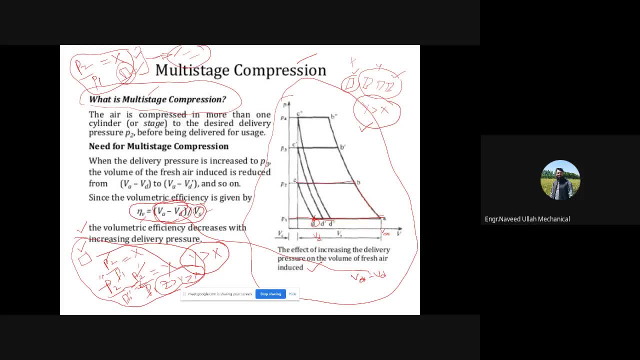 now so this is actually compression and then it is uh delivery and this one is expansion for this first case if you want to in if you don't want this p2 rather you want p3 or p2 bar 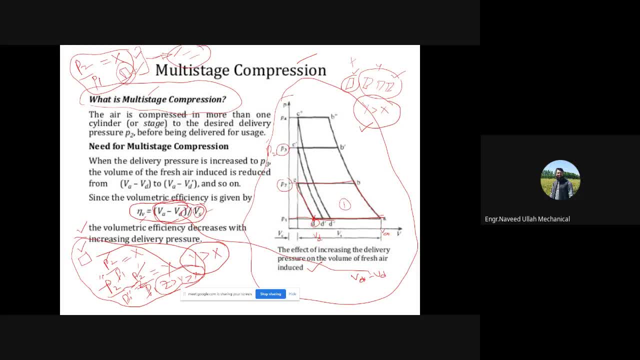 this is your you know let's say induction this is your you know let's say induction initially initially and this will be your compression this is and this will be your compression this is and this will be your compression this is your delivery and again this is your your delivery and again this is your 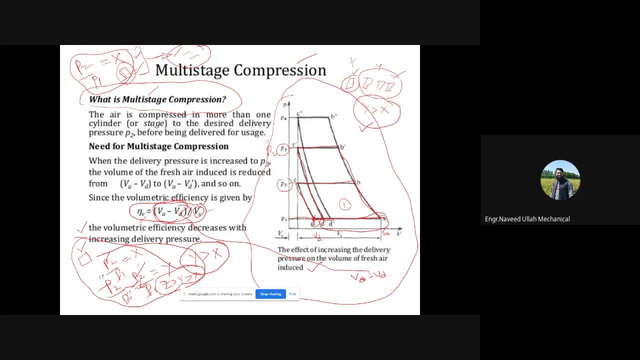 your delivery and again this is your expansion now you can see that expansion now you can see that expansion now you can see that this time your induced volume is d bar this time your induced volume is d bar this time your induced volume is d bar minus d a minus d a minus d a okay so your induced volume decreases okay so your induced volume decreases okay so your induced volume decreases again again again if you are further increasing this you if you are further increasing this you if you are further increasing this you want this more pressure dk pressure ratio want this more pressure dk pressure ratio want this more pressure dk pressure ratio so this will be your 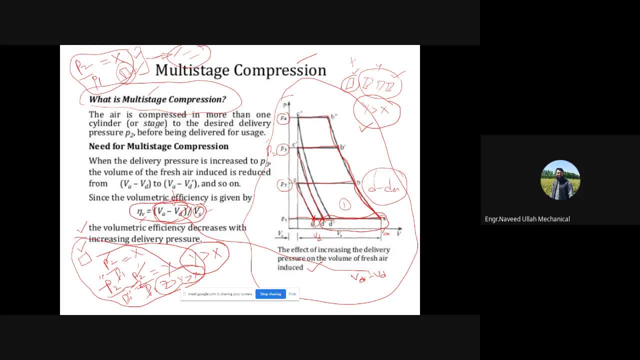 so this will be your so this will be your compression process this is delivery compression process this is delivery 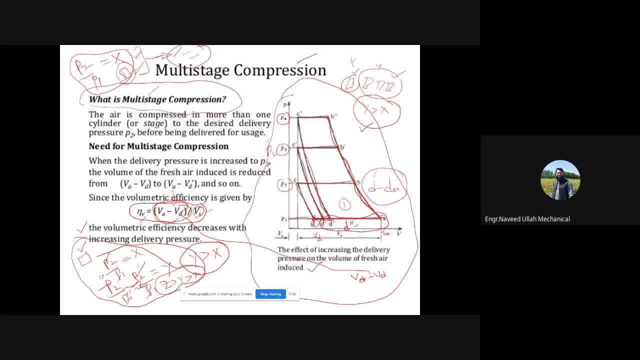 compression process this is delivery and this one is expansion okay so d and this one is expansion okay so d and this one is expansion okay so d double bar sorry d a double bar sorry d a double bar sorry d a minus d uh sorry this minus d uh sorry this minus d uh sorry this v a minus v d double bar this is now v a minus v d double bar this is now v a minus v d double bar this is now the the 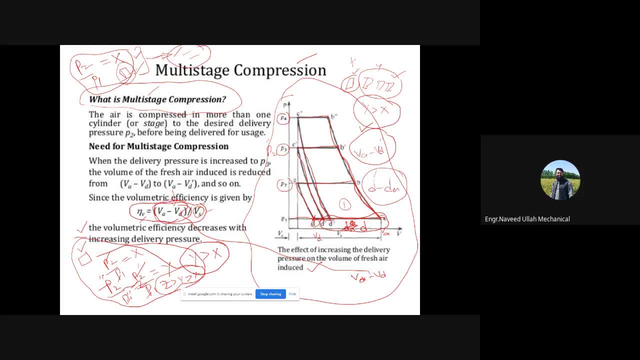 the induced volume okay so you can see that induced volume okay so you can see that 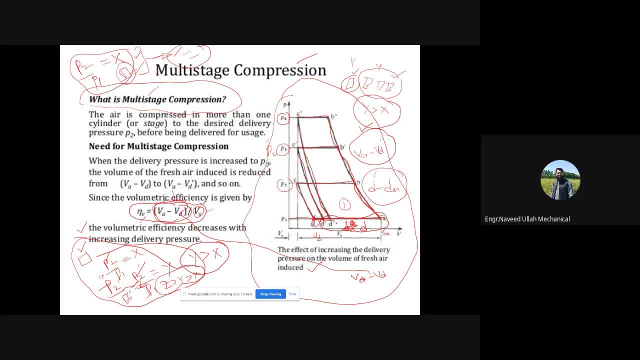 induced volume okay so you can see that increasing pressure ratio increasing pressure ratio increasing pressure ratio the induced volume is decreased the induced volume is decreased the induced volume is decreased for the same for the same for the same you know 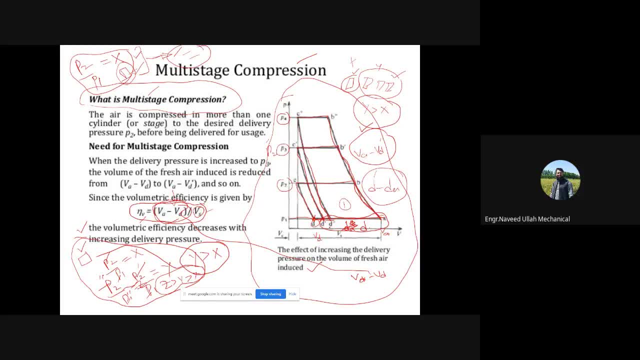 you know you know uh initial pressure uh initial pressure uh initial pressure to occupy to occupy to occupy the same the clear volume is the same the same the clear volume is the same the same the clear volume is the same and 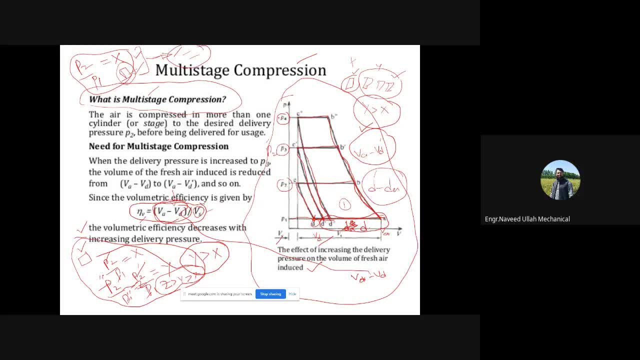 and and by increasing the pressure ratio in the by increasing the pressure ratio in the by increasing the pressure ratio in the same same same single stage a single cylinder single stage a single cylinder single stage a single cylinder reciprocating ear compressor reciprocating ear compressor reciprocating ear compressor the induced volume decreases the induced volume decreases the induced volume decreases in case of p2 by b1 it is this one in case of p2 by b1 it is this one in case of p2 by b1 it is this one in case of in case of p2 by b1 it is this one in case of p2 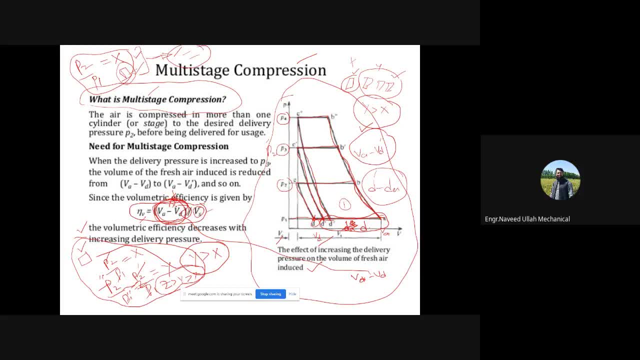 in case of p2 by b1 it is this one in case of p3 by p1 it is reduced in case of p3 by p1 it is this one in case of p3 by p1 it is reduced in case of p3 by p1 it is this one in case of p3 by p1 it is reduced in case of p4 by p1 it is reduced in case of p4 by p1 it is reduced in case of p4 by p1 it is reduced further further further it means that the numerator is 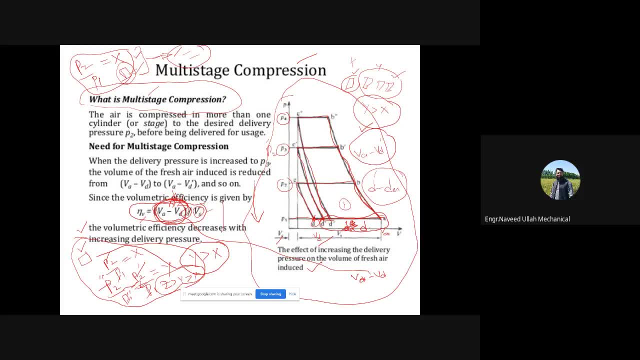 it means that the numerator is it means that the numerator is decreased by increasing the pressure decreased by increasing the pressure decreased by increasing the pressure ratio so ratio so ratio so you will have volumetric efficiency you will have volumetric efficiency you will have volumetric efficiency which is one of the parameter which is one of the parameter which is one of the parameter it will decrease and we don't want this it will decrease and we don't want this 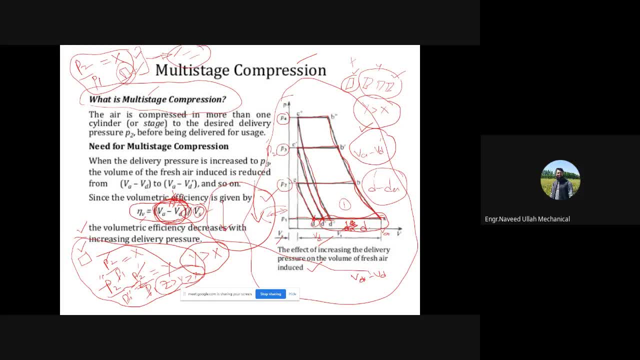 it will decrease and we don't want this because because because cylinder or single stage cylinder or single stage cylinder or single stage compression ratio compression ratio 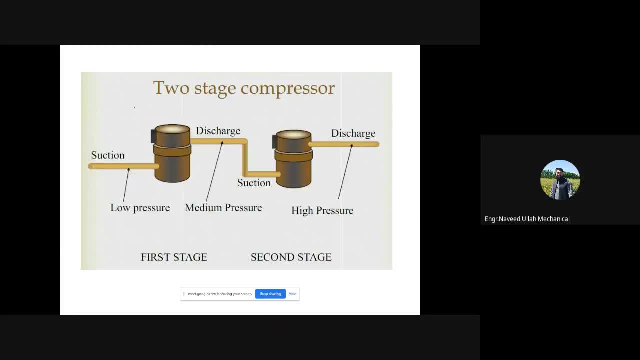 compression ratio one one one second thing is if you remember previously second thing is if you remember previously 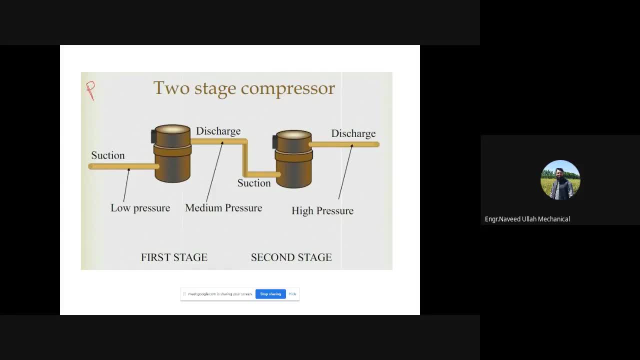 second thing is if you remember previously now i told you in this class if you use now i told you in this class if you use 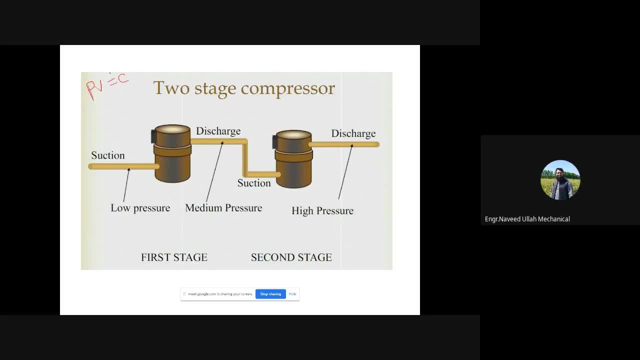 now i told you in this class if you use pv is equal to constant pv is equal to constant pv is equal to constant that is what that is if you want to that is what that is if you want to that is what that is if you want to ensure or if you can ensure ensure or if you can ensure ensure or if you can ensure that the process of compression is that the process of compression is that the process of compression is isothermal isothermal isothermal so you can say that you can consume or the so you can say that you can consume or the so you can say that you can consume or the you know the the compressor will consume you know the the compressor will consume you know the the compressor will consume less work 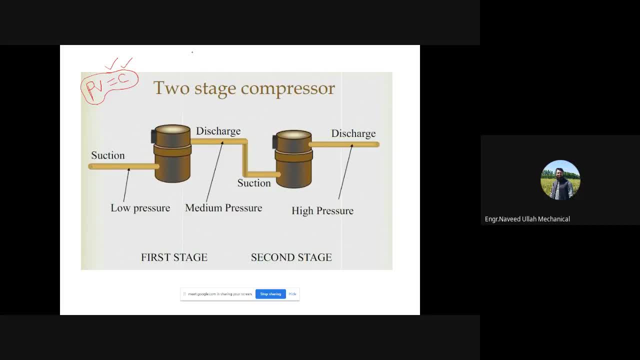 less work less work now how to achieve this now how to achieve this now how to achieve this very simply cooling very simply cooling very simply cooling because because because okay this is this was actually the okay this is this was actually the okay this is this was actually the th diagram that we saw earlier th diagram that we saw earlier 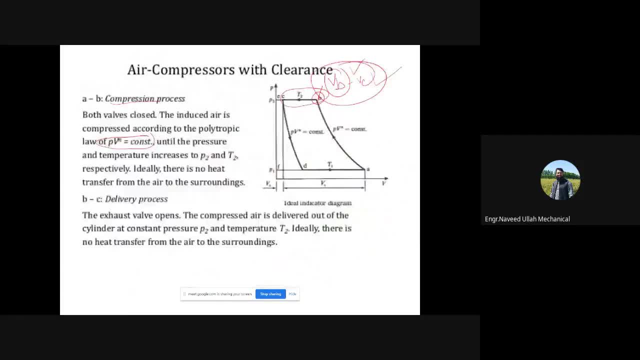 th diagram that we saw earlier that you see um that you see um that you see um what is that what is that what is that somewhere somewhere somewhere here here 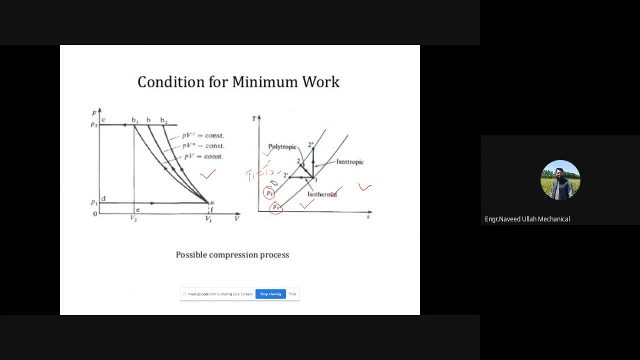 here okay okay okay by this this is your by this this is your by this this is your t1 t1 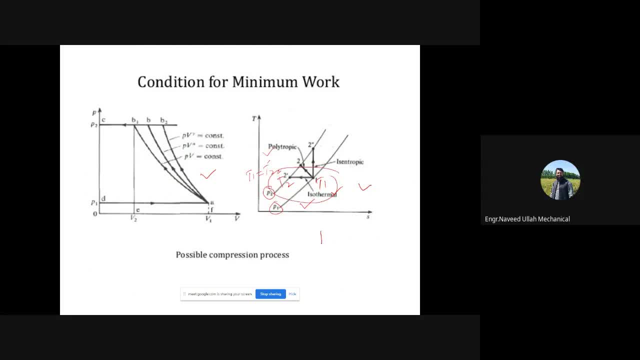 t1 and this is your and this is your and this is your t2 bar and you see that t1 is equal to t2 t2 bar and you see that t1 is equal to t2 t2 bar and you see that t1 is equal to t2 bar this means that 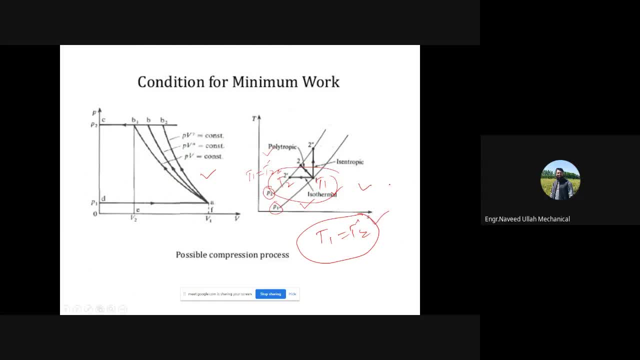 bar this means that bar this means that all the way you are basically cooling all the way you are basically cooling all the way you are basically cooling this year this year this year pressure you can cool this pressure you can cool this pressure you can cool this temperature and you can then cool temperature and you can then cool temperature and you can then cool this this this to uh the initial temperature to uh the initial temperature to uh the initial temperature constant cooling process constant cooling process 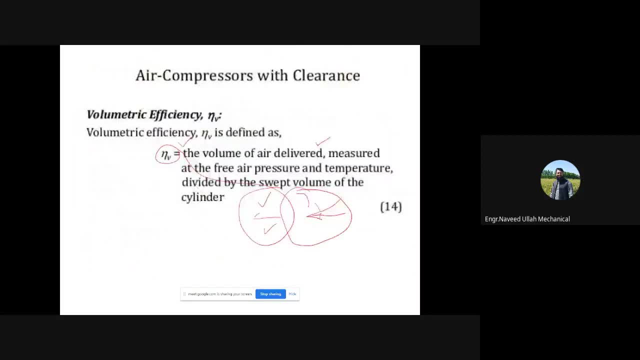 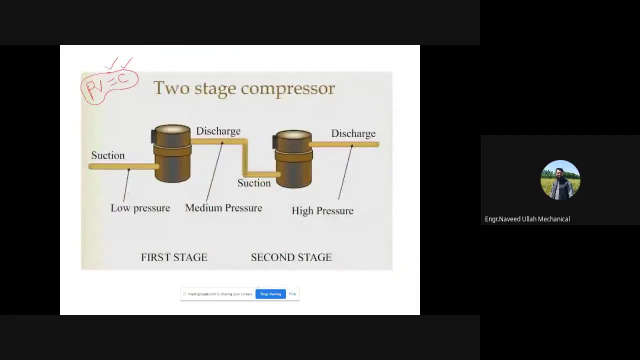 constant cooling process single stage single stage single stage you cannot efficiently achieve you cannot efficiently achieve you cannot efficiently achieve the cooling process uh in a single the cooling process uh in a single the cooling process uh in a single cylinder or in the single stage cylinder or in the single stage cylinder or in the single stage complete intercooling complete intercooling complete intercooling so for that reason so for that reason so for that reason to make the process nearly isothermal to make the process nearly isothermal to make the process nearly isothermal so for that reason uh you know you use 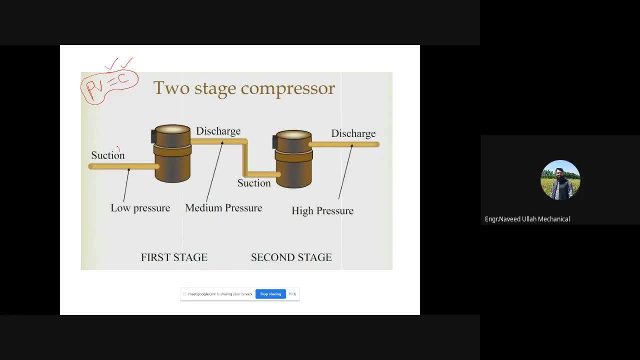 so for that reason uh you know you use so for that reason uh you know you use the two stage or three stage compression the two stage or three stage compression the two stage or three stage compression process so this will be your suction process so this will be your suction process so this will be your suction this is very schematic okay suction at this is very schematic okay suction at this is very schematic okay suction at low pressure and this is the compressor low pressure and this is the compressor low pressure and this is the compressor then it will then it will then it will have a discharge at medium pressure and have a discharge at medium pressure and have a discharge at medium pressure and then this discharge will be suction for then this discharge will be suction for 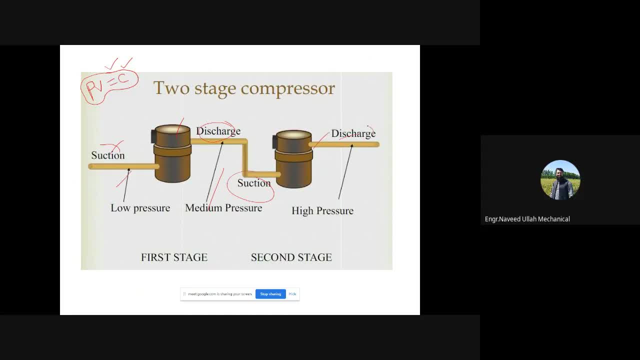 then this discharge will be suction for this one and you know this will be the this one and you know this will be the this one and you know this will be the discharge from the second one and that discharge from the second one and that discharge from the second one and that the pressure p3 let's say for example the pressure p3 let's say for example the pressure p3 let's say for example to this p1 that will be your pressure to this p1 that will be your pressure to this p1 that will be your pressure ratio okay so you can see that in ratio okay so you can see that in ratio okay so you can see that in between these two you can dedicatedly between these two you can dedicatedly between these two you can dedicatedly use use use the heat exchanger over here okay the heat exchanger over here okay the heat exchanger over here okay you can achieve this you know as a thermal you can achieve this you know as a thermal you can achieve this you know as a thermal process process process right we have a uh we have right we have a uh we have right we have a uh we have discussed discussed discussed this situation multi-stage compression this situation multi-stage compression this situation multi-stage compression right right right this situation can be improved by this situation can be improved by performing multi-stage compression 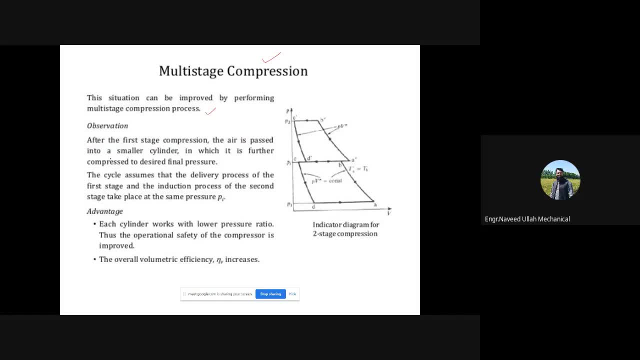 performing multi-stage compression performing multi-stage compression observation observation observation after the first stage compression the after the first stage compression the after the first stage compression the ear is passed into a smaller cylinder ear is passed into a smaller cylinder ear is passed into a smaller cylinder in which it is further compressed to uh in which it is further compressed to uh in which it is further compressed to uh desired final pressure the cycle assumes desired final pressure the cycle assumes desired final pressure the cycle assumes that the delivery process of the first that the delivery process of the first that the delivery process of the first stage and the induction process of the 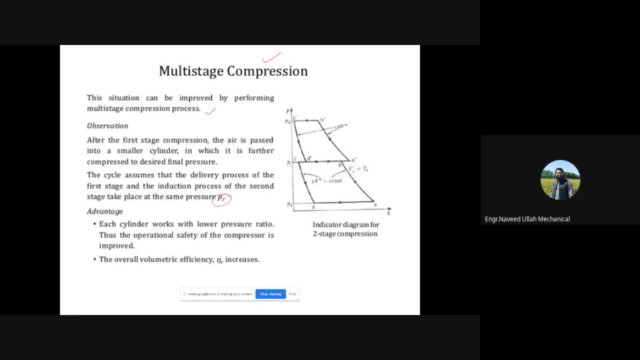 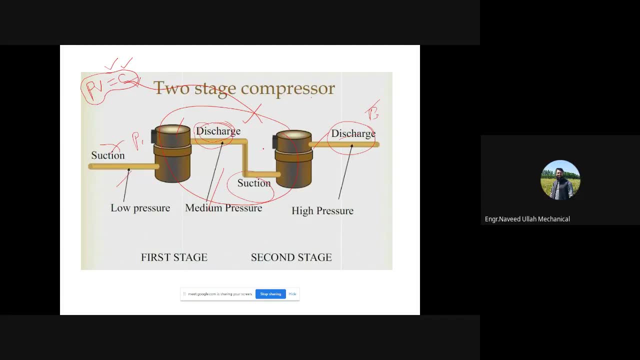 stage and the induction process of the stage and the induction process of the second stage take place at the same second stage take place at the same second stage take place at the same pressure pressure pressure pressure discharge of the first discharge of the first discharge of the first and induction suction of the second they and induction suction of the second they and induction suction of the second they are actually at the same pressure is are actually at the same pressure is are actually at the same pressure is called pi intermediate this is your p1 called pi intermediate this is your p1 called pi intermediate this is your p1 this is your p2 this is your pi this is your p2 this is your pi this is your p2 this is your pi they can obviously there will be a 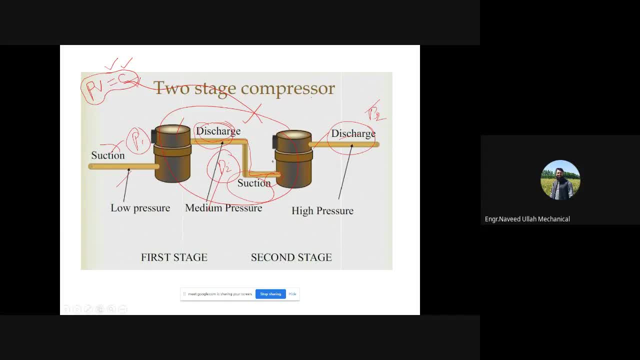 they can obviously there will be a they can obviously there will be a pressure loss inside this uh you know pressure loss inside this uh you know pressure loss inside this uh you know ducts like it ducts like it ducts like it opposed to the pressure increment at opposed to the pressure increment at opposed to the pressure increment at the pressure increase in these cylinders 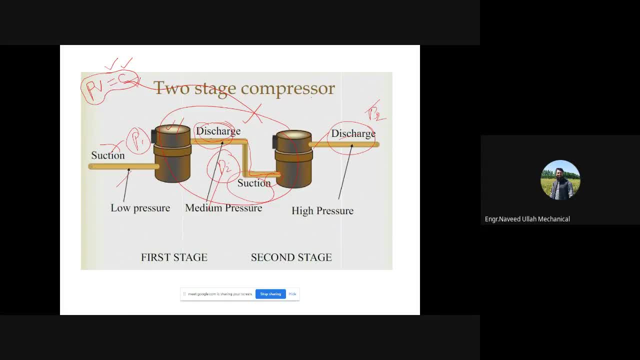 the pressure increase in these cylinders the pressure increase in these cylinders okay are in these sorry compressors okay are in these sorry compressors okay are in these sorry compressors pressure drop pressure drop 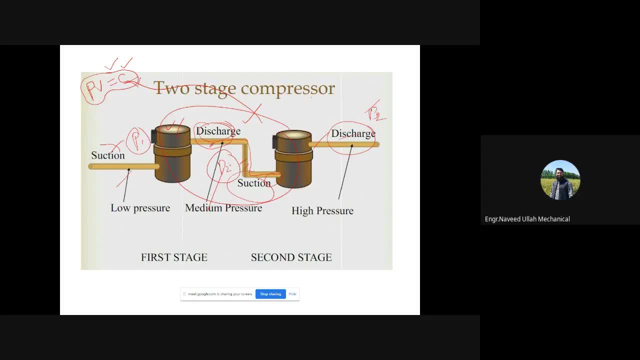 pressure drop this one inside this duct this duct it is this one inside this duct this duct it is this one inside this duct this duct it is very small so for that reason although very small so for that reason although very small so for that reason although here the pi will not happen here here the pi will not happen here here the pi will not happen here this way it will be different but they this way it will be different but they this way it will be different but they are considering that they are this is are considering that they are this is are considering that they are this is the same this is talking about this pi the same this is talking about this pi 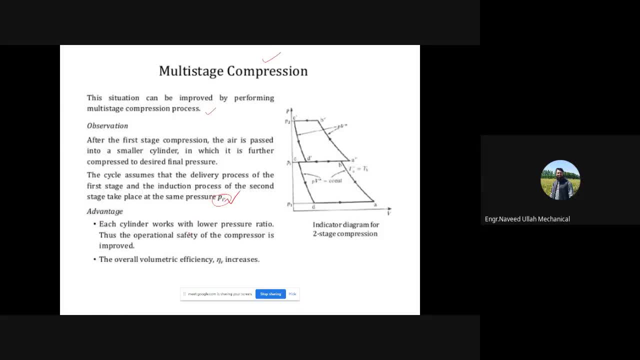 the same this is talking about this pi okay okay okay so what is the advantage of each cylinder 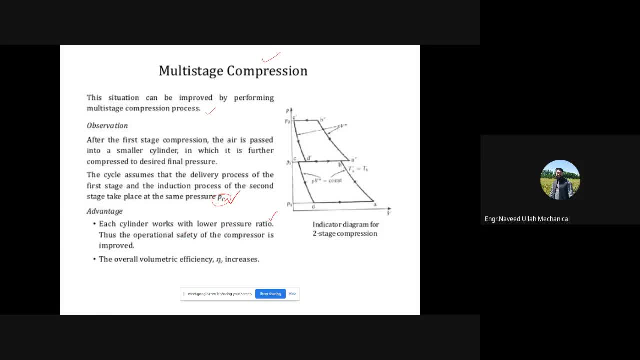 so what is the advantage of each cylinder so what is the advantage of each cylinder works with lower pressure ratio works with lower pressure ratio works with lower pressure ratio one of the first advantages is that if one of the first advantages is that if one of the first advantages is that if a double cylinder 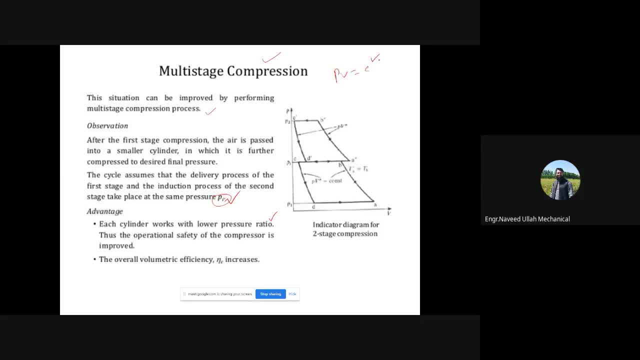 a double cylinder a double cylinder two things we discussed one to achieve two things we discussed one to achieve two things we discussed one to achieve pvc equal to constant pvc equal to constant pvc equal to constant second thing is that volumetric second thing is that volumetric second thing is that volumetric efficiency decreases which is not good efficiency decreases which is not good 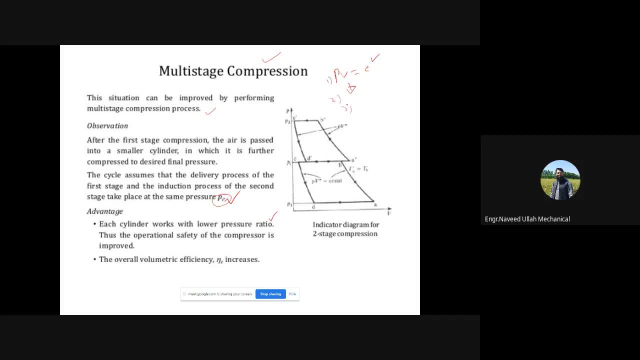 efficiency decreases which is not good okay well third thing is that okay well third thing is that 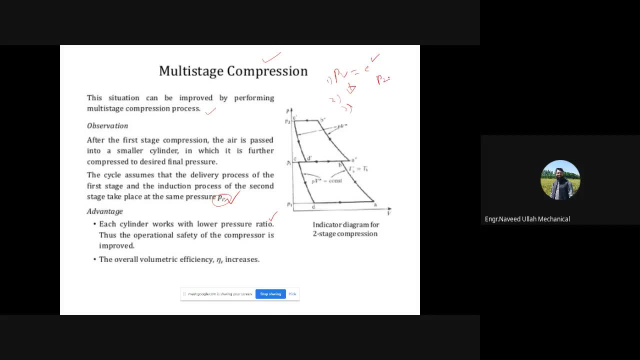 okay well third thing is that let's say for example your pressure ratio let's say for example your pressure ratio let's say for example your pressure ratio is a p is a p is a p four by p p four by p p four by p p p three by p one three by p one three by p one right and this is let's say for example right and this is let's say for example right and this is let's say for example hundred by one bar hundred by one bar hundred by one bar abhiya for example now this hundred bar 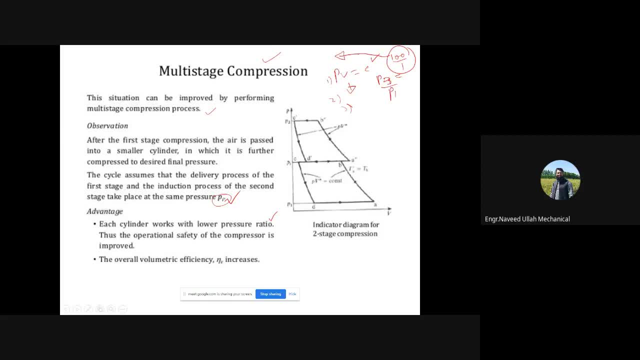 abhiya for example now this hundred bar abhiya for example now this hundred bar high pressure you are working with high pressure you are working with high pressure you are working with are the system is under the influence of are the system is under the influence of are the system is under the influence of high pressure ratio high pressure ratio high pressure ratio that is hazardous you know that right that is hazardous you know that right that is hazardous you know that right hazardous actually has a one and then to hazardous actually has a one and then to 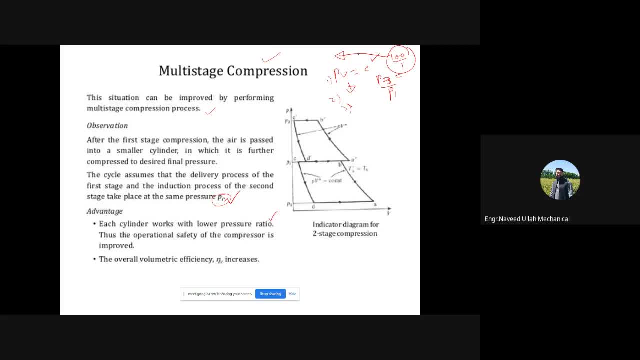 hazardous actually has a one and then to keep that uh keep that uh keep that uh pressure okay you need to have these pressure okay you need to have these 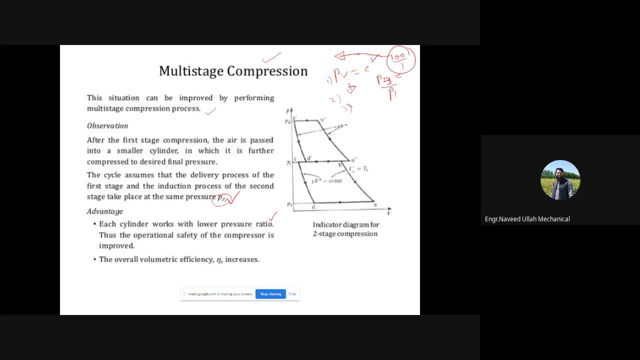 pressure okay you need to have these cylinders okay and these compressor cylinders okay and these compressor cylinders okay and these compressor made of a very sophisticated material that made of a very sophisticated material that made of a very sophisticated material that can withstand this pressure can withstand this pressure can withstand this pressure okay and this is even hazardous to the 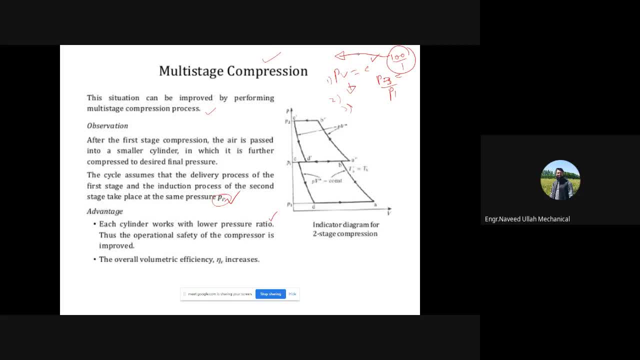 okay and this is even hazardous to the okay and this is even hazardous to the operator also operator also operator also now in if you are you know reducing now in if you are you know reducing now in if you are you know reducing and if you are using multi-stage and if you are using multi-stage and if you are using multi-stage compression top compression top compression top one two one two one two fifty bar in first stage and fifty two let's 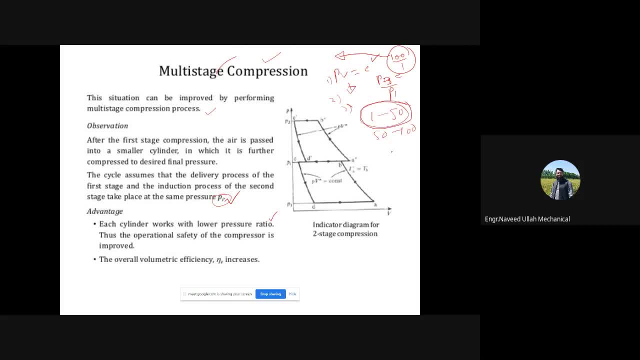 fifty bar in first stage and fifty two let's fifty bar in first stage and fifty two let's say hundred bar in second stage now what is say hundred bar in second stage now what is say hundred bar in second stage now what is the your pressure ratio inside the your pressure ratio inside the your pressure ratio inside are in a single uh you know stage that are in a single uh you know stage that are in a single uh you know stage that is your 50 by one is your 50 by one is your 50 by one okay so it is not hazardous you have okay so it is not hazardous you have 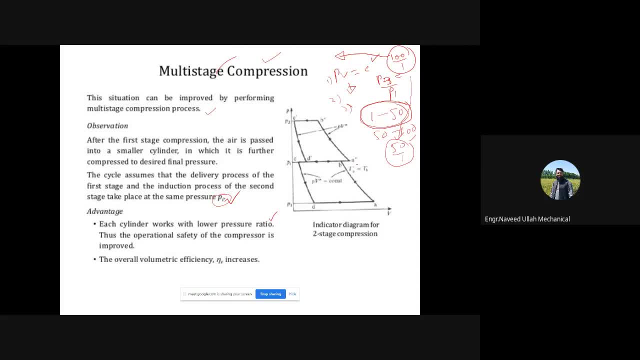 okay so it is not hazardous you have actually reduced that to half almost actually reduced that to half almost actually reduced that to half almost together it is actually not hazardous one together it is actually not hazardous one together it is actually not hazardous one and the second thing is that you can you and the second thing is that you can you and the second thing is that you can you reduce uh you know the reduce uh you know the reduce uh you know the material cost okay just say up material cost okay just say up material cost okay just say up they are saying that you see uh here they are saying that you see uh here they are saying that you see uh here uh d to a is a uh d to a is a uh d to a is a two-stage measure d to a is uh induction 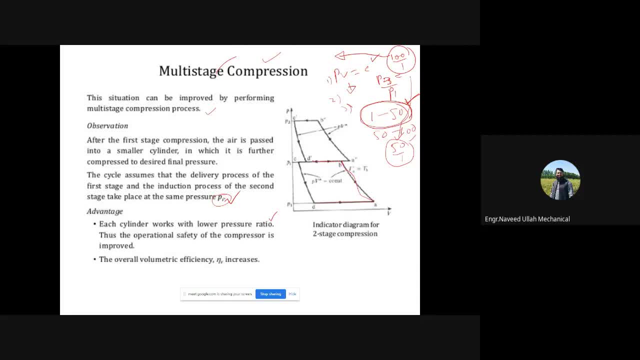 two-stage measure d to a is uh induction two-stage measure d to a is uh induction then b a compression process then then b a compression process then then b a compression process then c two uh sorry b to c is delivery but c two uh sorry b to c is delivery but c two uh sorry b to c is delivery but that delivery is basically that delivery is basically that delivery is basically you know this uh uh you know this uh uh you know this uh uh induction to the second okay so a double induction to the second okay so a double induction to the second okay so a double prime b double prime we have b prime c prime b double prime we have b prime c prime b double prime we have b prime c prime and this one okay so you can see prime and this one okay so you can see 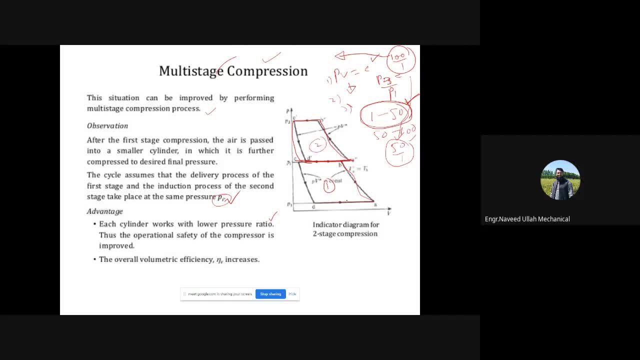 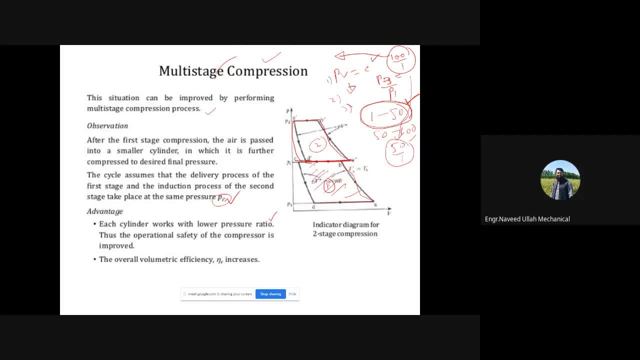 achieve the isothermal process the work consumed by this and this plus this will consumed by this and this plus this will consumed by this and this plus this will be less than the first one 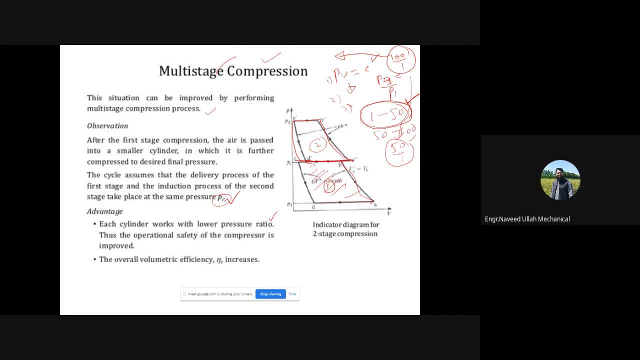 the system is not hazardous one second the system is not hazardous one second the system is not hazardous one second thing is that you are not losing the thing is that you are not losing the 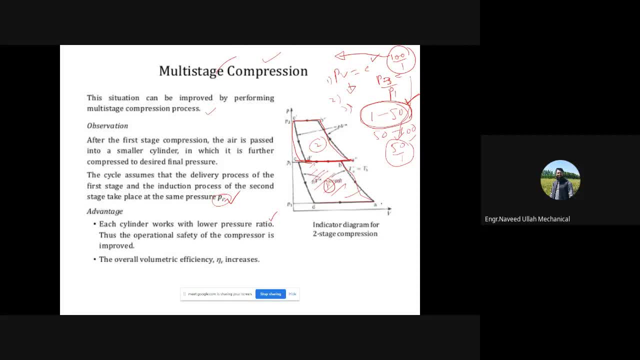 thing is that you are not losing the volumetric efficiency okay too much volumetric efficiency okay too much volumetric efficiency okay too much because you are having the same 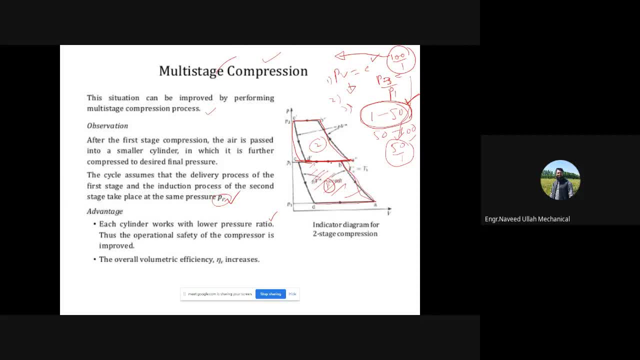 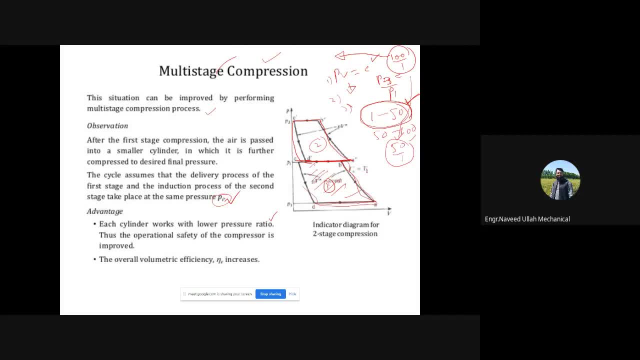 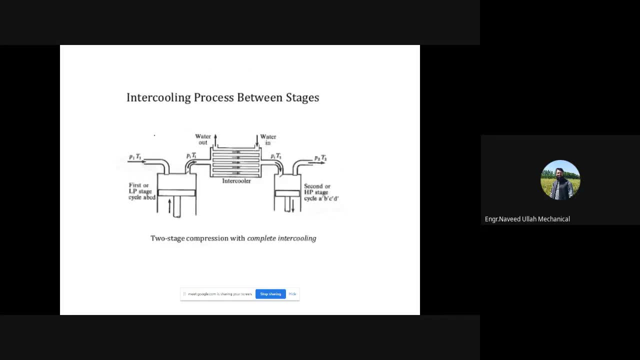 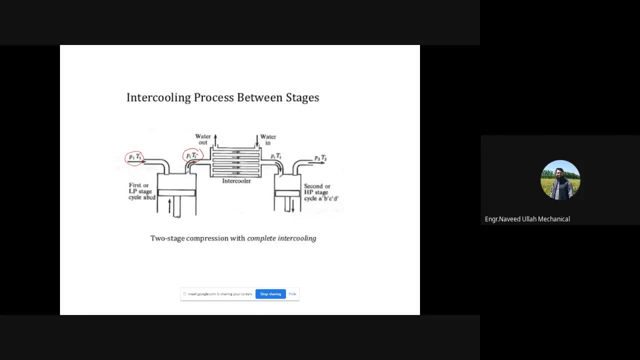 this is p i t i okay and iti it should be ti i think okay and iti it should be ti i think okay and iti it should be ti i think this is a intermediate pressure this is a intermediate pressure 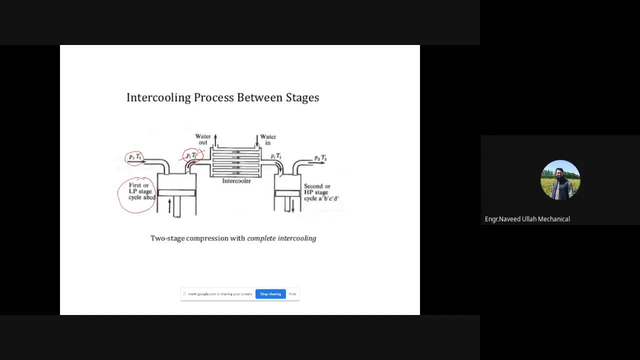 this is a intermediate pressure intermediate temperature after fun's intermediate temperature after fun's intermediate temperature after fun's first stage of low pressure compressor first stage of low pressure compressor 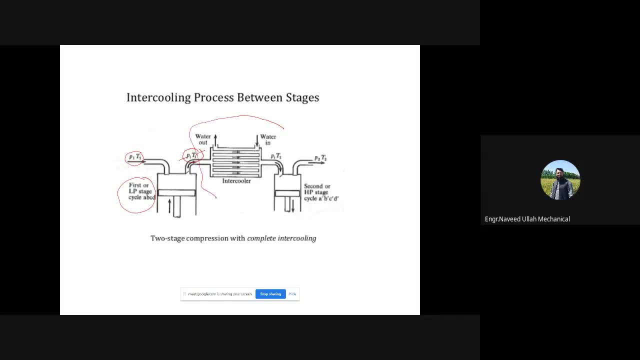 first stage of low pressure compressor and then you know there is a dedicated and then you know there is a dedicated and then you know there is a dedicated heat exchanger or intercooler installed heat exchanger or intercooler installed heat exchanger or intercooler installed here 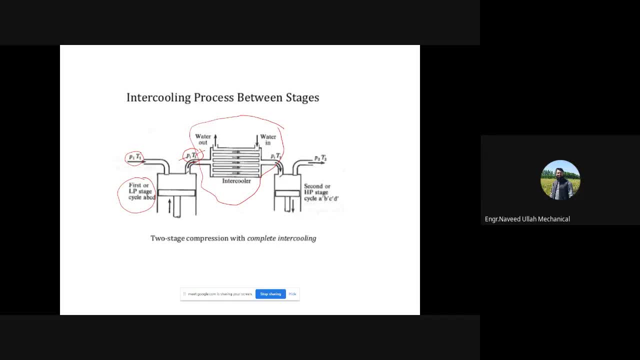 here here here here okay 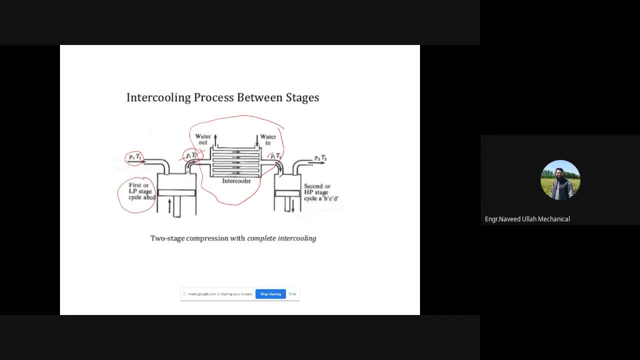 okay okay so this intercooling process makes this so this intercooling process makes this so this intercooling process makes this they are saying that this is ideally you they are saying that this is ideally you they are saying that this is ideally you know this is supposed to be p i know this is supposed to be p i know this is supposed to be p i but this t i but this t i but this t i is reduced to what to t1 is reduced to what to t1 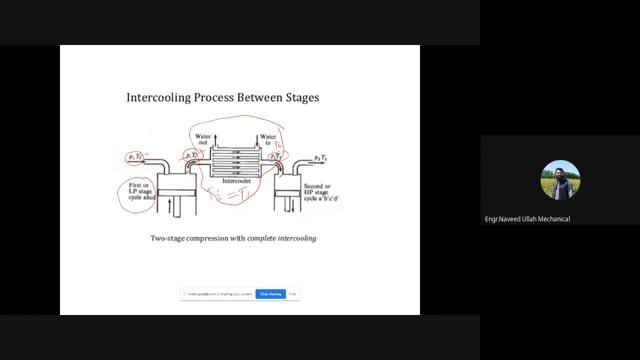 is reduced to what to t1 okay the pressure was increased from okay the pressure was increased from okay the pressure was increased from t1 to t i t1 to t i t1 to t i but using this intercooler it is again but using this intercooler it is again but using this intercooler it is again converted to converted to converted to t1 ticket and you are actually t1 ticket and you are actually t1 ticket and you are actually having this having this having this so it's intercooler so it's intercooler so it's intercooler and sometimes after coolers are there 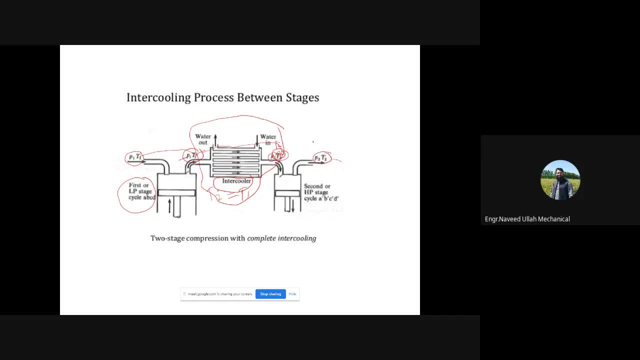 and sometimes after coolers are there and sometimes after coolers are there cng pumps cng pumps cng pumps they have actually delivering this they have actually delivering this they have actually delivering this at p2 but at t2 at p2 but at t2 at p2 but at t2 increased temperature then they are increased temperature then they are increased temperature then they are actually using this after coolers actually using this after coolers actually using this after coolers in order to have this yes p2 but this in order to have this yes p2 but this in order to have this yes p2 but this one is at t1 etc anyway 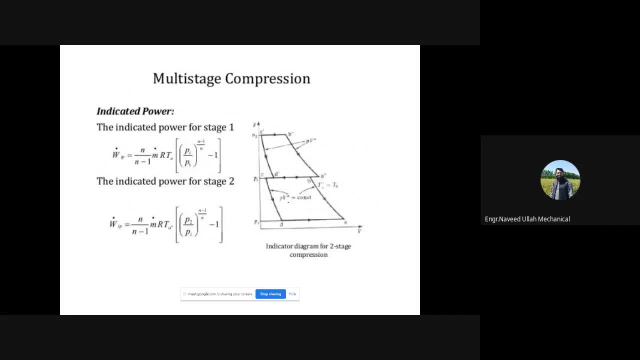 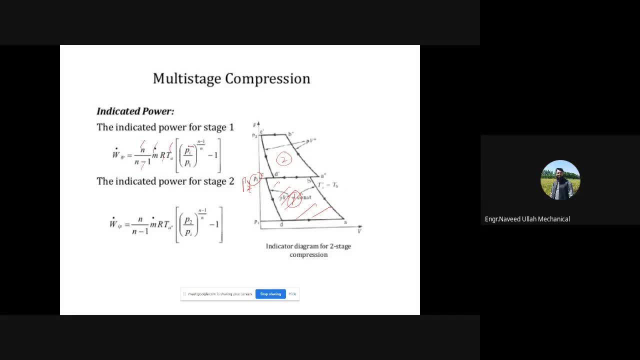 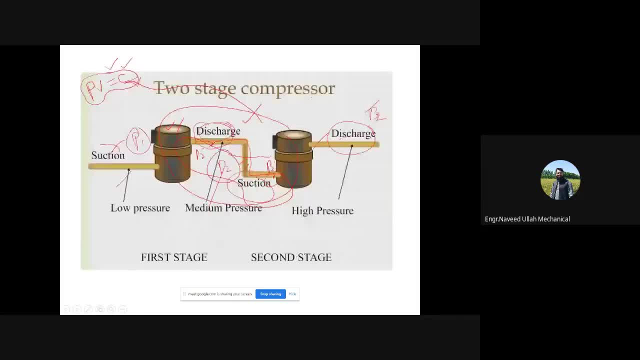 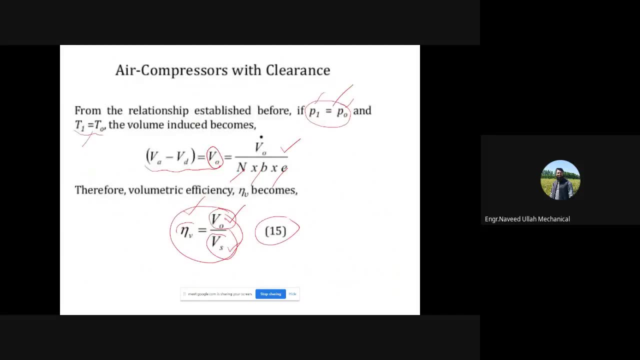 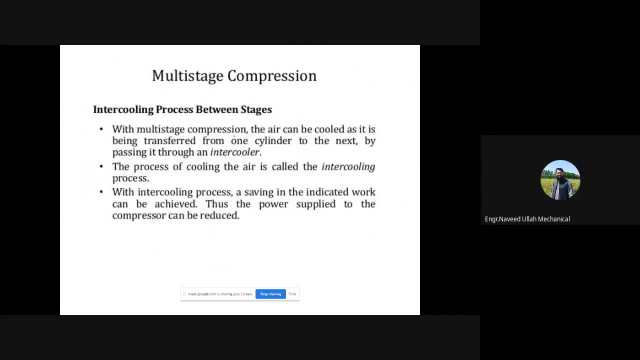 actually divided this into two stages actually divided this into two stages right right right right intercooling process between stages 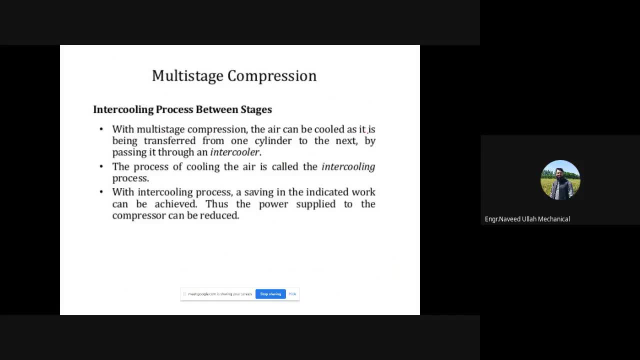 intercooling process between stages with multi-stage compression the with multi-stage compression the with multi-stage compression the air can be cooled as it is being air can be cooled as it is being air can be cooled as it is being transferred from one cylinder to the transferred from one cylinder to the transferred from one cylinder to the next by passing through intercooler next by passing through intercooler next by passing through intercooler dedicated intercooler the process of dedicated intercooler the process of dedicated intercooler the process of cooling the air is called intercooling cooling the air is called intercooling cooling the air is called intercooling process and with inter cooling process process and with intercooling process process and with intercooling process are saving an indicated work intercooling 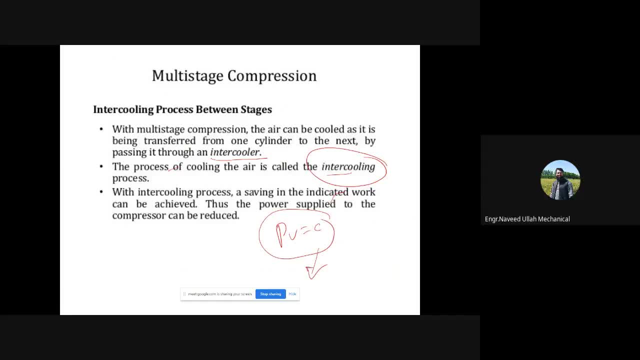 are saving an indicated work intercooling constant or a honey pie key by constant or a honey pie key by constant or a honey pie key by a girl in the pooling the process will be 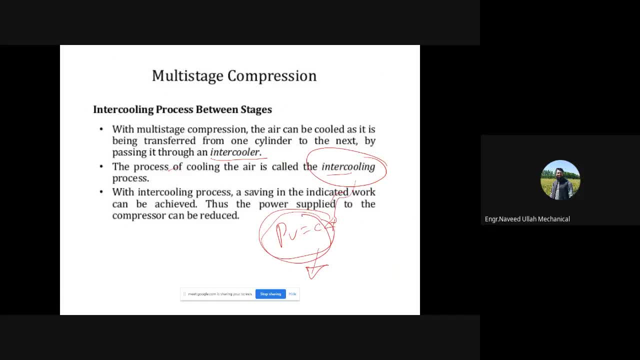 a girl in the pooling the process will be a girl in the pooling the process will be are it will tend to world this PV is are it will tend to world this PV is are it will tend to world this PV is equal to constant and if you are having equal to constant and if you are having equal to constant and if you are having this type of compression previously we 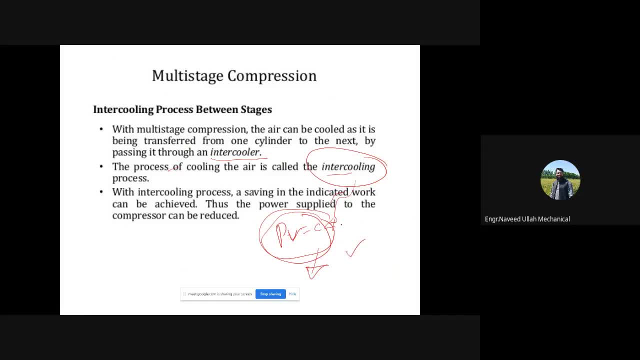 this type of compression previously we this type of compression previously we discussed that the working will be less 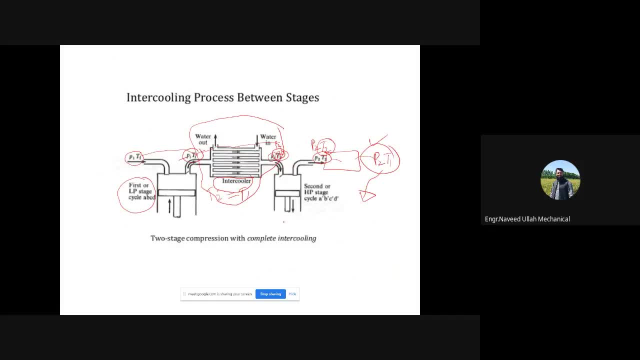 discussed that the working will be less discussed that the working will be less ticket we achieve an obvious manager ticket we achieve an obvious manager ticket we achieve an obvious manager you can see this this cylinder this 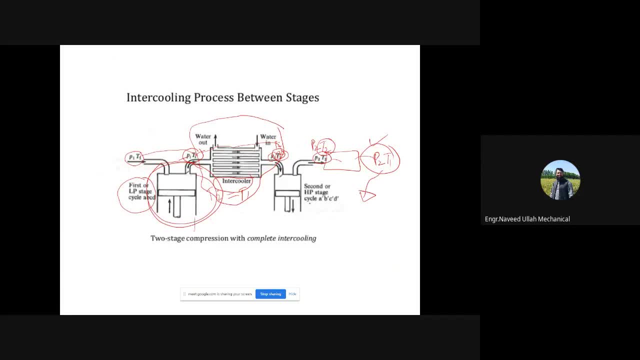 you can see this this cylinder this you can see this this cylinder this stage is a bigger in size than this one 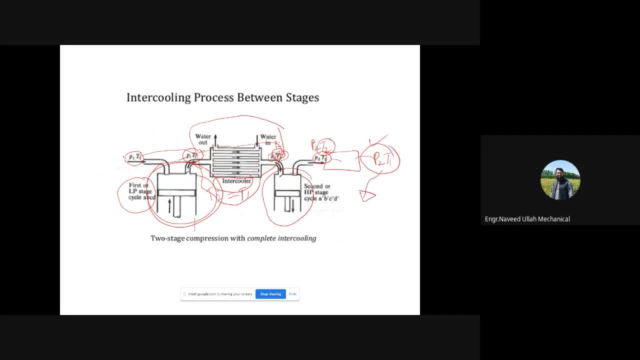 stage is a bigger in size than this one or excuse enough to put a check in case or excuse enough to put a check in case or excuse enough to put a check in case I induced my room Zara a three-year I induced my room Zara a three-year I induced my room Zara a three-year induction curtain the delivered volume 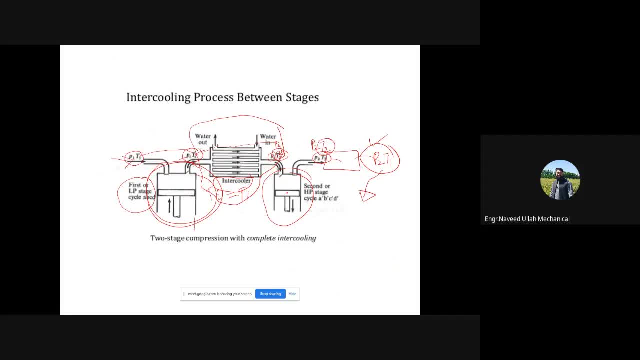 induction curtain the delivered volume induction curtain the delivered volume of this stage one is a induced volume of of this stage one is a induced volume of of this stage one is a induced volume of this stage to wages which is basically this stage to wages which is basically this stage to wages which is basically compressed the compressed a compressed compressed the compressed a compressed 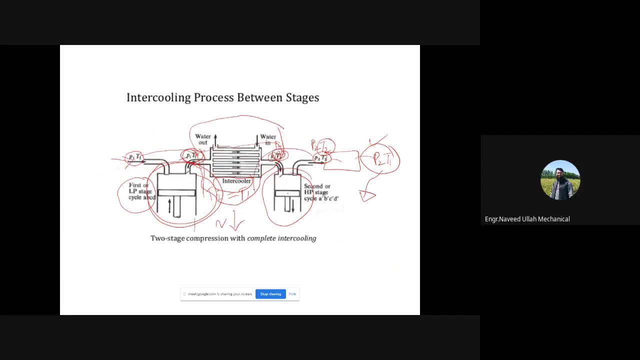 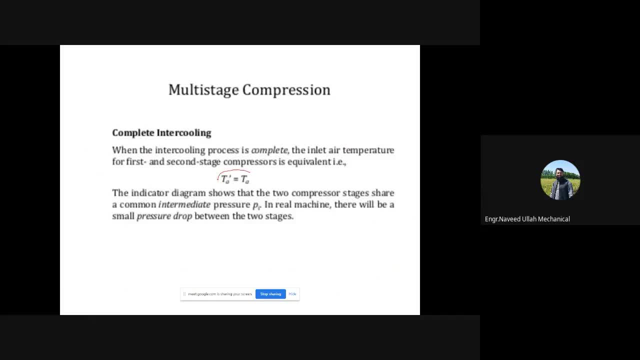 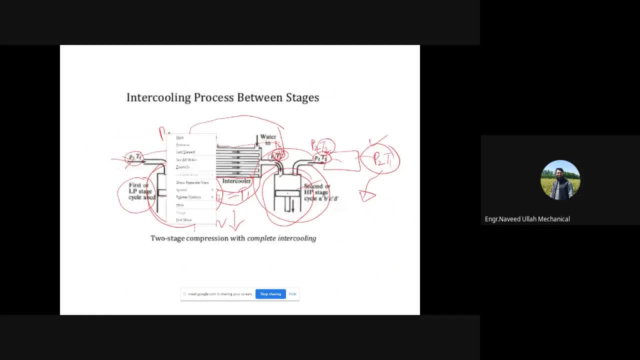 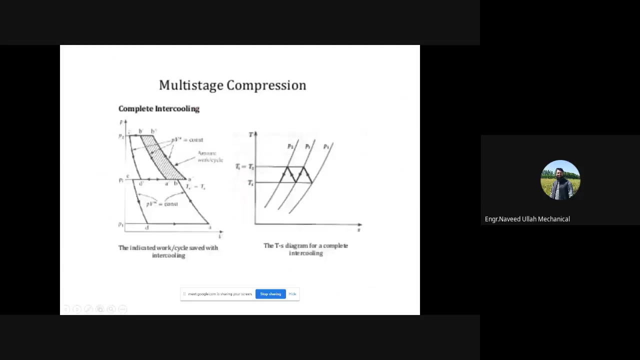 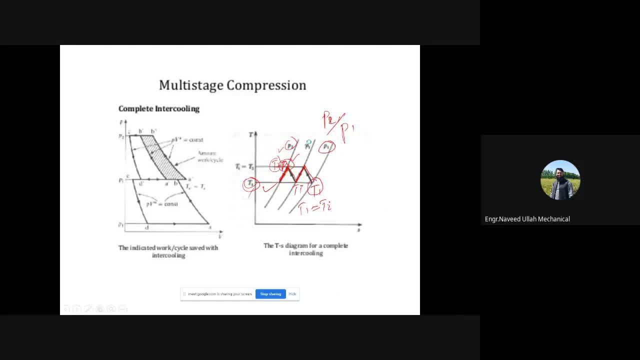 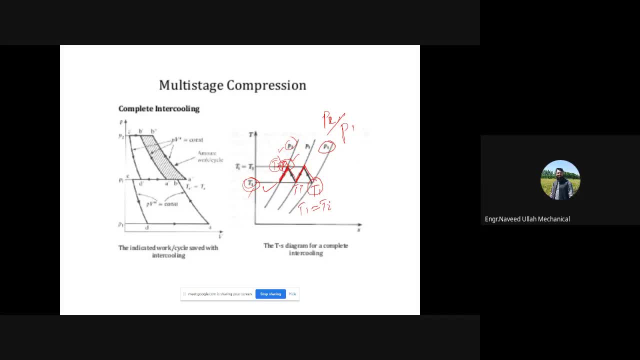 announcement remember most probably working most probably Kaki I should announce that when we will complete this chapter 12 okay maybe in the next class so after that after that week okay there will be a quiz in in your relative 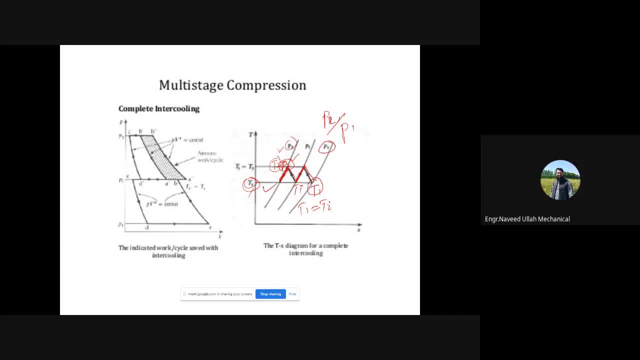 classes section C a class hoagie section your back a section okay up nick losses me they will be quiz okay quiz we had host areas yoga because I'm just feeling that that is not the proper way that we are giving a unique visit or something like this the quiz will get written in a specific way I am just feeling that that is not the proper way that we are giving a quick visit and something like this the quiz 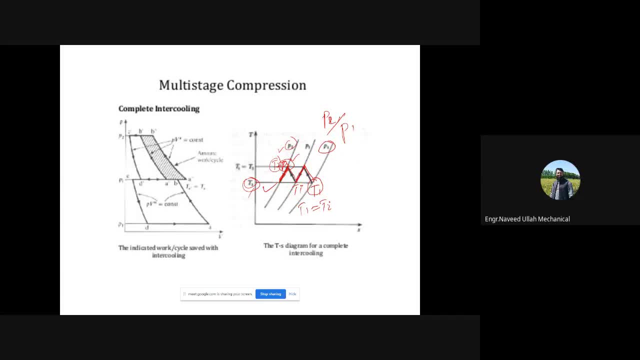 will be like this that it will be sort of viva okay the students in the class that will be you know we'll be having an interactive section session and i will ask from the student in the 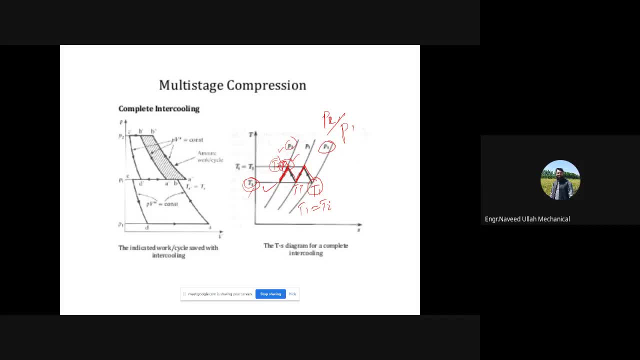 in the topic that we have studied earlier okay chapter 9 10 or 12 and they need to answer me and i will on the spot you know assign marks to that student okay so we will be having two this type these types of quizzes in this session and two assignments will be there so this is actually the sessional work and you know very well that this sessional work is actually of 30 marks okay that is even having a greater percentage 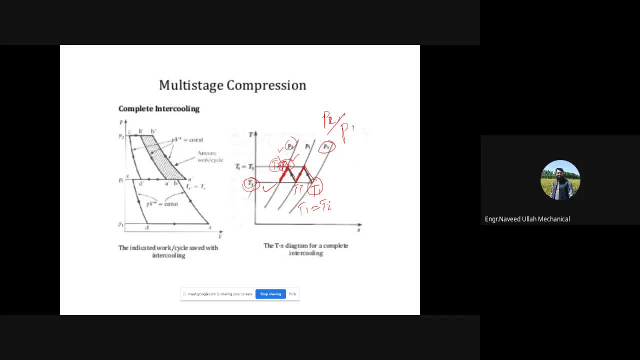 okay so i will announce on your google classroom for each and every section in their respective class there will be a quiz and that quiz will be of this type that i will ask questions from you and i will assign you marks at that particular time okay so this is 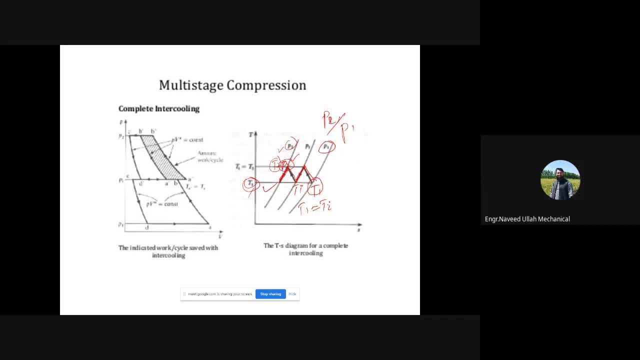 and that assignment will may be one in your chapter 11 and that assignment will be in chapter 13 right so this thing will be in your mind okay um you can 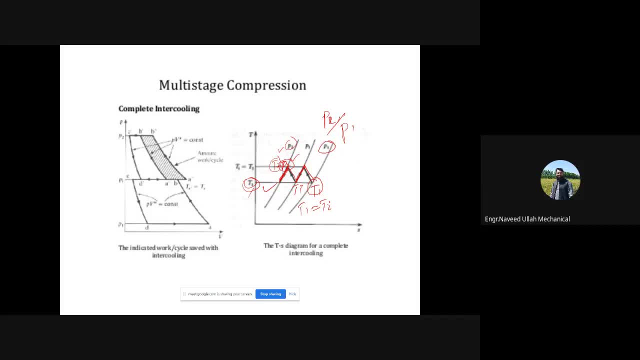 listen to this lecture and i also uploaded the slides on your google classroom and if you feel any problem then you can contact me right so i said that your time may not be available 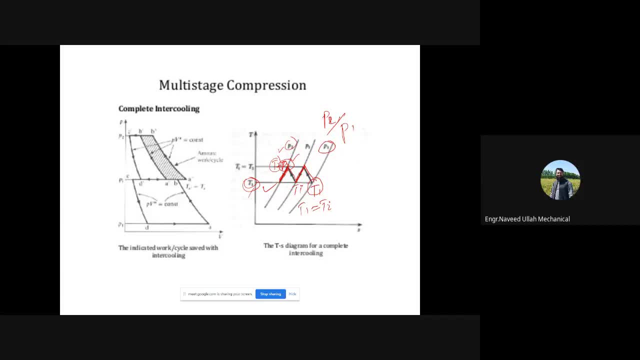 although there are no classes were there but actually i found some time so i have